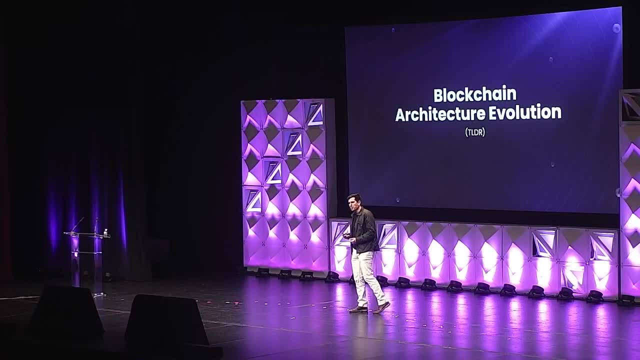 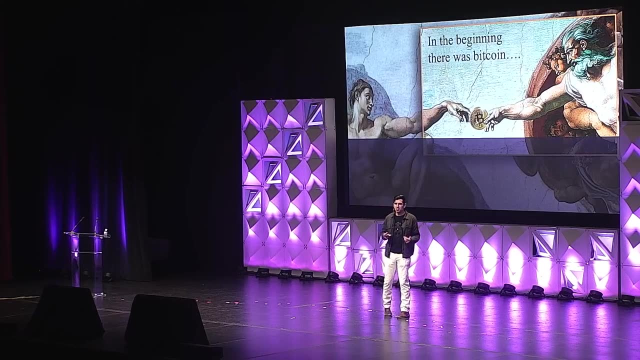 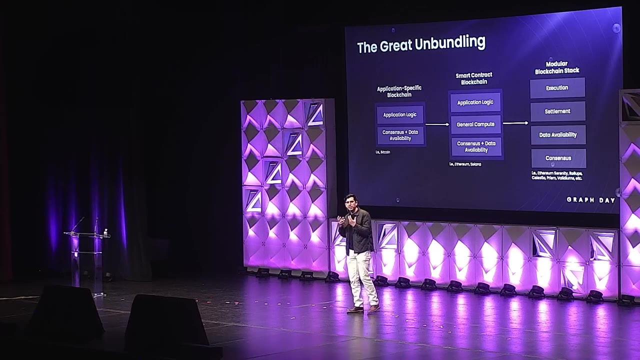 So here's the mandatory Bitcoin slide. In the beginning there was Bitcoin. It was good, But the problem was it only really did one thing right: It was the money app, And it was all kind of rolled into the other innovations of blockchain around consensus and having. 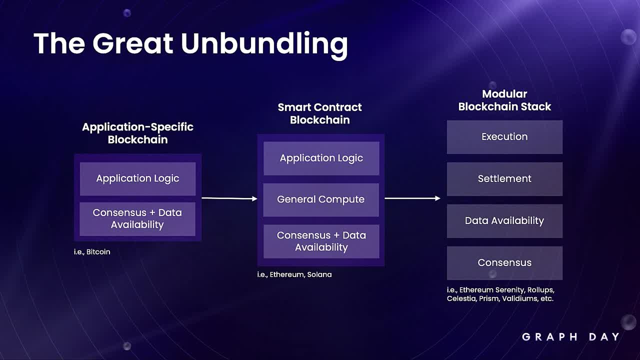 this distributed data availability and state machine. A few years later, projects like Ethereum came along and said: hey, what if we decouple the, The general compute layer, and allow people to build their own purpose-built, application-specific smart contracts? But it was all still bundled in the same package, right? So consensus. 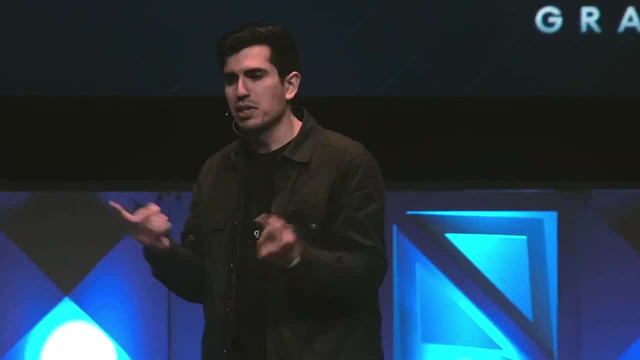 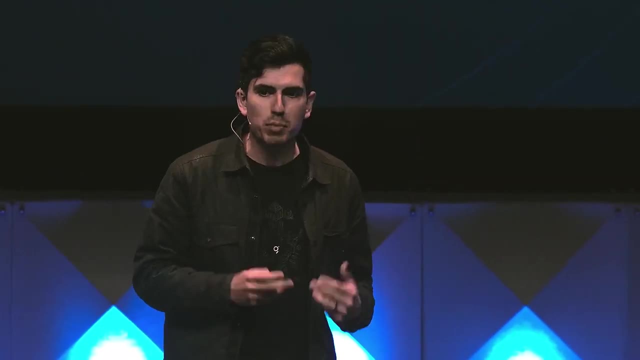 data availability, smart contract execution- it was all happening within the same chain. Now, in the last few years, with the advent of technologies such as roll-ups, as well as purpose-built chains such as Celestia or Arweave, we're seeing this great unbundling. 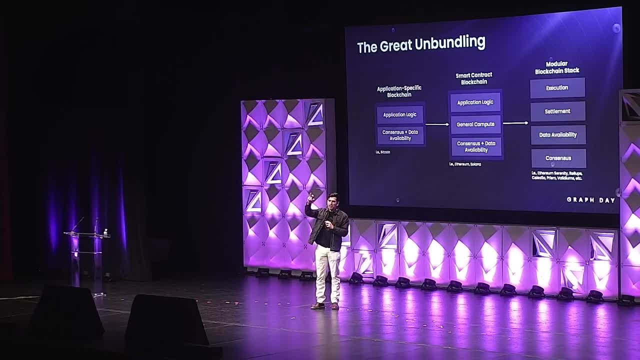 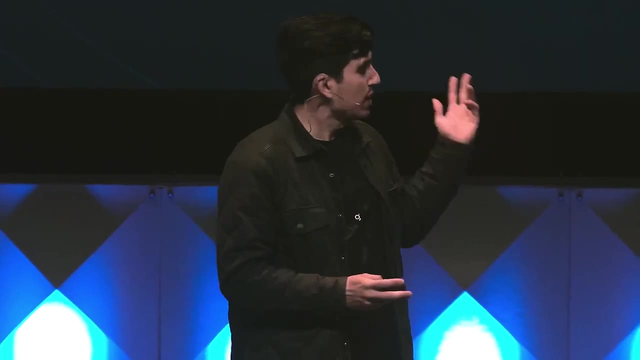 happen where These layers are starting to separate and you're starting to see purpose-built layers in the stack that can each be optimized for their own purpose and scaled out independently, And this permits a whole new universe of design patterns represented by the columns that you 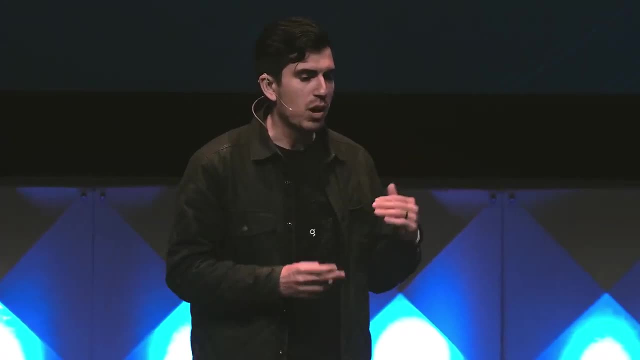 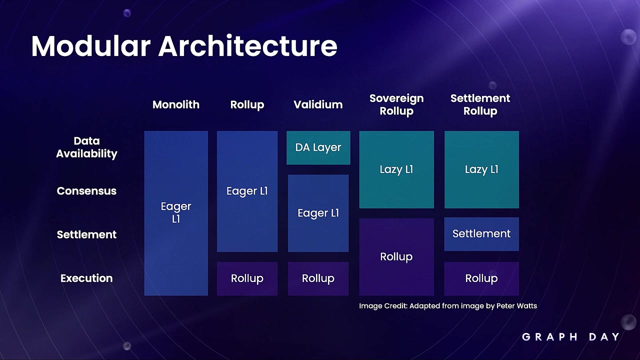 see behind me where the rows are, the different layers in the modular blockchain stack that have been unbundled, And you can see that we can still do the classic monolithic architectures, we can do roll-ups, we can do validiums and so on. 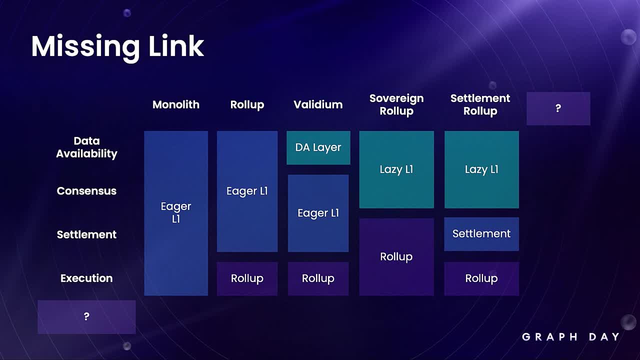 And what I would like to pose to you is that there's actually a missing layer in the modular blockchain stack that's been underappreciated and under-considered in the blockchain space up until this point, And to understand why I believe that's the case, I want to walk you through a few missing 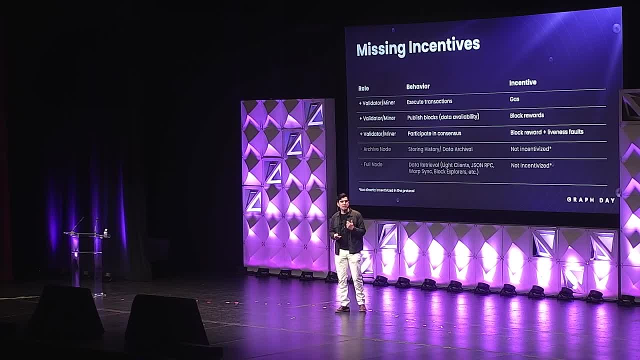 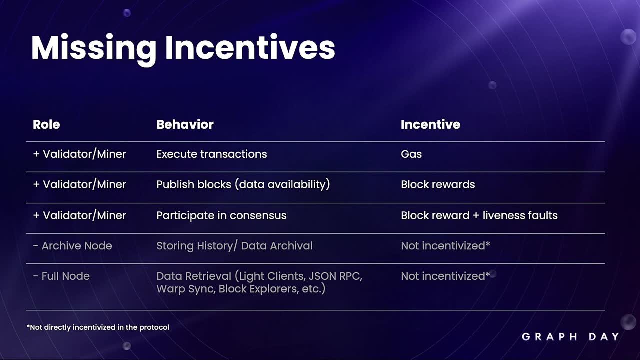 pieces that exist in blockchains today. The first is on the incentive layer, So we tend to think a lot about the incentives that exist in blockchain, such as the gas price auction, the block rewards, Um, Um. there's also things that blockchains need to do to succeed that aren't directly incentivized. 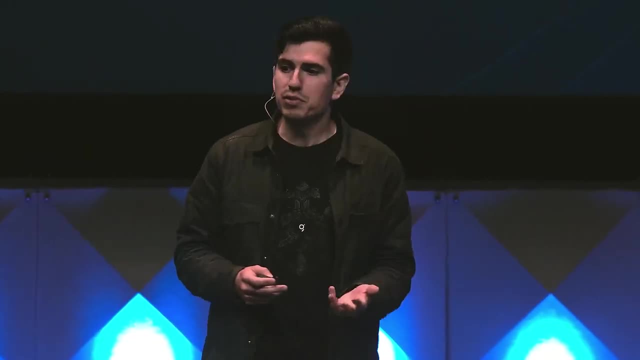 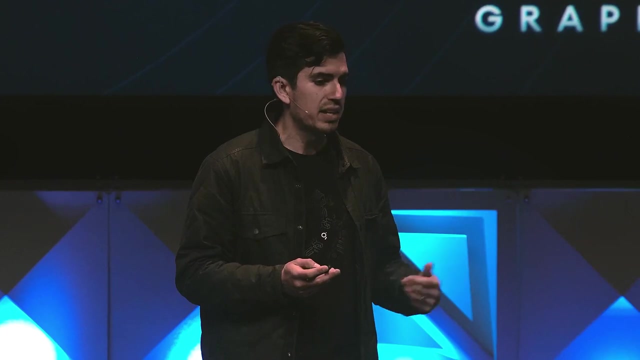 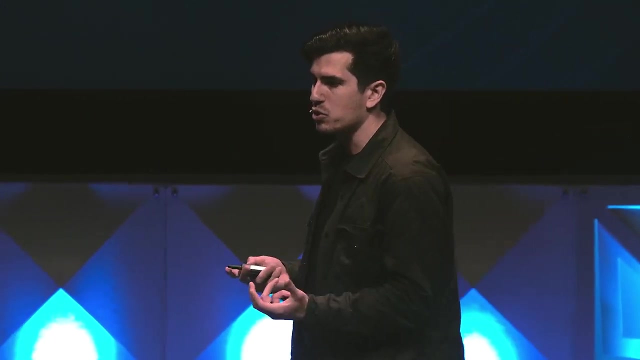 such as storing historical state, running archive nodes, doing data retrieval right. A big part of the Ethereum and blockchain vision was being able to do light clients and warp sync. have you know, decentralized block explorers? All of that stuff is not incentivized directly in the blockchain. 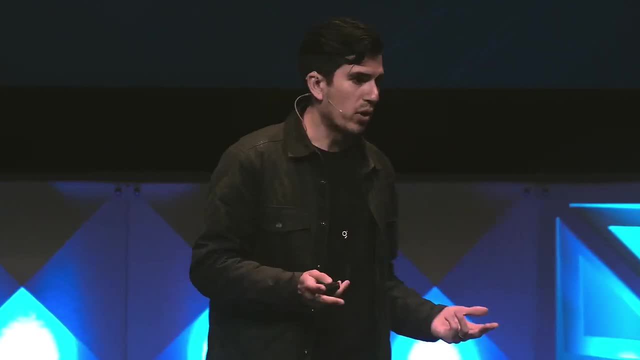 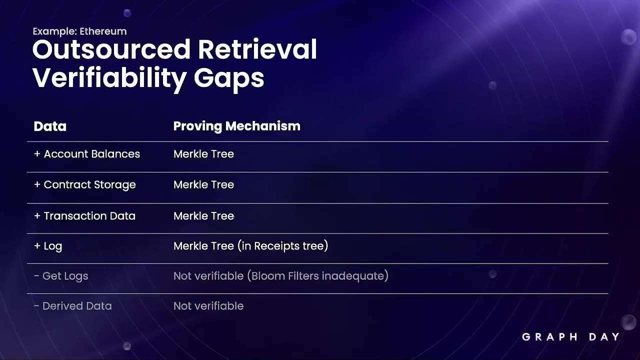 protocols that we have today. Furthermore, it's not possible to verifiably get all types of data off of the blockchains that we have today. If you're interested in account balances or you know transaction lists, great. But if you're interested in derived data or more complex, 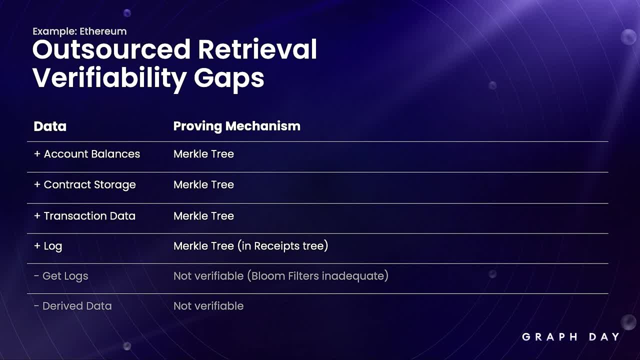 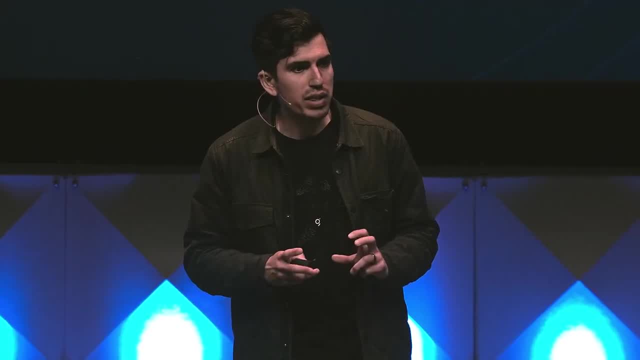 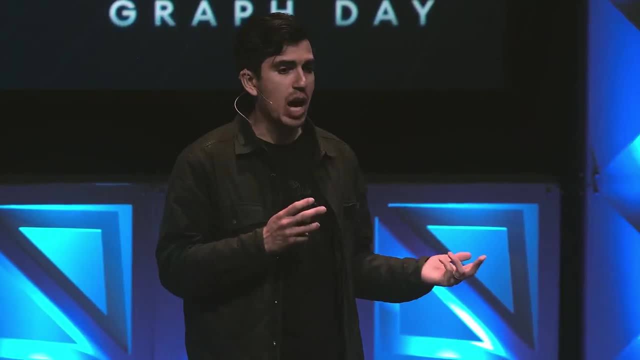 you know filtered queries like ethget logs. there's actually not a verifiable way to outsource these types of queries to a full node. Now, one way that you could approach solving this problem is to spin up a bunch of centralized blockchain APIs on top of the full nodes in this blockchain data supply chain, And indeed, 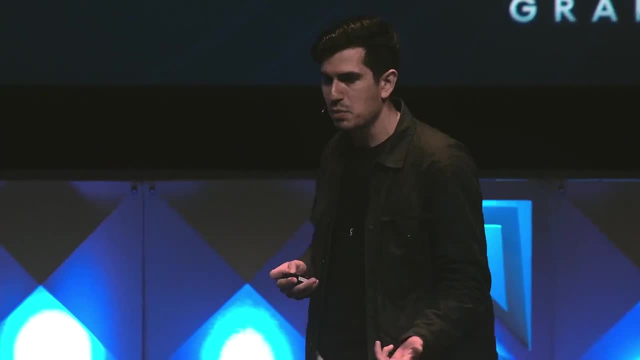 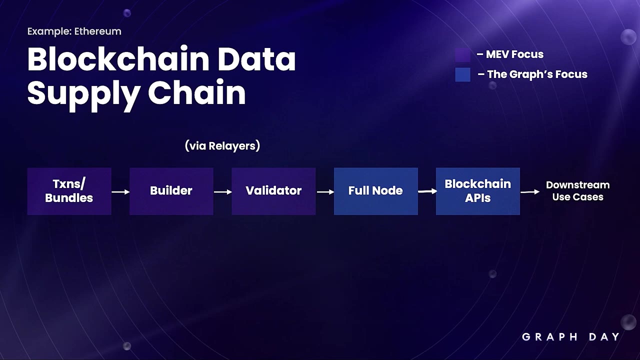 that's what's happened. We see things like Infura, Alchemy, the OpenCNFT API be very successful, But we believe in a similar spirit to the MEV researchers that are looking at the transaction supply chain and observing that centralization at one layer in that chain can infect the other. 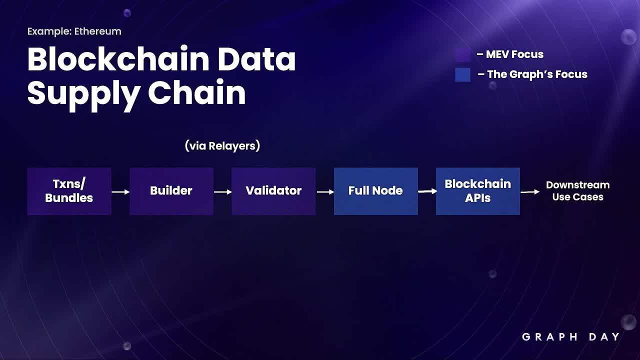 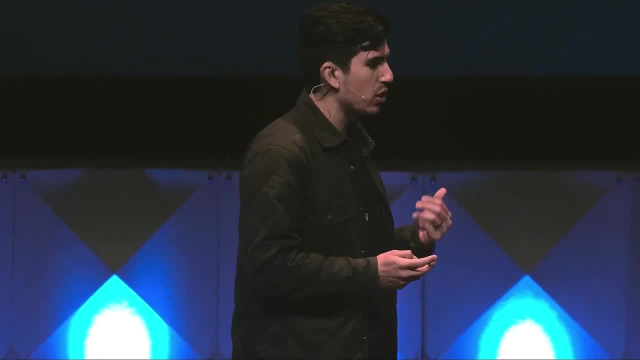 layers. We believe that it's necessary for the end-to-end blockchain data supply chain to be decentralized. Otherwise, the only ones with the incentive to run these full nodes, these archive nodes, are going to be centralized companies and will all be disintermediated from. 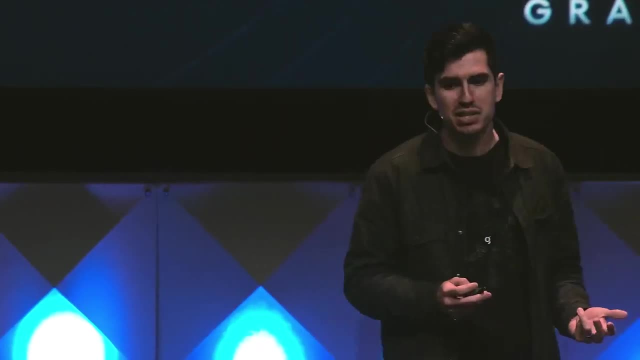 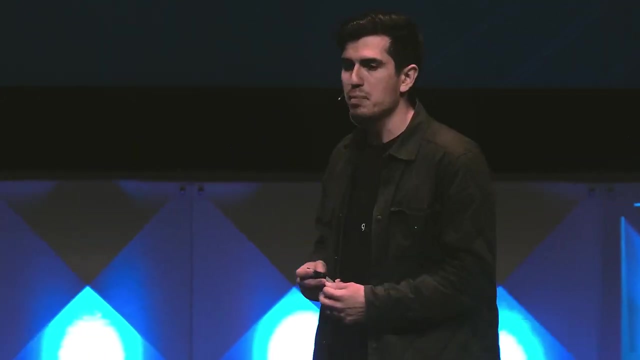 the benefits we hope to get from Web3 and decentralization in the first place. Indeed Afri, a notable Ethereum core developer, famously said that if we all end up accessing Ethereum through Infura, then we're going to be able to do a lot of things, And so 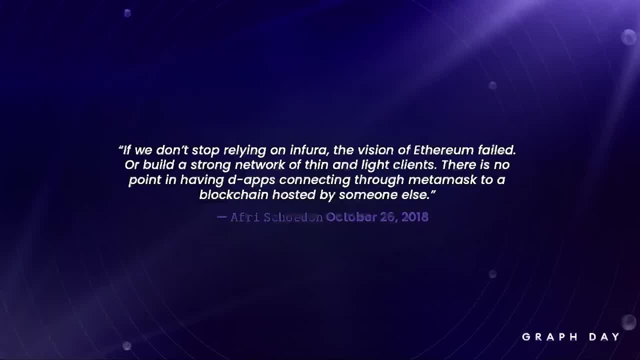 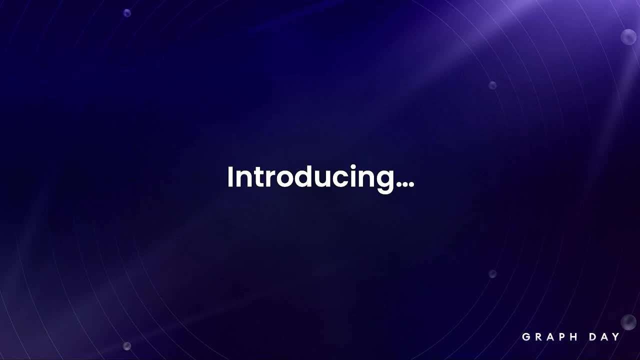 we're going to be able to do a lot of things. And so we're going to be able to do a lot of things, And so I'd like to introduce a new concept to you guys today, Since this is graph day. you can probably 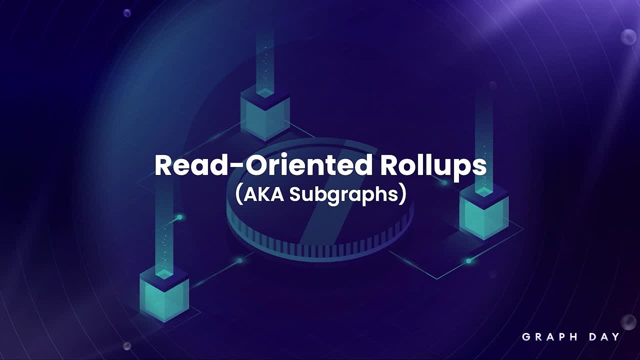 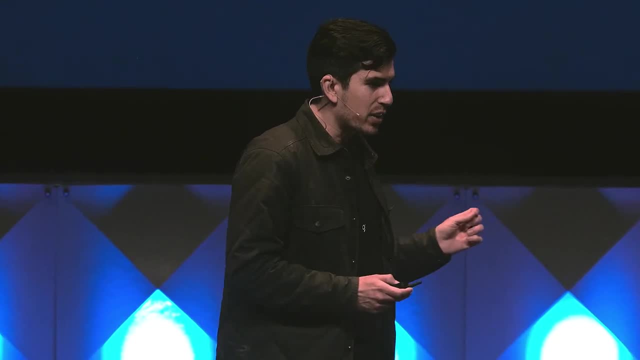 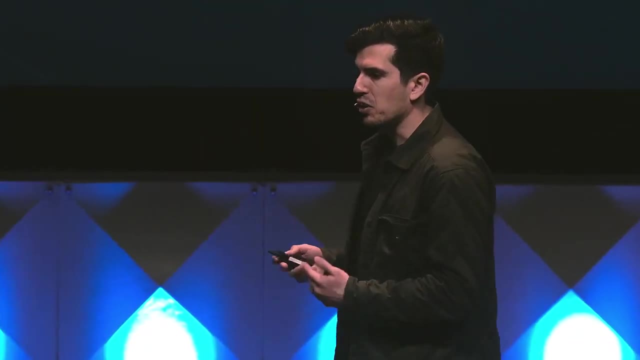 see where I'm going with this. We're going to talk about subgraphs, But in this context I want to talk about them as read-oriented rollups And to understand why I'm using that label in this context. let's do a quick recap of what rollups do today. They're a classic example. 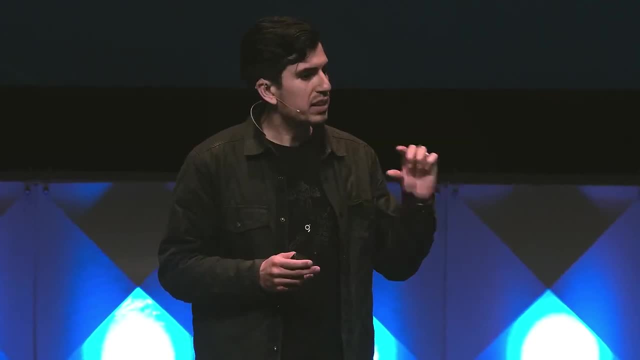 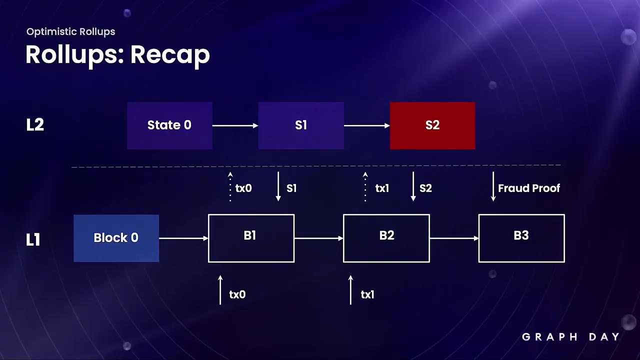 of this unbundling, where data availability and consensus stays on layer one, but state machine execution moves to layer two And specifically it's the transactions that are stored as like call data on Ethereum, And then you can either submit fraud proofs that a block on the layer two is incorrect. 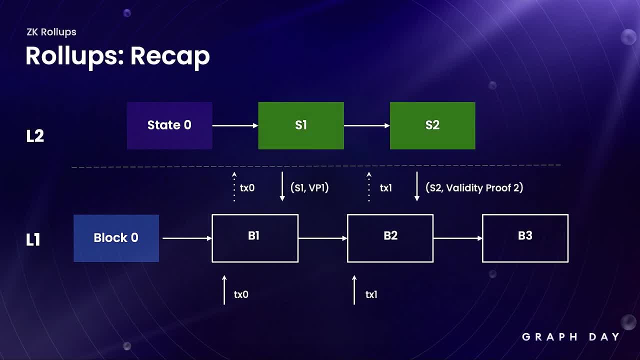 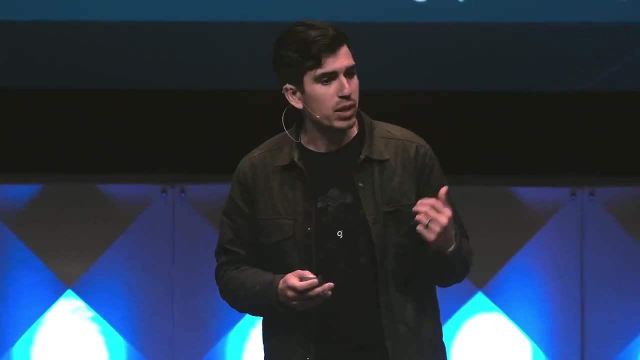 as in the optimistic use case or in the ZK rollup use case, you can get validity proofs that every block is correct and can be verified on layer one in real time. Now, read-oriented rollups support either of these patterns: the optimistic or the ZK pattern. 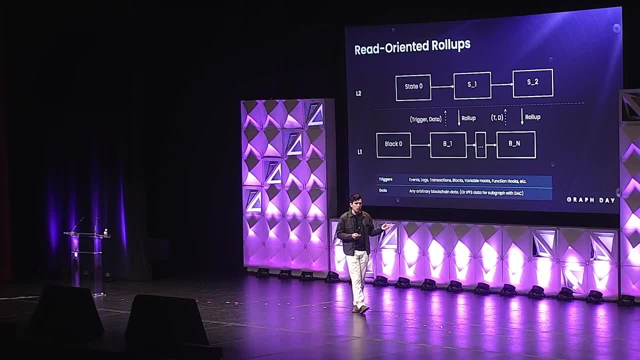 The main difference is that, whereas traditional write-oriented rollups use a transaction-oriented state machine where the users are submitting transactions with the expectation that they'll be sequenced in a certain way on the L2, be executed in a smart contract, read-oriented 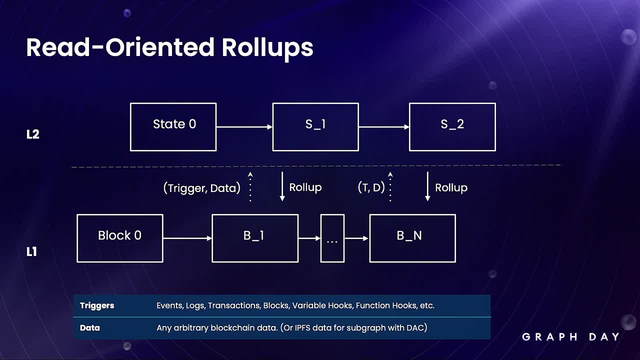 rollups support either of these patterns, And so the main difference is that, whereas traditional write-oriented rollups are all about producing the derived data that's necessary to use blockchain data for specific applications, So they can actually do arbitrary event sourcing or map. 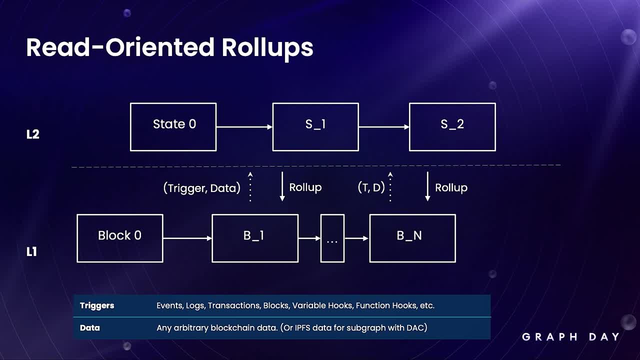 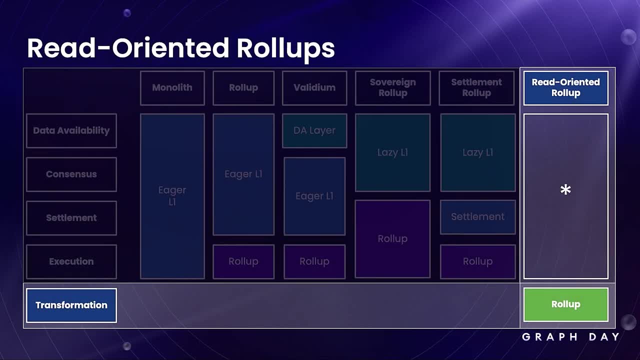 produce logic over any sets of triggers that exist on the layer one, But nonetheless they still rely on layer one for consensus and data availability, And so the new layer of the modular blockchain stack that I want to propose is this transformation layer, And that's really where 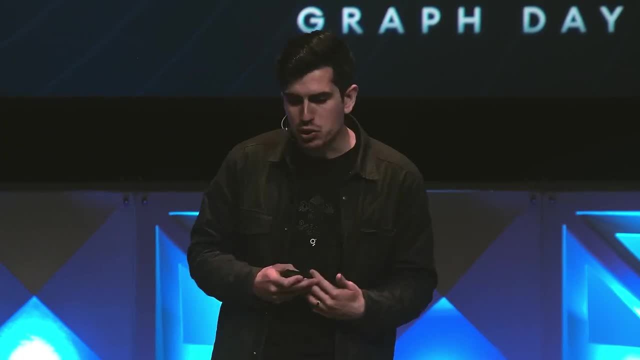 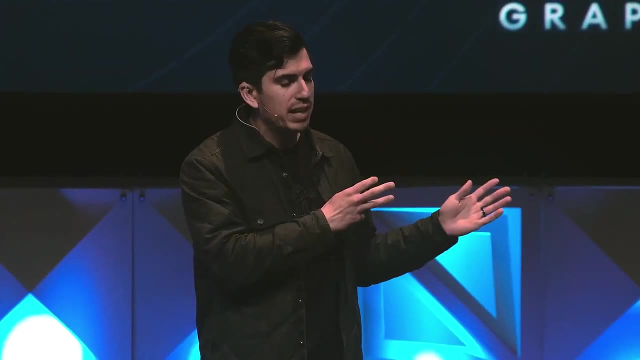 read-oriented rollups shine. It's not so much about the user a priori having an expectation of how they're going to change state in these read-oriented rollups. It's more that the users can have taken arbitrary actions in the past and these read-oriented rollups can be designed around the 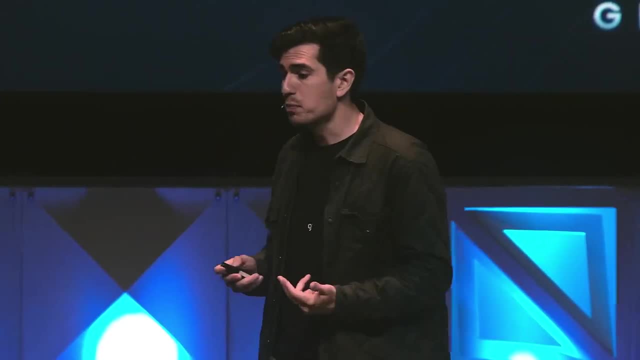 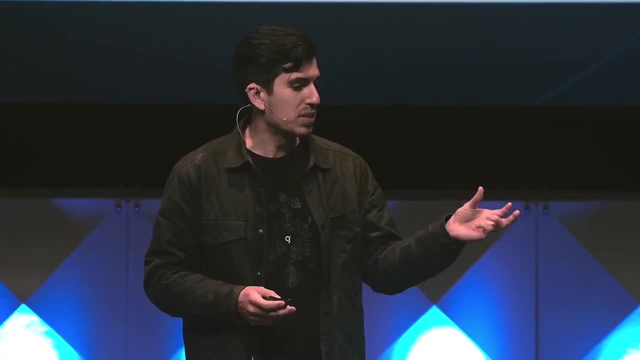 data that already exists on the chain. Importantly, they can support almost all of the design patterns that we see today. So I've talked more about rollups here, but the Validium's pattern, where data availability is handled on the chain and the data availability is handled on the chain. 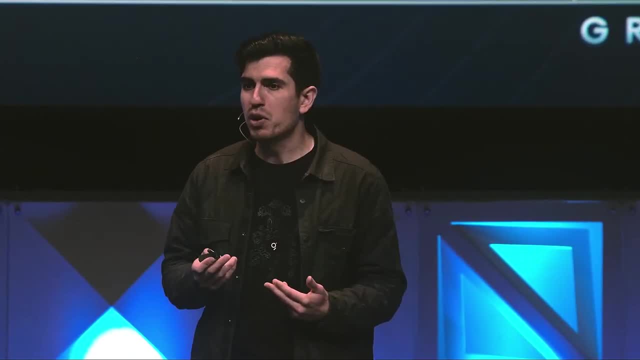 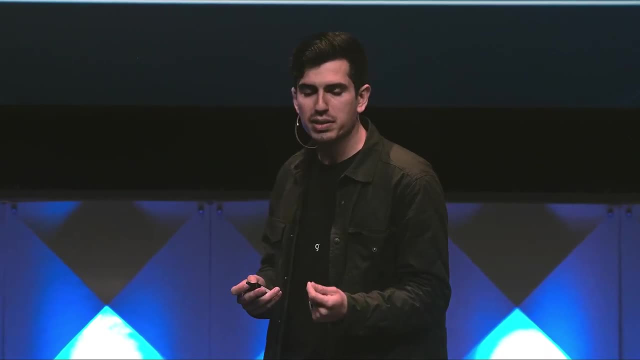 is handled on a separate layer is likely where subgraphs will need to go to support NFT use cases in the decentralized network where all the metadata is stored on IPFS and doesn't have layer one data availability guarantees. Importantly, like all rollups, these are: 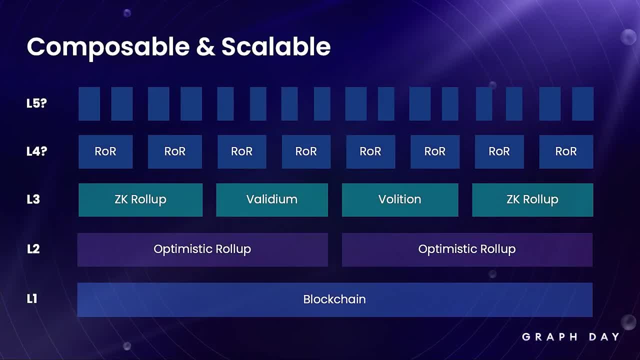 composable and scalable. So, in the same way that you can have Validium rollups verified in an optimistic rollup or in a ZK rollup, you can also have read-oriented rollups built on top of layer ones, other layer twos or indeed other read-oriented rollups. The case with 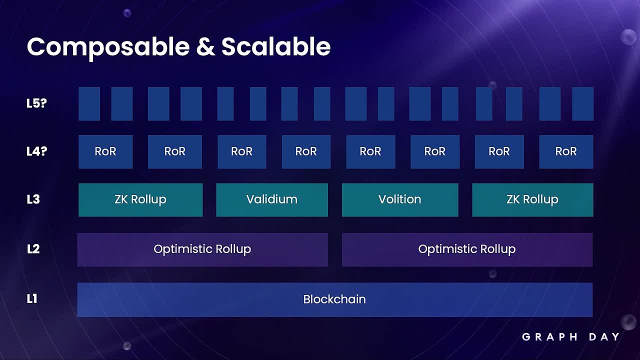 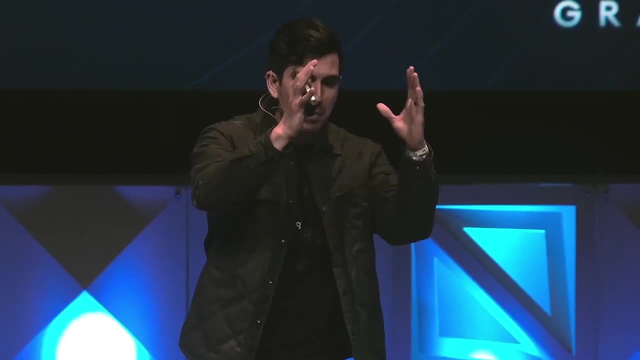 subgraph composition and some of the data pipeline execution models that you'll hear about later today. And this composability through sharding is what gets us the scalability benefits of rollups. It's that each person can focus on the small shard of computation that they're interested in. 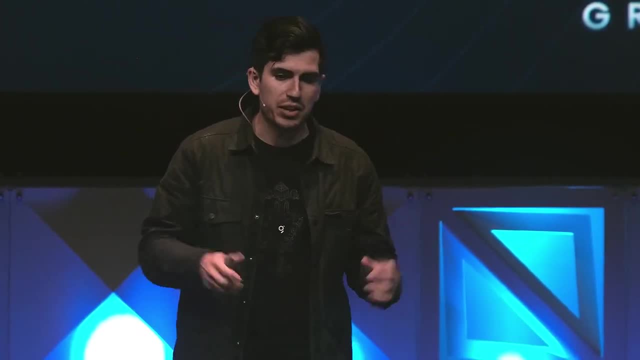 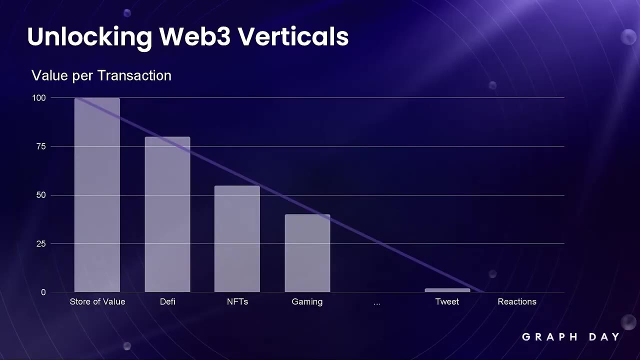 and the path back to the layer one, base layer. And when we think about scalability, it's not just scalability in a vacuum that we care about. it's really about unlocking more use cases for Web3.. So it's not surprising that the first use 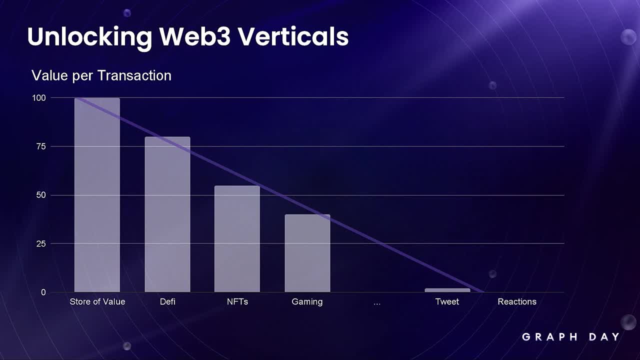 cases that had product market fit were the store value use cases, because you can send one transaction and store value indefinitely And as we move along the value per transaction curve to the far side, we get to like an individual tweet where maybe the value per transaction is. 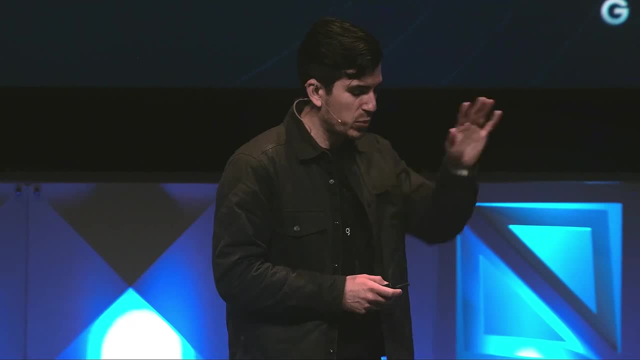 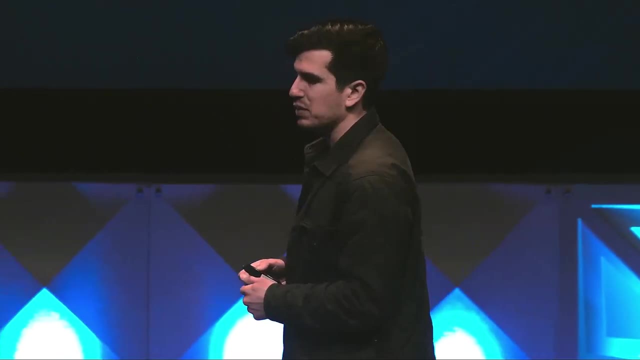 actually greater than the value of the transaction, And that's why I like to think about scalability. quite low. Everyone else's tweets, of course, Your tweets are great. The other benefit to read-oriented roll-ups is that they're natively provisioned and upgradable, at least as they exist in the graph, Because it's not important. 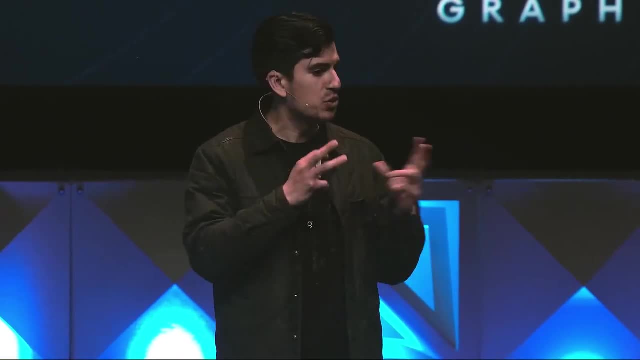 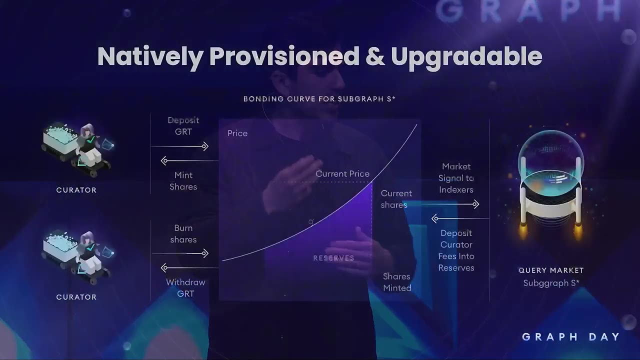 for the user to have an a priori mental model of how the state execution is going to happen, and it's really ex post definitions of the derived data. you can upgrade subgraphs. you can natively provision them all in the context of the graph using the curation mechanism. 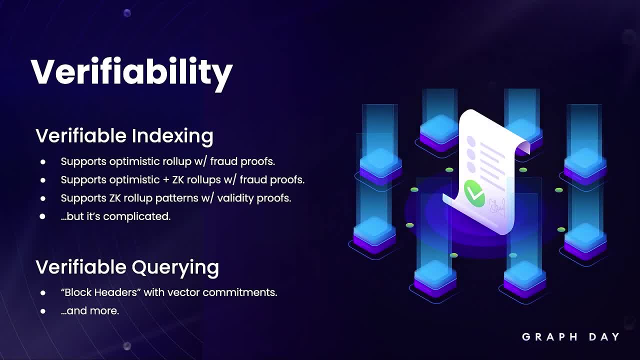 that Yaniv walked us through earlier, But we'd be remiss if we didn't talk about verifiability. right? If we're making the argument that subgraphs, read-oriented roll-ups, are part of the modular blockchain stack, then one of the most important things that blockchains do is they. 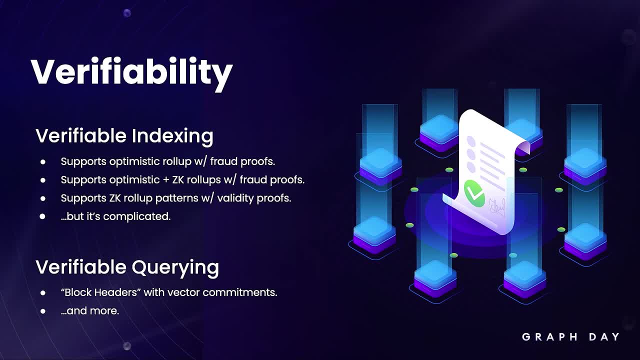 have these properties around. verifiability: In the context of the graph, we like to talk about verifiable indexing, verifiable querying For verifiable indexing. we support many of the patterns that we've seen today, with a caveat that it's a little. 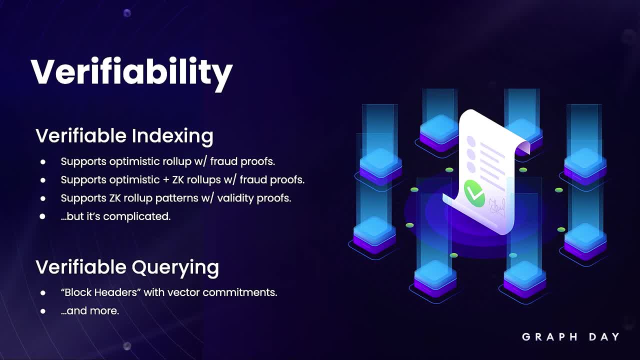 bit more complicated and we'll get to that in a second. And then, on the other side, we want to make sure that, once you've indexed a subgraph, that you can actually reach in query the data that you're interested in and have guarantees that that data is correct, Starting with verifiable 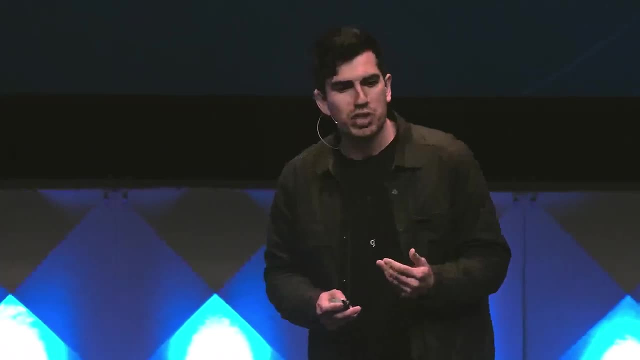 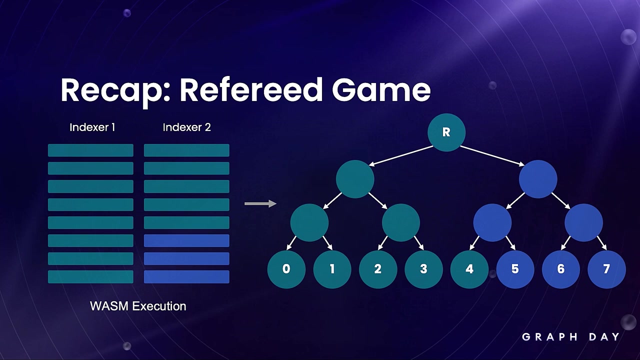 indexing. let's look at one example of how we can approach this, which is using a refereed game. This is a form of interactive fraud proof that's been put into production recently. layer two, such as Arbitrum. In this model, you look at the execution paths of two different 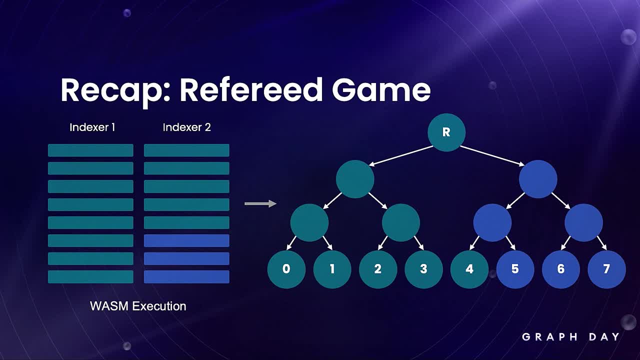 validators and you can run a sort of binary search to figure out where they diverged in execution and then recompute that single step of the computation on-chain. So that's kind of where the scalability benefits come in. is that you really only need to process this tiny bit? 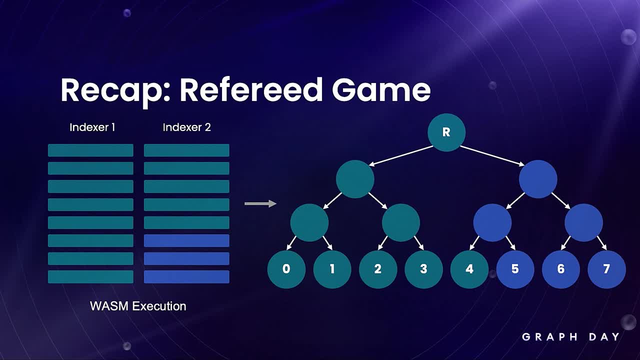 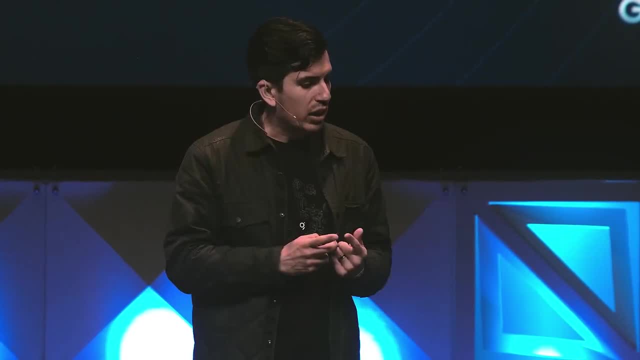 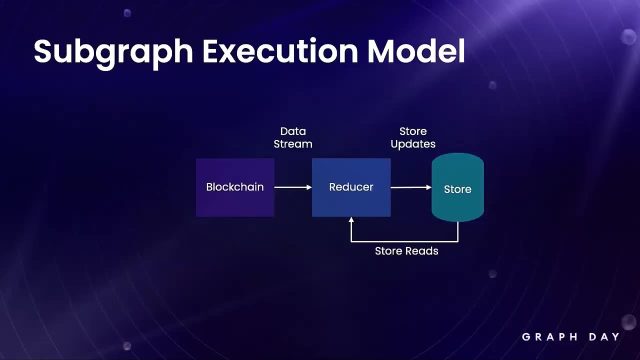 of computation on the layer one rather than the full computation In the subgraph use case. already our WASM computation, which is the subgraph mapping, is already a little bit more complex than what you'd see in a typical WASM program. Yes, there are steps that are sort of native or 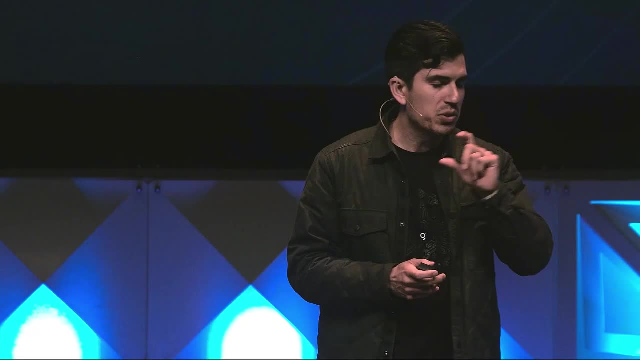 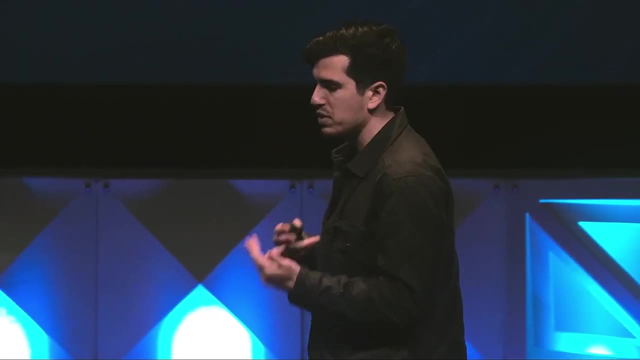 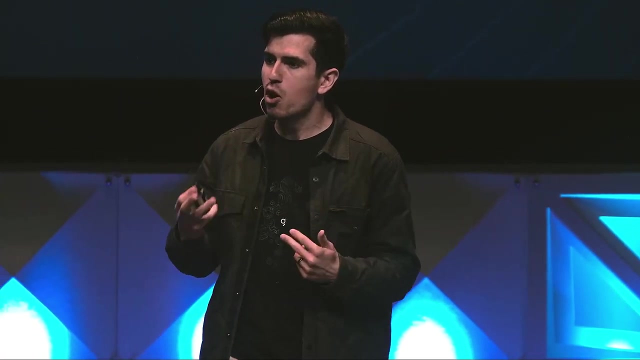 endogenous to the WASM module, but there's also computational steps that are calling out for more data from another blockchain or calling out for data that had previously been computed in the store, And this is only going to get more complex as the subgraph execution model evolves to support. 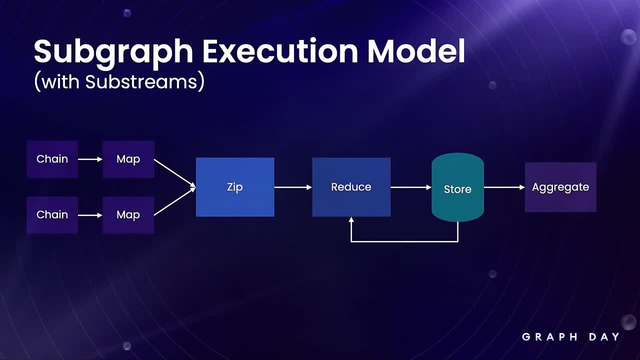 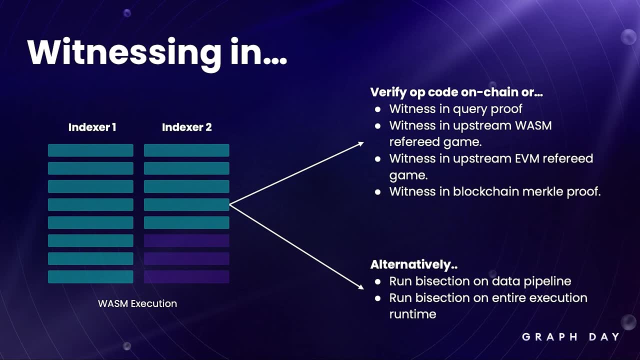 higher performance data. So we're going to look at the subgraph execution model and we're going to look at its use cases, as you're going to hear about from Sebastian of the Graph Council later today, And so what this means is that when we run this binary search to figure out where two 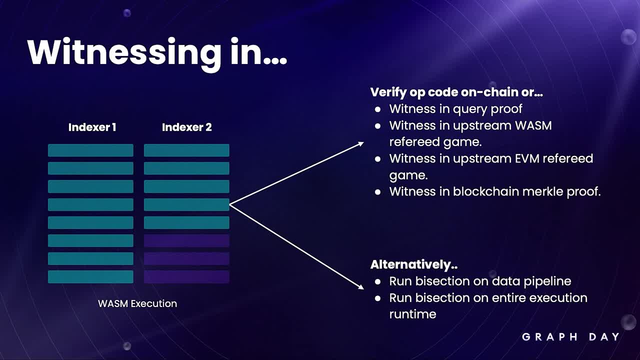 subgraphs' execution paths diverged. it might be that we're just rerunning an opcode on-chain, but it could also be that we're witnessing in proofs from other systems, such as an EVM-based refereed game or a query proof or a Merkle proof from an underlying blockchain. 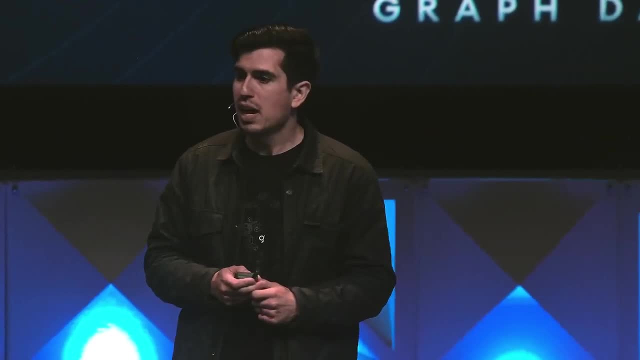 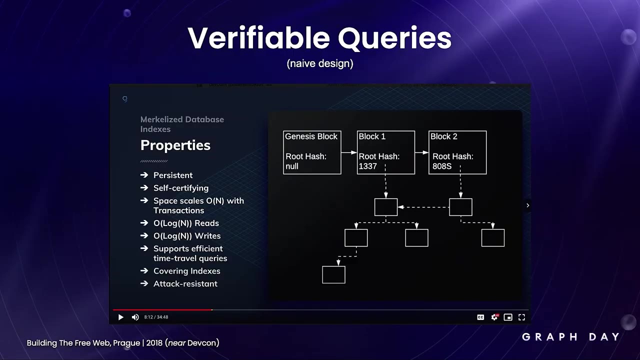 But the theory is there. This is really, at this point, an engineering challenge that our ecosystem needs to tackle together. On the verifiable query side, this is actually something that we've been thinking about for a number of years. This is a screenshot from a talk. 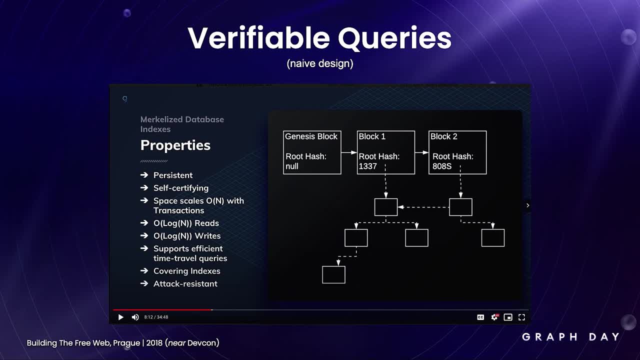 that I gave near DevCon. We weren't quite invited to speak at DevCon back then in 2018, where we presented this idea that maybe we could look at the database indexes that are in use today, the data structures that are used to power those indexes, and can we just come up with 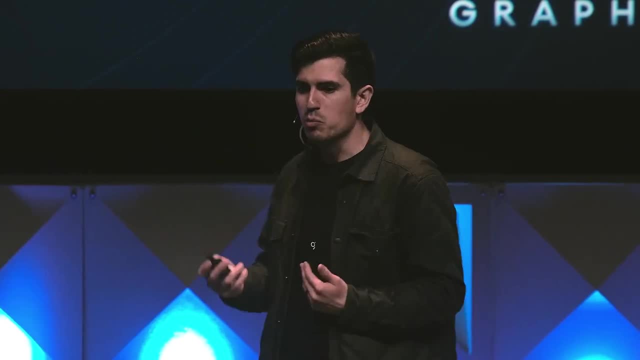 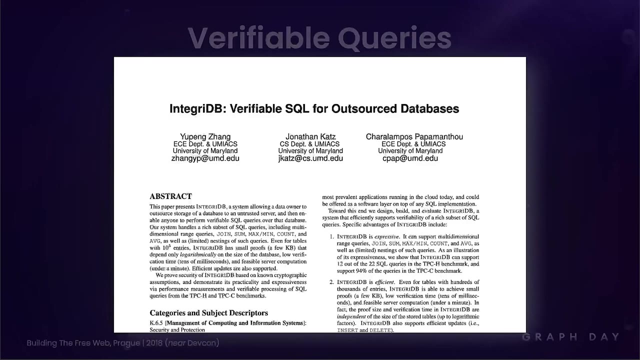 Merkle-ized versions of those indices. It seemed like a reasonable idea, And indeed that actually was part of what led us to stumble upon this line of research that's called outsourced databases. This is basically a line of research in academia that describes a setting in which consumers can 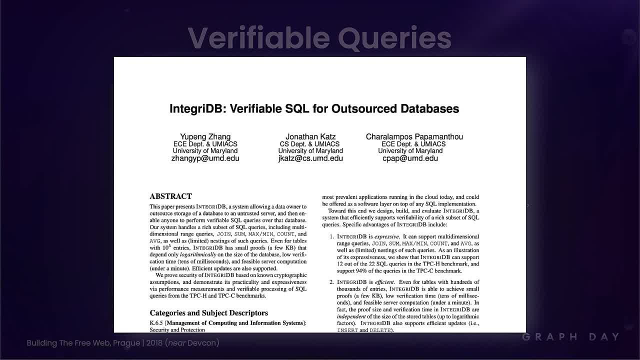 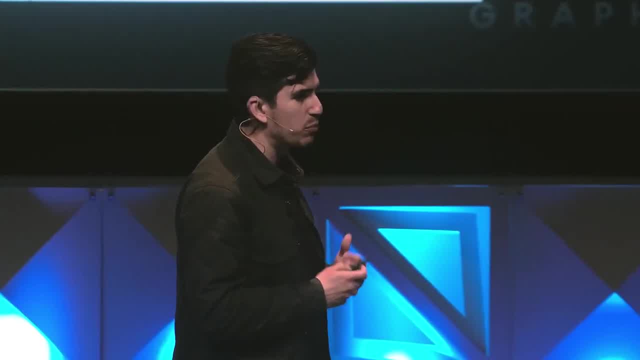 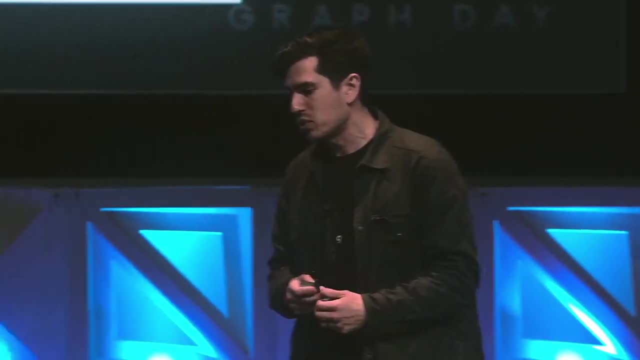 safely outsource queries to a server and trust the results without having any of that data locally on their machine. This paper in TegraDB actually approached this problem using authenticated data structures based on Merkle trees and traditional database data structures, But it wasn't quite as expressive. 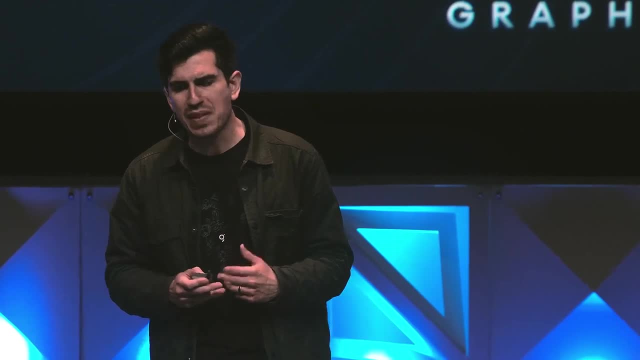 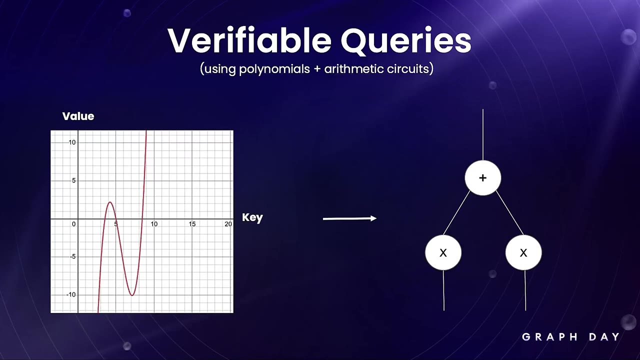 and efficient as we might like, And that's kind of what led us to look at a different type of authenticated data structure called polynomial commitments, And, as it turns out, with clever math, you can actually store all the data or represent all the data in a database. 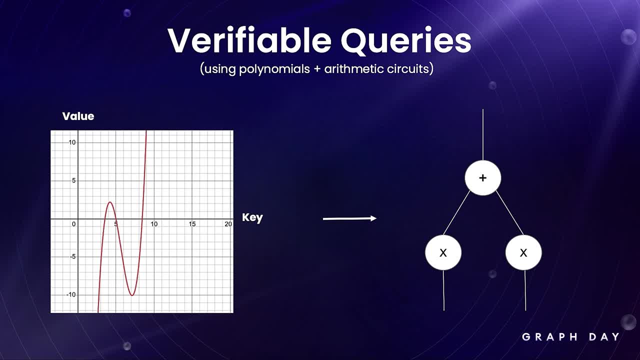 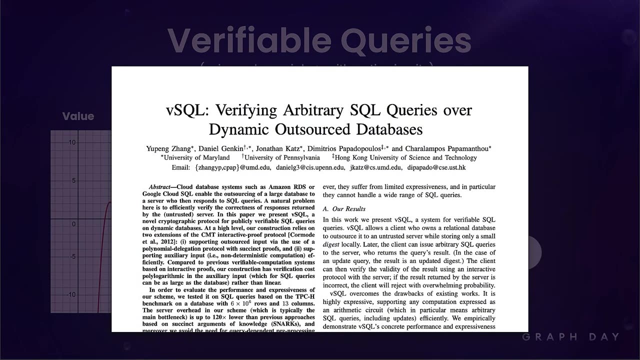 inside of a polynomial. And these things have the nice property that they tend to be more efficient across a number of different dimensions. but they also compose nicely with arithmetic circuits, which are one of the magical building blocks that powers your knowledge proofs. And indeed there's another notable paper in this line of research, called V-SQL, that 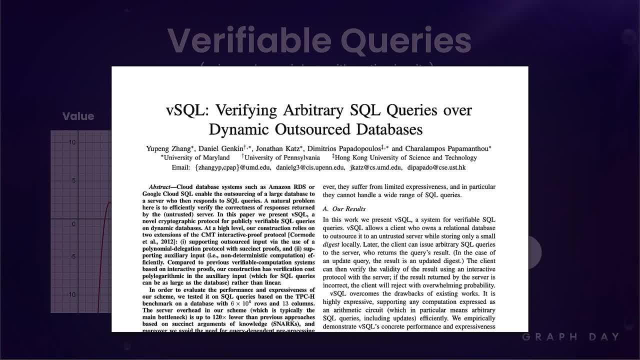 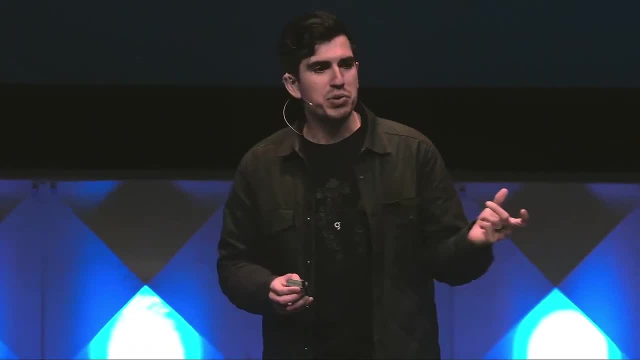 followed exactly this approach, And the exciting results, the exciting experimental results that you'll be hearing about from Zach Burns later today, were partly inspired by this lineage of research. Now, verifiability isn't something that we're just doing as a virtue signal. It's not just 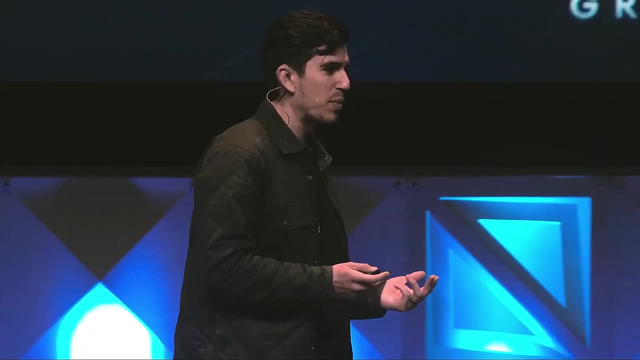 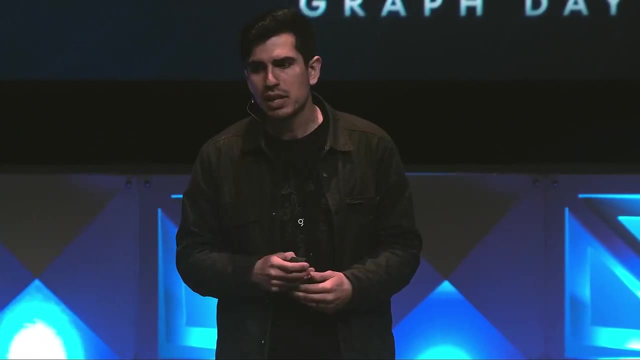 something we're doing to check the box of being a protocol in Web3.. We think this is going to have a meaningful impact on the use cases that we see the subgraphs and the graph applied towards. You know so, today most use cases are front-end use cases, right, Whether it's a read-only app. 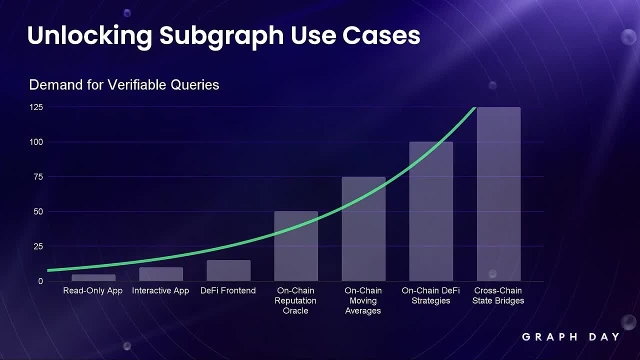 an interactive app, some kind of DeFi front-end, But there's a host of on-chain use cases that the graph has not really yet been applied to in earnest. You could imagine a subgraph acting as a reputation oracle, as we heard from Yaniv earlier today. You could imagine it being 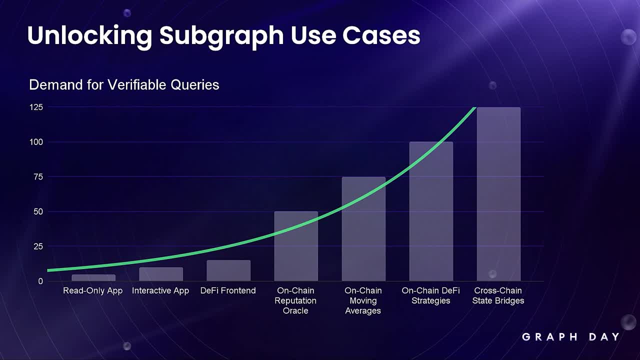 used as a price oracle or some kind of DeFi aggregations. You could even imagine it implementing Yearn-style automated trading strategies where the output of the strategy is bridged back onto the layer one or the lower level chain. And if you really trust the 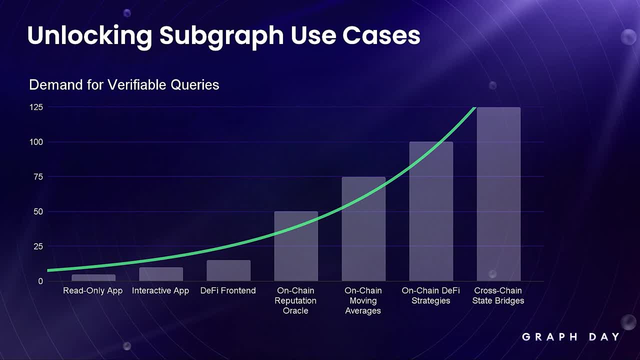 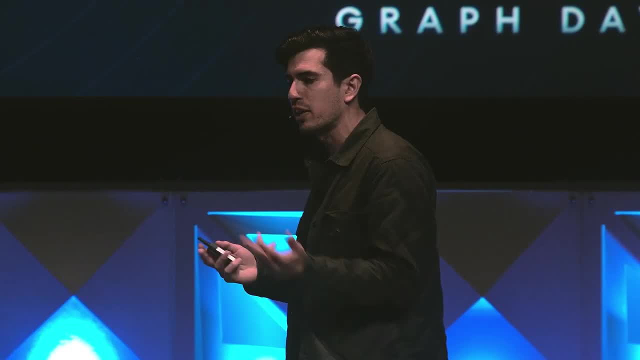 verifiability properties of the graph. you could even imagine using this in a cross-chain state managing use case. So today we tend to bridge really simple state across chains like a token balance. But imagine being able to bridge any arbitrary map reduce over some other chain. 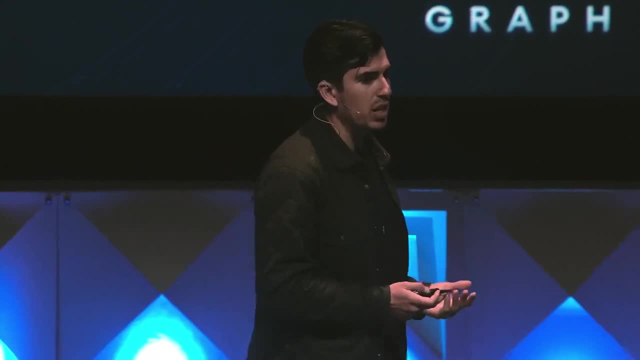 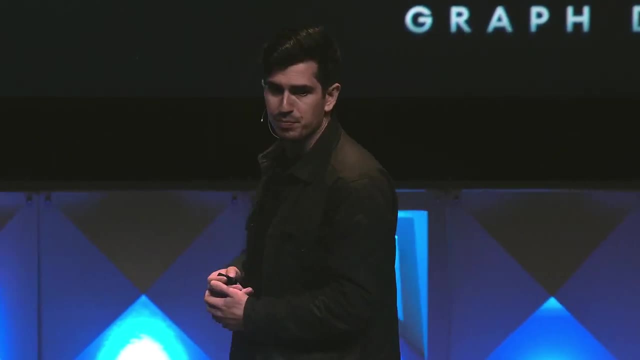 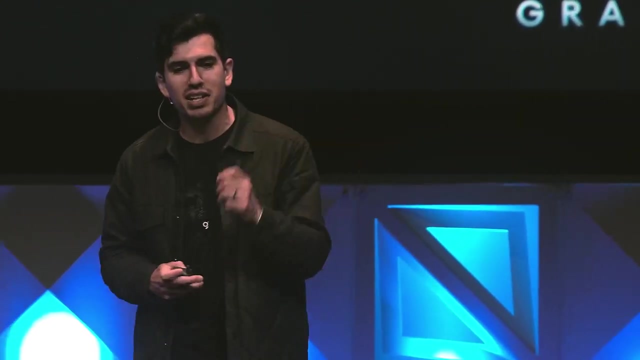 onto another chain. These are the types of use cases that become available to us once we take an earnest effort and focus on verifiability. Now, some people in our community have been a little ahead of the curve on testing the boundaries of what's possible. This is an 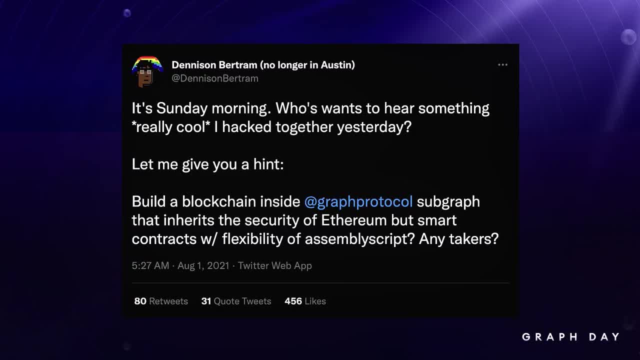 example that Denison, one of the subgraph developers in our ecosystem, ran last year where he re-implemented an ERC20 token inside of a subgraph, using the subgraph as a read-oriented roll-up where basically just the call data was stored on chain and then the state of the token. 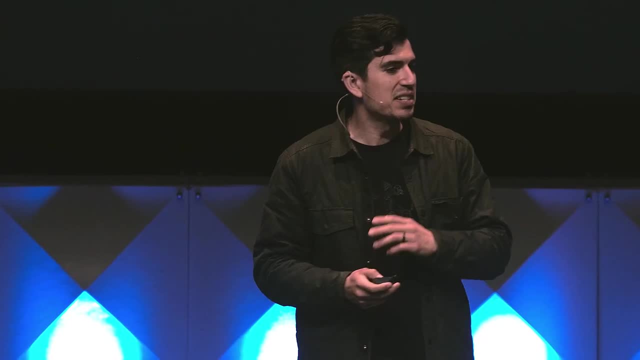 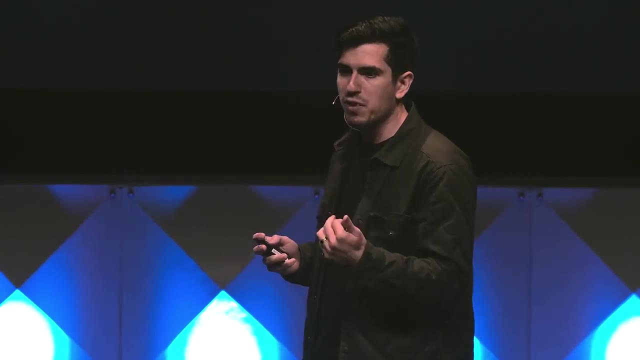 contract was basically all written in assembly script. Now, this isn't something I'd recommend doing today with the security model of the graph, but this is the kind of thing that would become trivial to do once verifiable indexing and verifiable queries has been delivered. 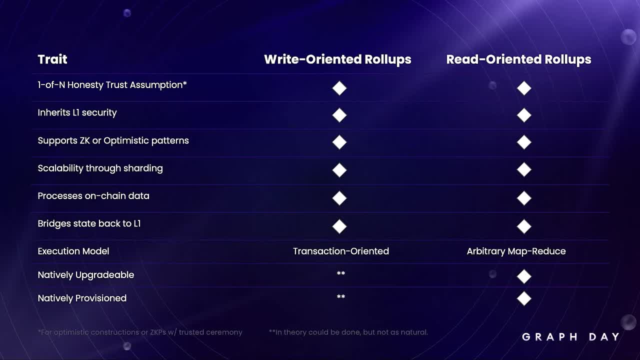 So to just recap really quickly: you know write-oriented read-ups, read-oriented read-ups, many of the same considerations. You know they have a one-of-n trust model. They have to design bridges. They take advantage of. you know the great unbundling, But the key difference is that 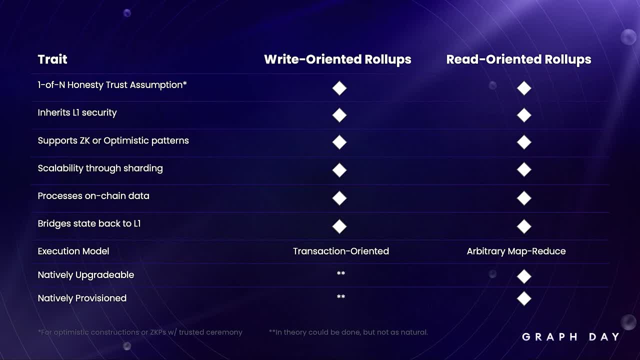 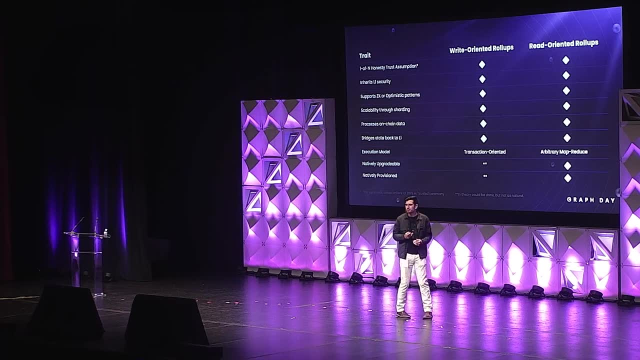 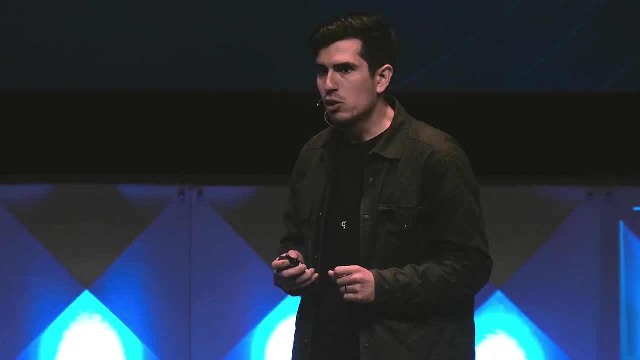 write-oriented read-ups are transaction-oriented state machines, whereas read-oriented roll-ups are arbitrary, map-produced operations and they're natively provisioned and upgradable. Now, admittedly, over the last few years, viewing the graph as a blockchain has not been our core. 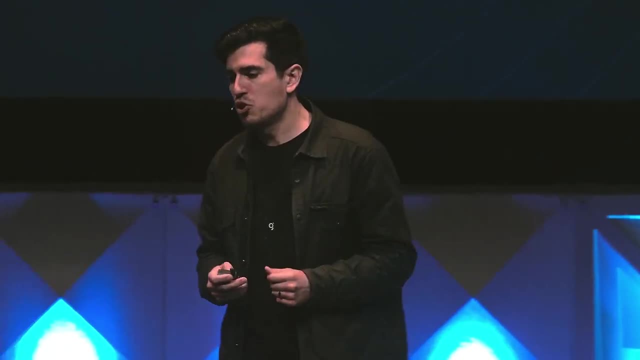 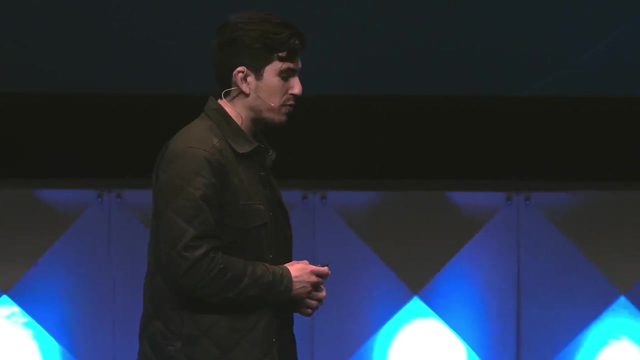 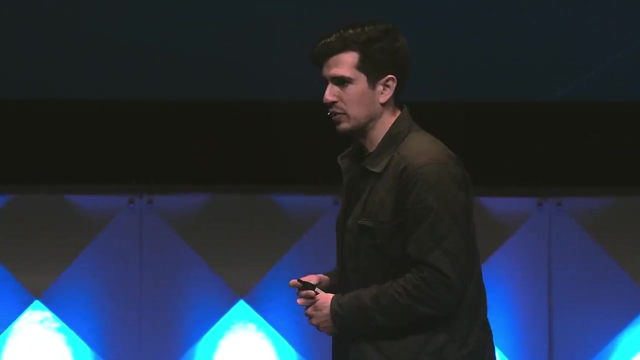 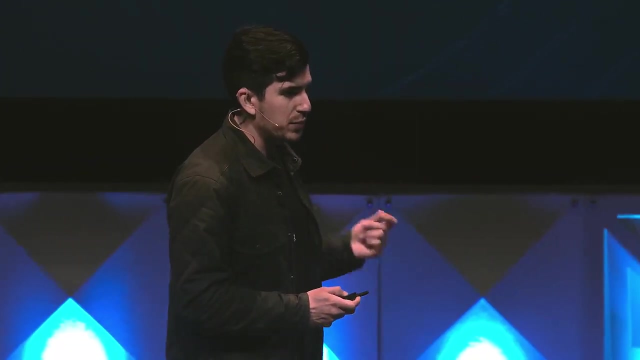 focus, although I do want to give a shout-out to Jackson Blazenski, who's really kept the torch burning on the verifiable queries research, at times by himself, and was integral to founding the cryptography working group within the graph ecosystem, So where most of our effort has been over the last few years, and rightfully so. 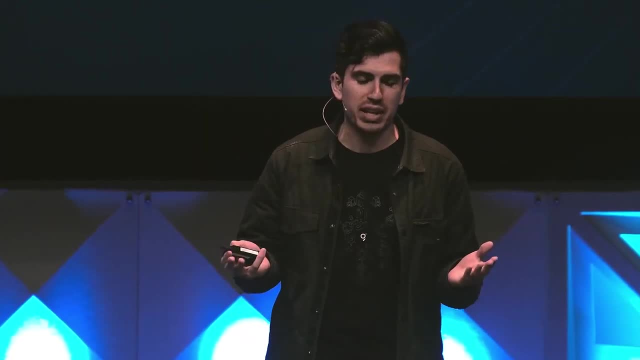 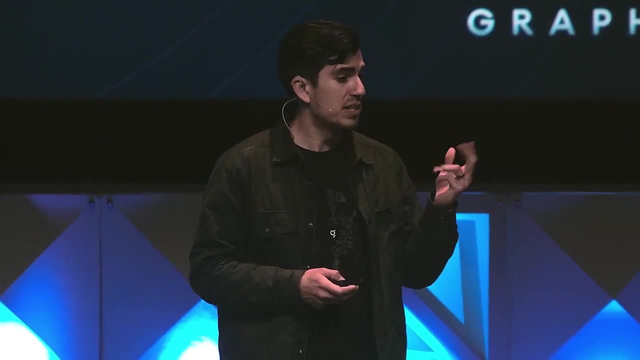 has been viewing the graph as a decentralized infrastructure market And the reason we started there is because the graph has had to handle incredible scale from essentially day one, And we're going to get into some of the challenges there, but before we do, because the challenges 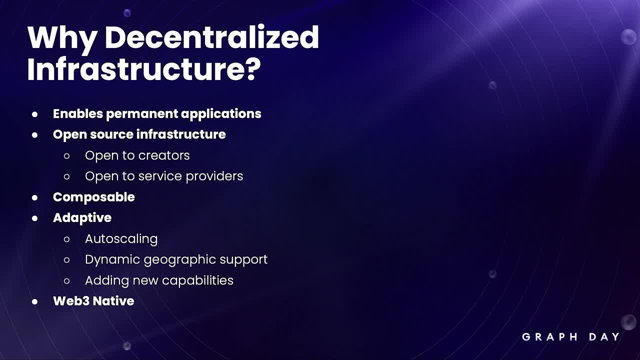 are daunting at times. let's focus on the benefits and why we're trying to overcome challenges. So let's talk about some of the challenges involved in building this in a decentralized way. So all of us are familiar with Web3.. I think we've heard a lot of the familiar benefits. 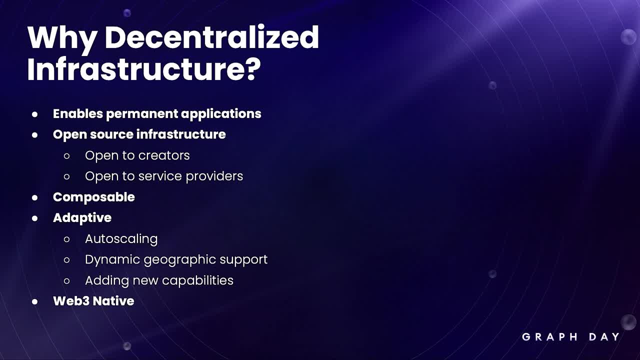 like being able to build permanent applications. The graph in particular, I think, is a great example of open-source infrastructure. So a lot of us are used to open-source software, where one developer solves a problem for themselves, publishes it as a library, other developers 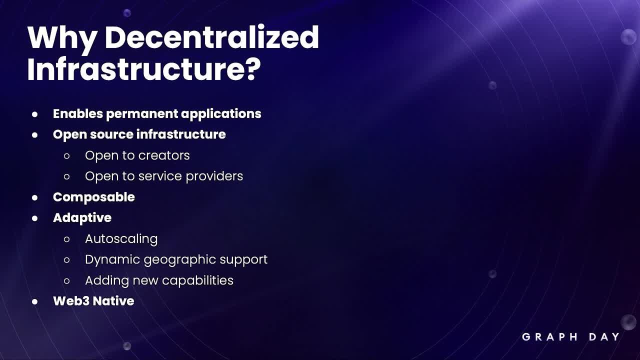 can build on that, remix it. Open-source infrastructure gives you all the same benefits, but for actual running software. So when someone solves a problem for themselves by building the subgraph, they've now solved that problem for everyone else that needs to use that type of data, And with. 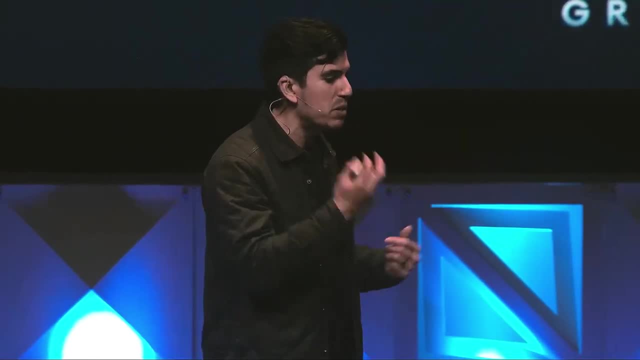 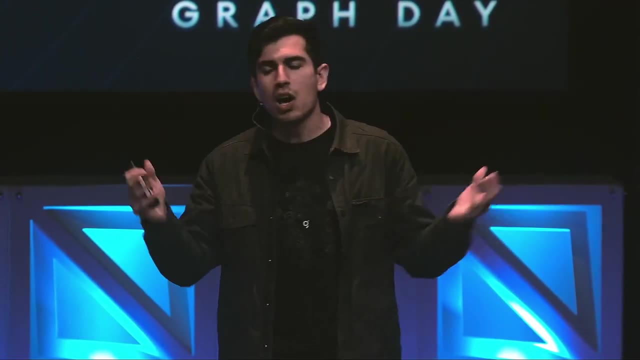 the advent of subgraph composition, people will be able to keep building on and remixing with the logic that's already been published to the graph today. So over time, the network will just become this rich tapestry of open, decentralized APIs that you can interact with. 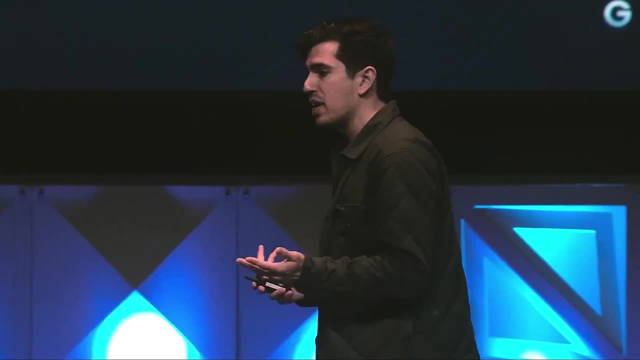 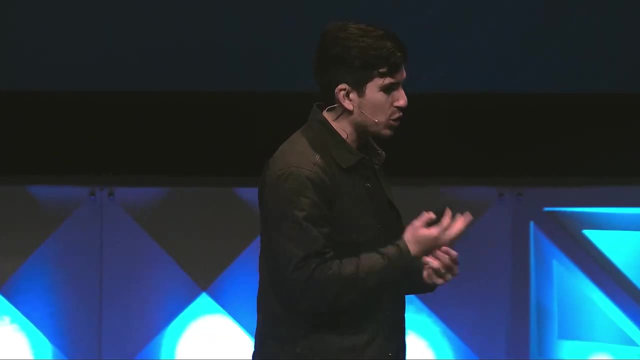 Importantly, the service providers that are serving these APIs are completely open and easy to use. So we're going to talk a little bit about that in just a few minutes. So open-source infrastructure is open and adaptable. That means you know there's no centralized 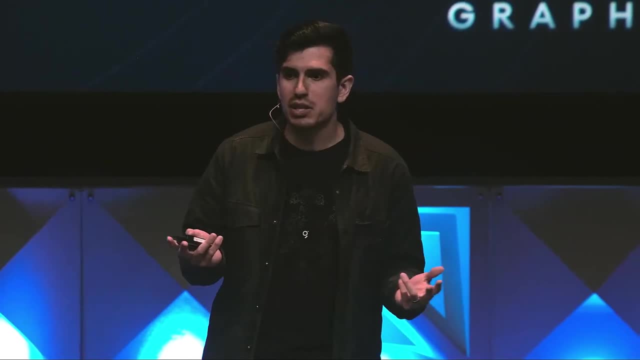 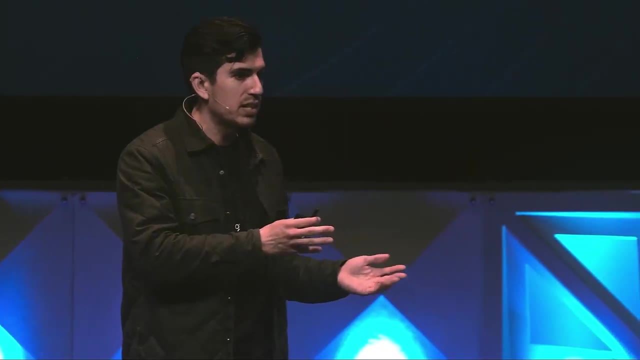 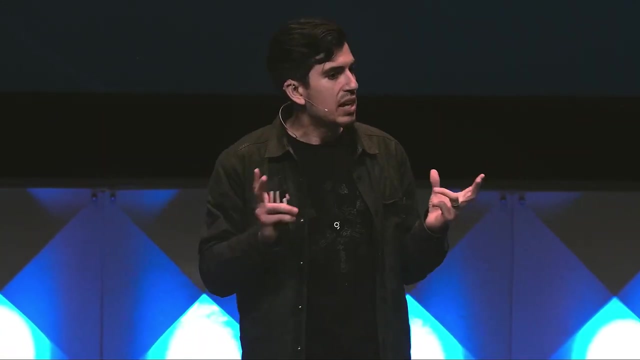 entity controlling them. They're responding in real-time to incentives, And those incentives lead them to do things like autoscale provision, more resources, service different geographies, add more database indices, caching layers to optimize their setup. All of that sort of happens in an uncoordinated, decentralized way to deliver a superior quality of service. 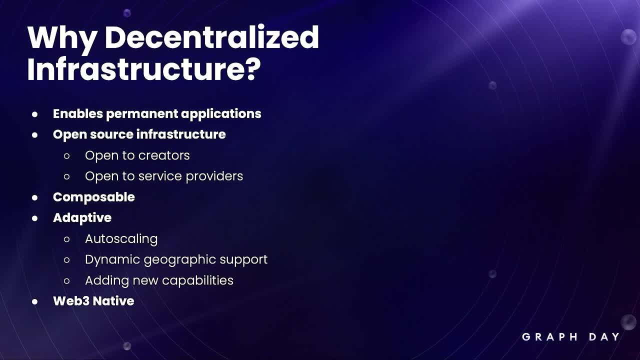 to the end user, And the last benefit I want to focus on today, because it's one that I think we've had some interesting progress on over the last year or two, is just the fact that the graph is Web3 native, And I want to highlight a couple examples of what that means. We heard from a couple speakers. 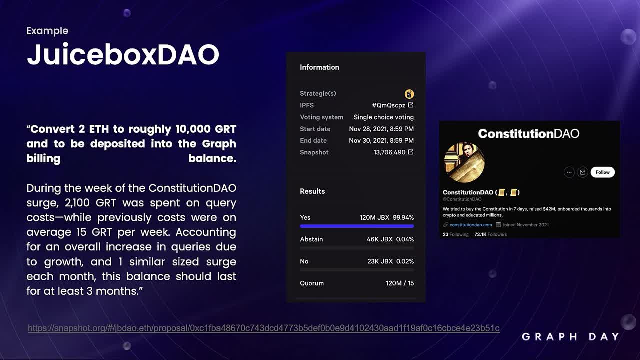 earlier today about Constitution DAO running on Juicebox which deployed to the decentralized network. I think it's super cool that you can actually go to the snapshot vote for the Juicebox DAO and you can see this DAO provisioning resources to power the subgraph that they 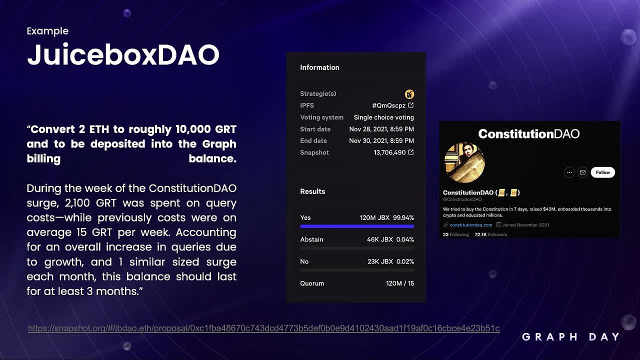 used to drive the fundraising platform that then went on to power, the Constitution DAO And a lot of us that have participated in DAOs. we may lament that most of the services that we want to use are outside of the trust boundary of the DAO. So you might create the Advocates DAO. 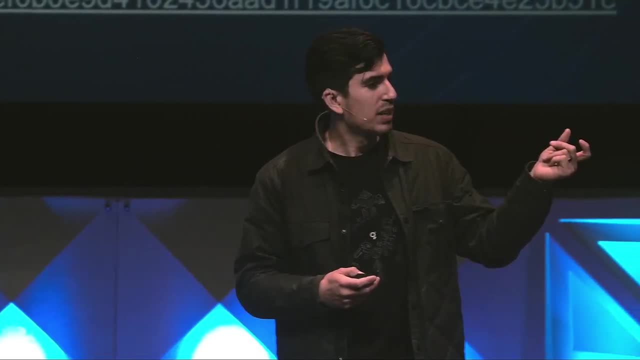 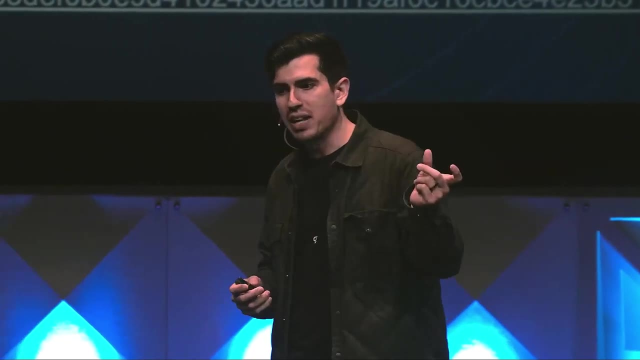 for example, but then that Advocates DAO needs a Twitter account and that Twitter account needs to be owned by an individual. It can't be owned by an individual. It can't be owned by an individual. It can't be owned by the entire DAO. The integration points are there. It's not Web3. 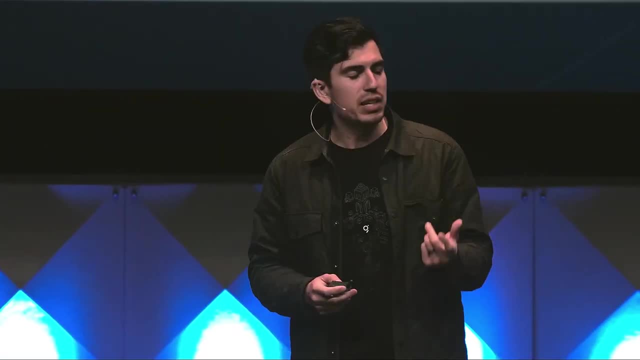 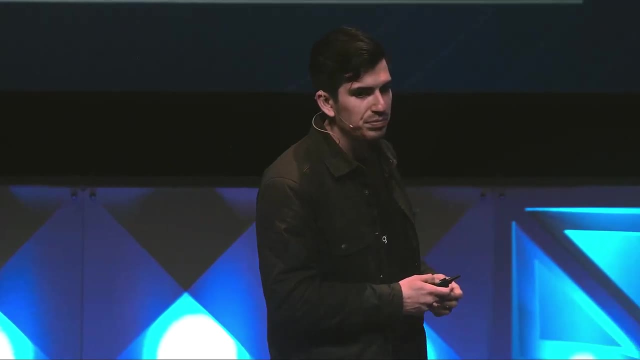 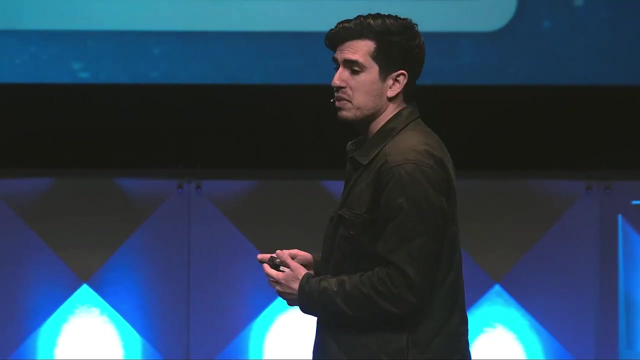 native, But when you're using the graph, the DAO can natively manage and control their subgraphs using the permission model and structure that's been embedded into the DAO. Another great example of Web3 native capabilities in the graph is the fact that subgraphs are just 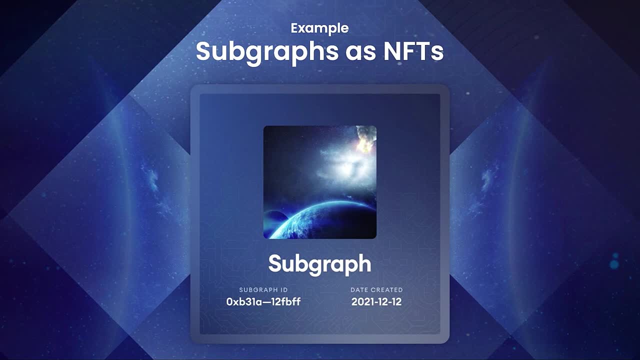 NFTs. So owning the subgraph confers a number of really important rights to the subgraph owner. You can do things like upgrade the subgraph. You can, you know, migrate the subgraph to the subgraph owner. You can upgrade the subgraph to the subgraph owner. 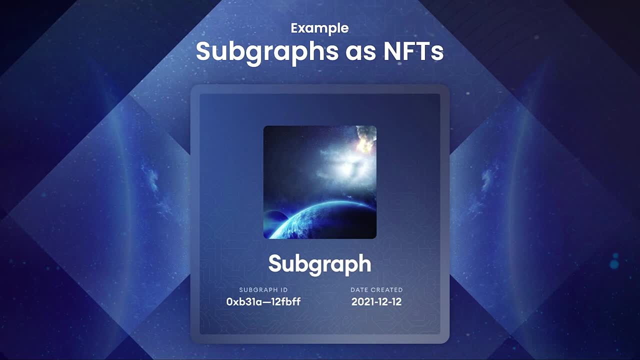 You can, you know, migrate the subgraph to the subgraph owner. You can, you know, migrate the curated stake on that subgraph. And we've heard from a lot of users that, hey, like sometimes you want to have, you know, an individual, start building the subgraph and 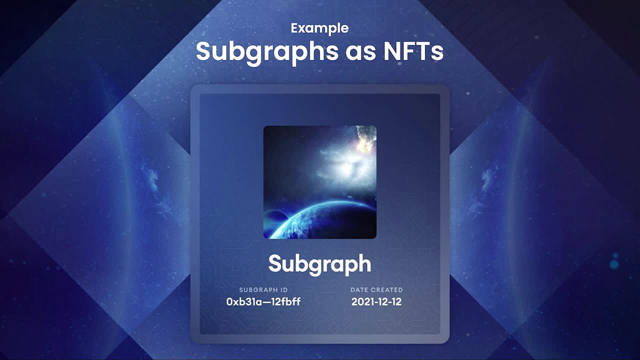 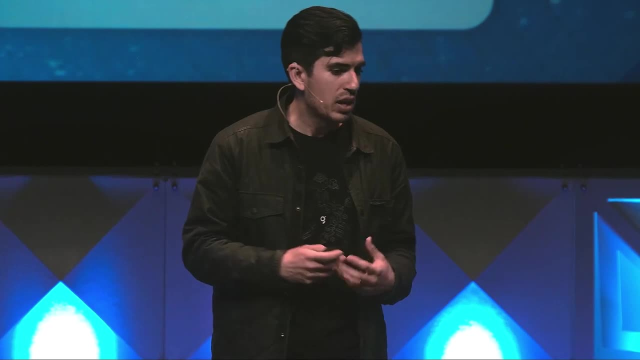 transfer it to a DAO. Sometimes you might be working with a dev shop, And so we solved that problem by just making subgraphs, NFTs, And so now they're digitally native, transferable, ownable items. They can integrate with DeFi. You could, you know, use it in all sorts of. 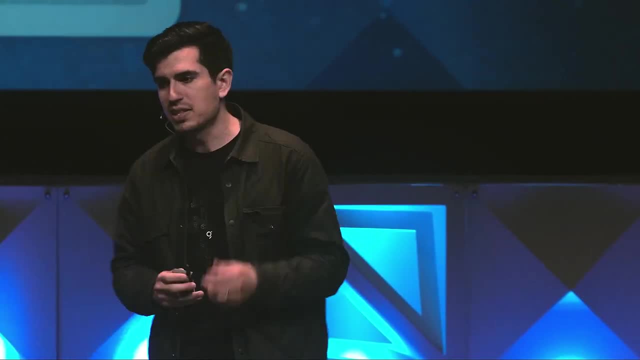 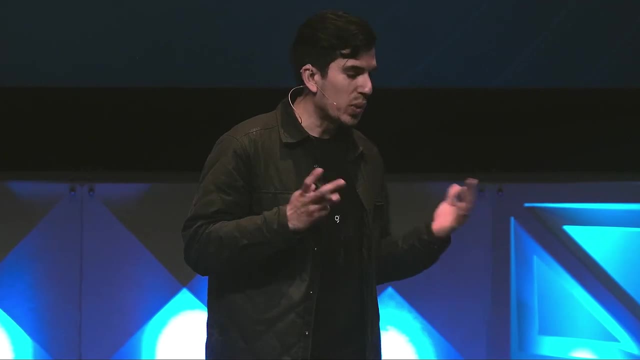 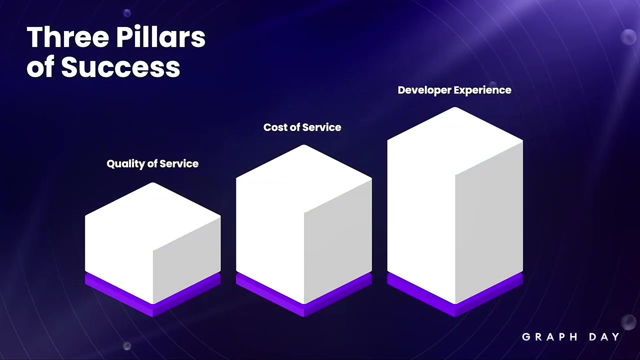 you know DeFi composability use cases, So it's- I think it's a fantastic use case for NFTs that are more than just a JPEG. So what does it take to make a decentralized infrastructure market successful? I would argue that there's three main pillars that are closely interrelated in subtle ways. 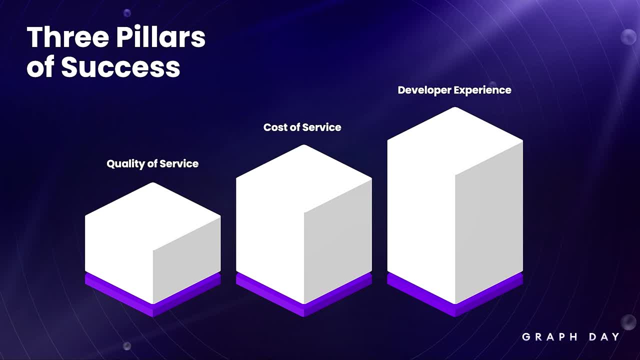 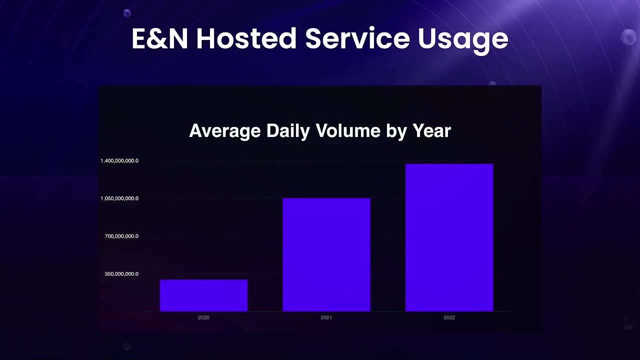 that we'll get into, And those are quality of service, cost of service and developer experience. So let's get into it. One of the challenges with quality of service, as I noted before, is the incredible volume of the service, And so I think it's a fantastic use case for NFTs that are 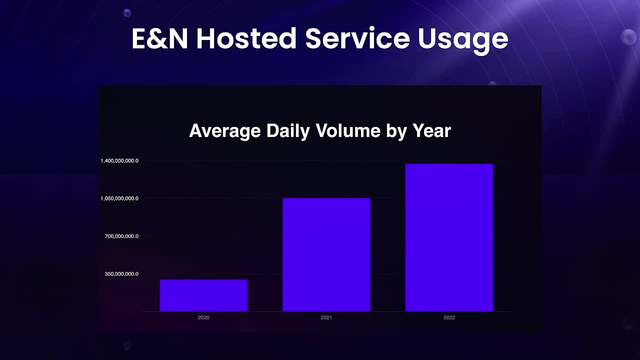 more than just a JPEG, And so I think it's a fantastic use case for NFTs that are closely interrelated in subtle ways that we've been processing from day one, But, you know, most recently it's not uncommon to be over. 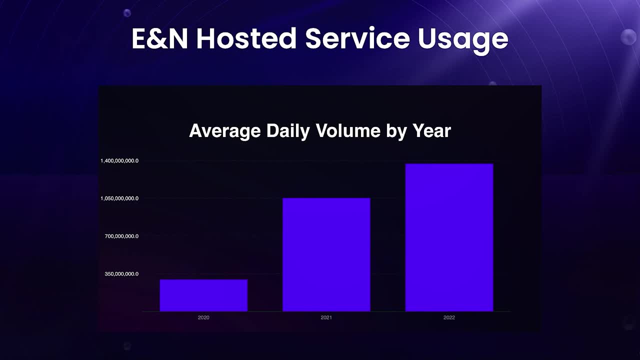 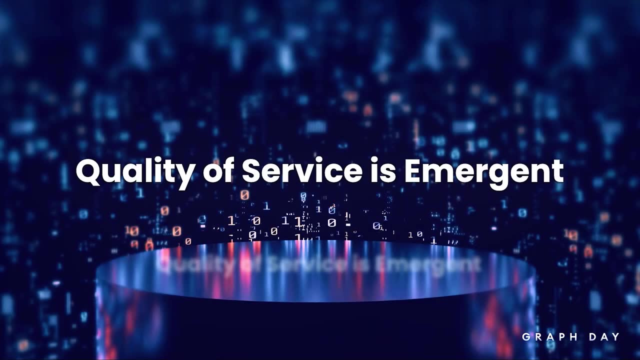 a billion queries per day. So that's really why we had to start from the scalability perspective and move towards verifiability. And the other big challenge with quality of service is that it's emergent. We don't control the nodes, We don't control the infrastructure- right We get. 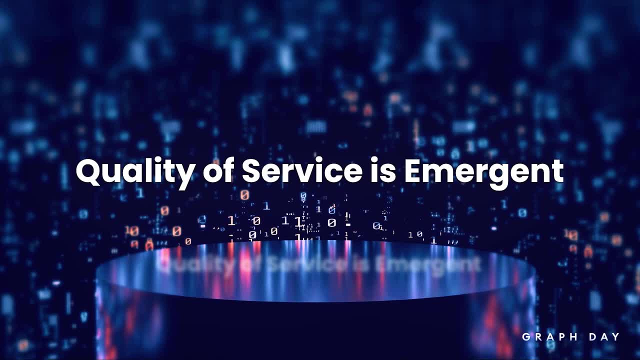 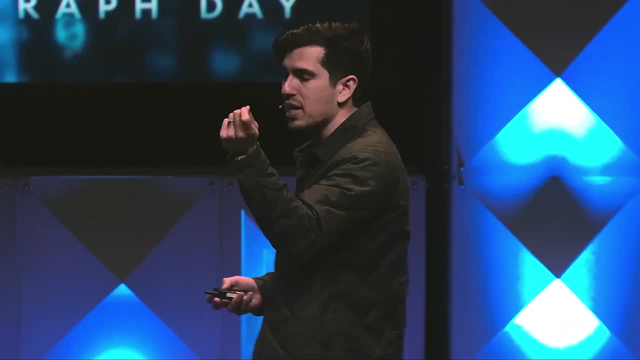 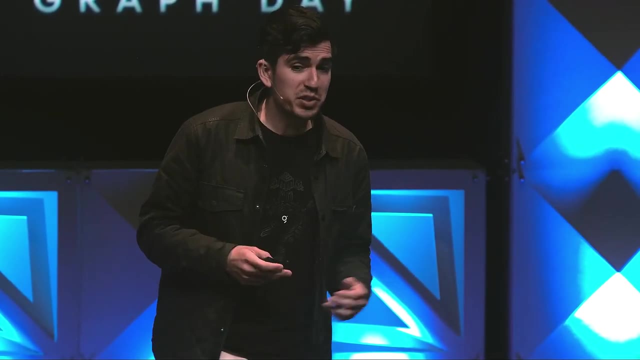 absorb the data. We can't directly absorb the data. We can't directly absorb the data. We can't directly observe from the blockchain what the you know uptime of a given indexer is. And despite all those challenges, quality of service is pretty good, Like you can see here that on many days. 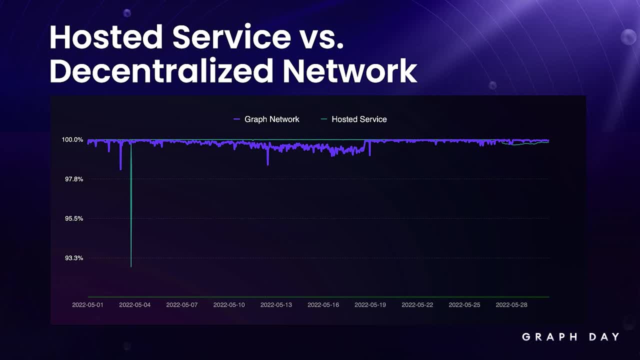 the decentralized network keeps up just fine with Edge and Node's hosted service. There's even times when the Edge and Node hosted service has had significant outages and the decentralized network has been more robust. But pretty good is not good enough, right? We're operating in a space. 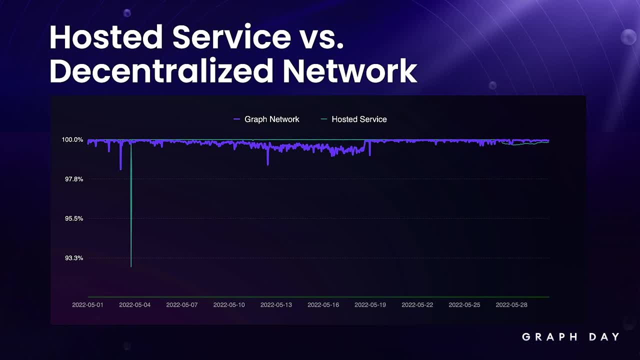 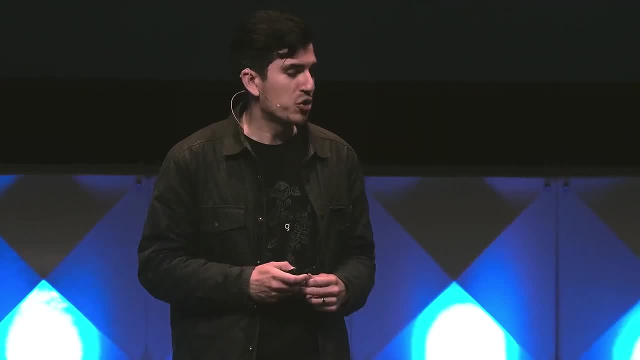 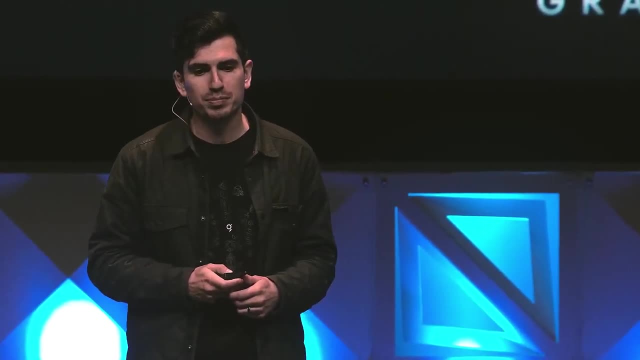 where people are comparing the graph to Web2 analogs. you know where they're used to: five nines of SLA right, Five nines of uptime. So this is something that we want to keep pushing ourselves on until the graph can be as performant and as stable as is humanly possible. A big part. 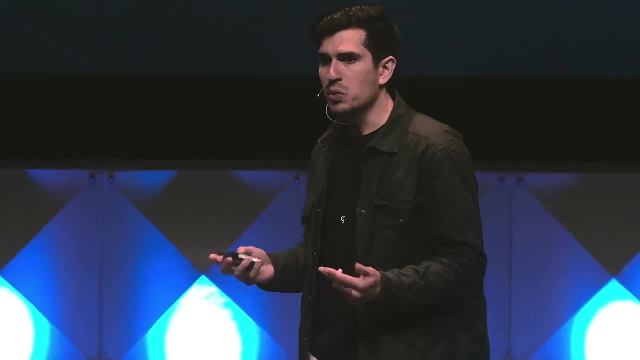 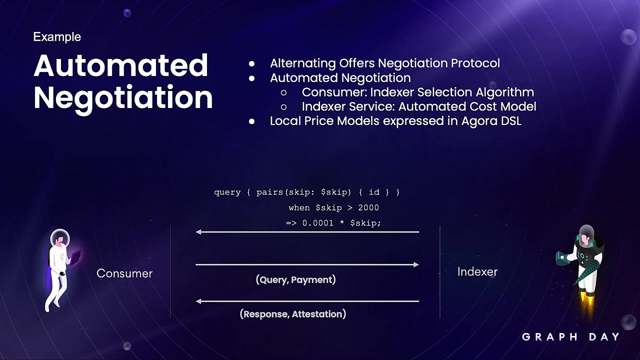 of the driver of quality service is the query market. So we have this automated negotiation protocol that you heard a little bit about earlier today, where there's alternating offers between the consumer and the indexer, And the indexer can communicate prices to the consumer using a. 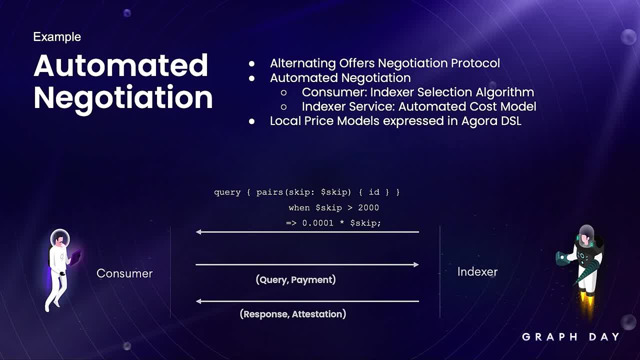 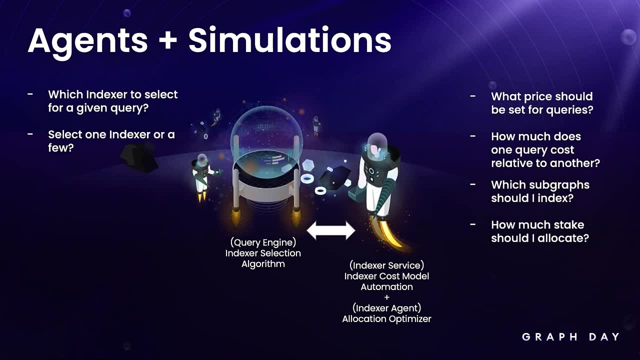 domain-specific language called Agora, designed by Edge and Node's own, Zach Burns. And, importantly, when I talk about negotiation, I'm not talking about two humans, you know, sitting at a table negotiating with each other. hey, how much is this query going to cost? that's worth fractions of. 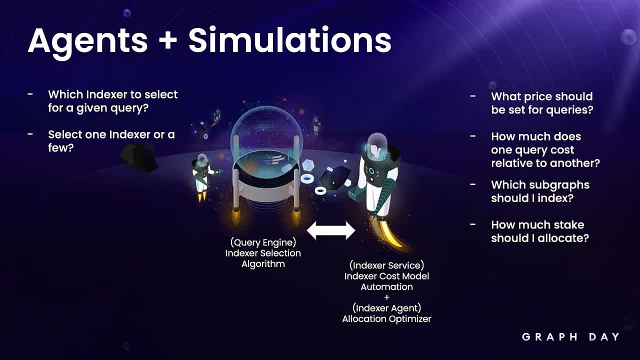 you know a fraction of a penny. That would introduce so much mental transaction overhead that it would cause a lot of trouble. So I'm not talking about two humans sitting at a table. that would completely obviate all the benefits that we get from a decentralized infrastructure. 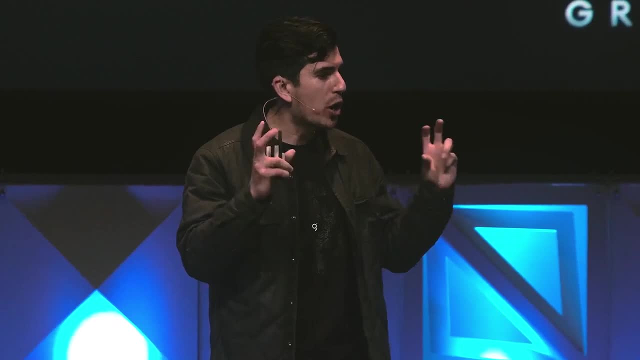 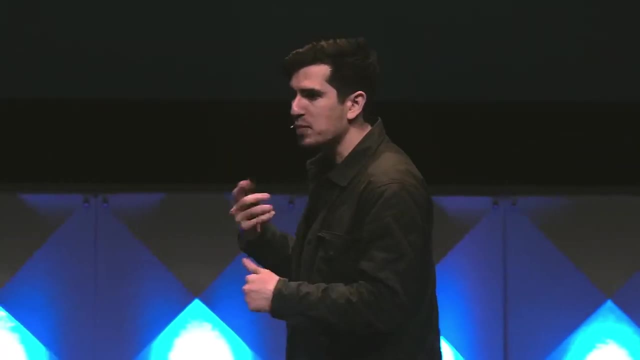 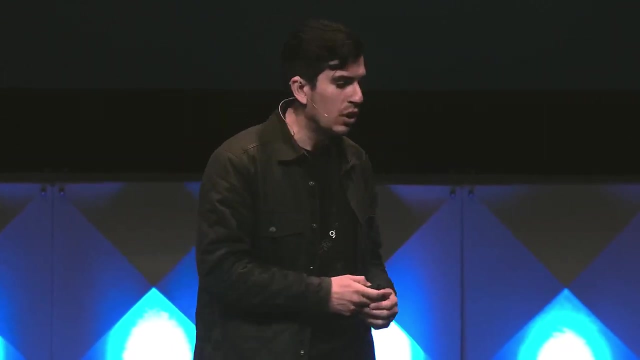 layer. Instead, what we're talking about are automated negotiating agents on either side of that marketplace that are in real time optimizing their decisions based on preferences that have been input to them by their respective owners. On the consumer side, we have the indexer selection. 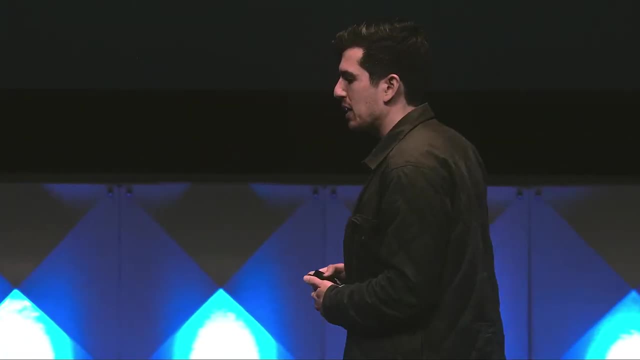 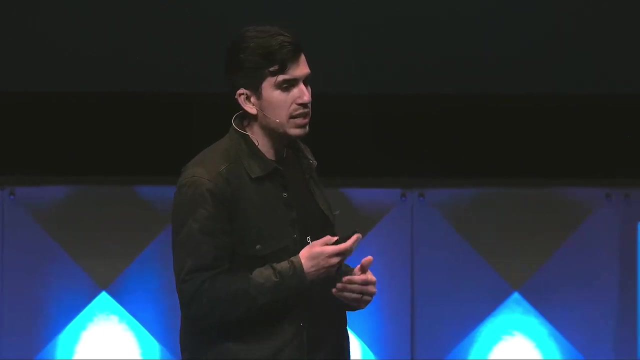 algorithm. On the indexer side we have the indexer service And on the consumer side we have the indexer agent that sets prices And we also have the indexer agent that decides which subgraphs to even index in the first place. And I'm excited to announce that this week we're launching two. 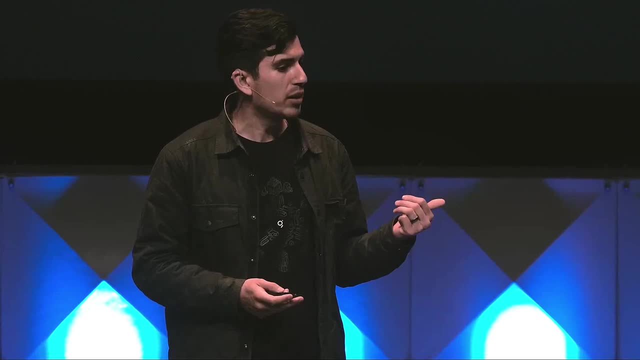 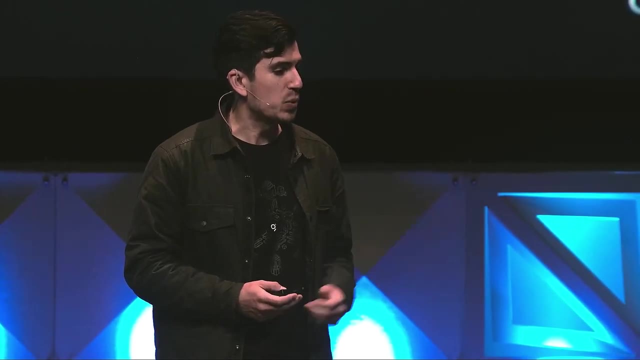 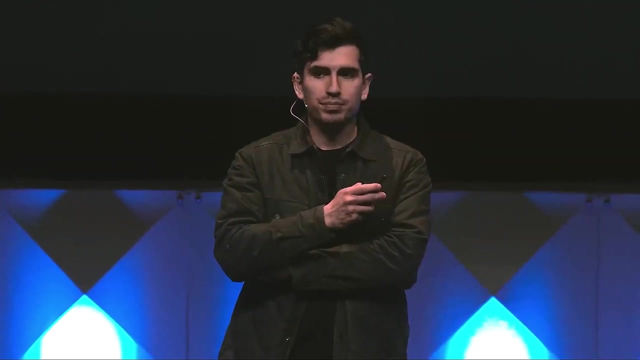 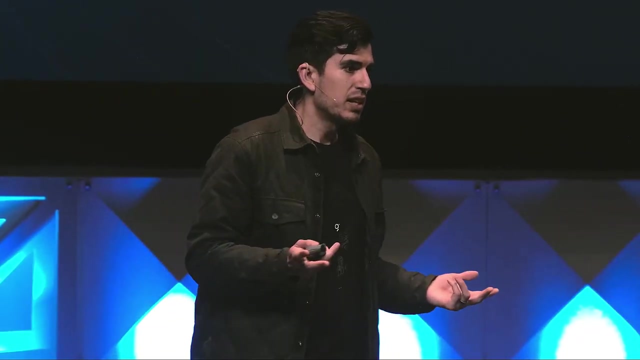 brand-new tools for indexers, one called automated Agora and the other that's an allocation optimization tool- And those will be available in beta to try out at GraphHack this weekend. The other benefit to having these agents, beyond just making the lives of our users better, is that 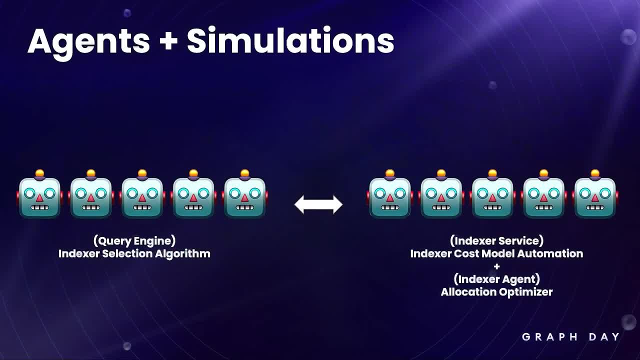 now we can actually run these agents in simulations called agent-based models. So this is a technique from computational social science where we can basically take all these bots, put them in different scenarios and see what are the emergent properties that come out of that related to cost. 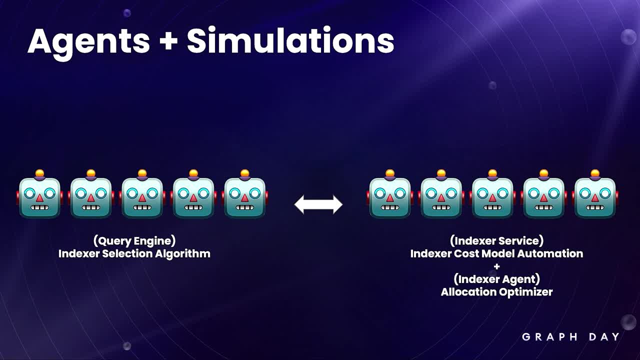 of service or quality of service. We can do that by both tweaking the behaviors of the agents, but we can also tweak the rules of the system. So we can do that by both tweaking the behaviors of the agents, but we can also tweak the rules of the protocol and see how the existing agents 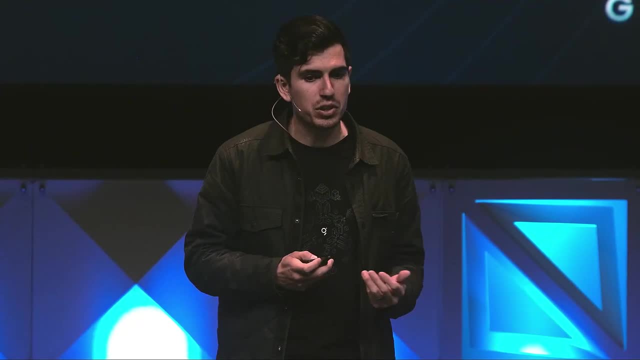 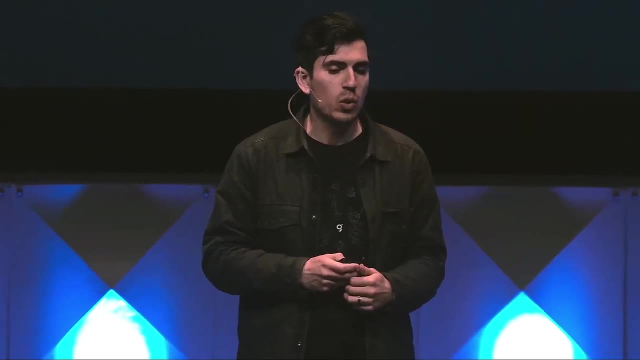 lead to a different outcome for quality of service, And we have a number of improvements that are sort of on the backlog that we think are going to continue pushing the boundaries on quality of service and cost of service that we're going to validate in this way. 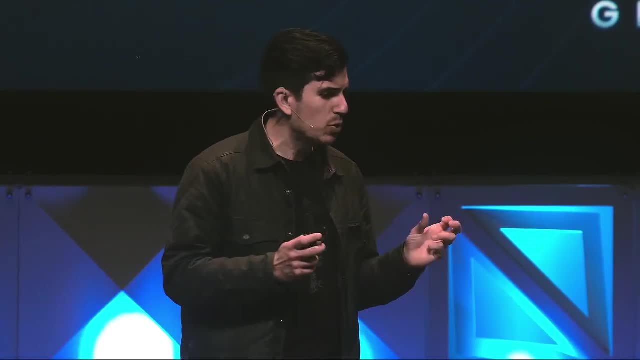 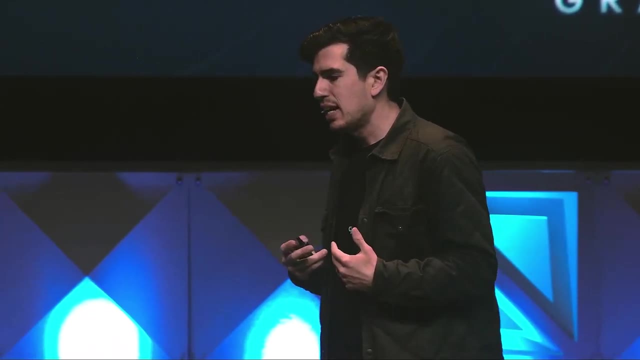 Now, when it comes to using agents as a consumer, maybe the indexers can handle it, but most consumers? this is kind of a new pattern, right? We're not used to having robots that can handle it. We're not used to having robots that can handle it. 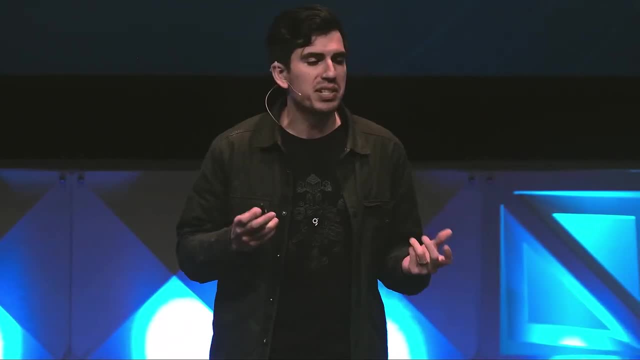 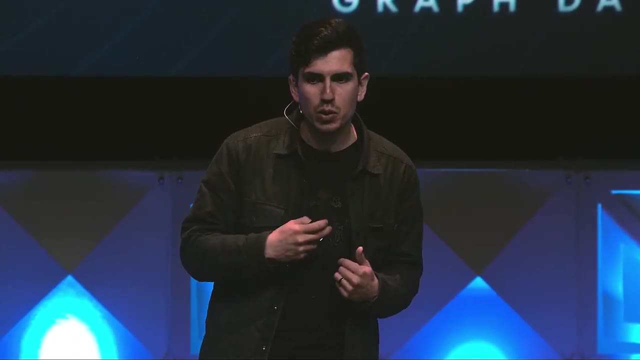 Robots make decisions on our behalf. In fact, quite the opposite. We're used to technology giving us information that we can then use to make decisions, But here we're flipping the script. Here we need a way of representing what users want, so that agents can make automated decisions. 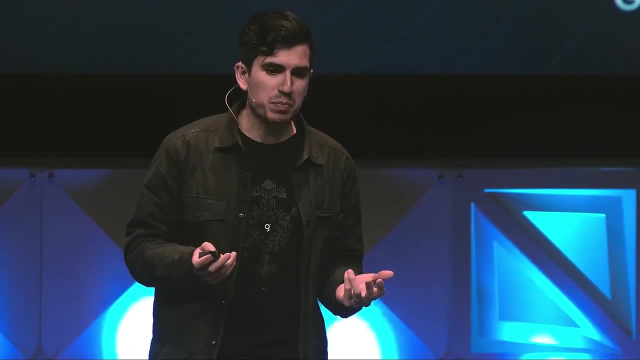 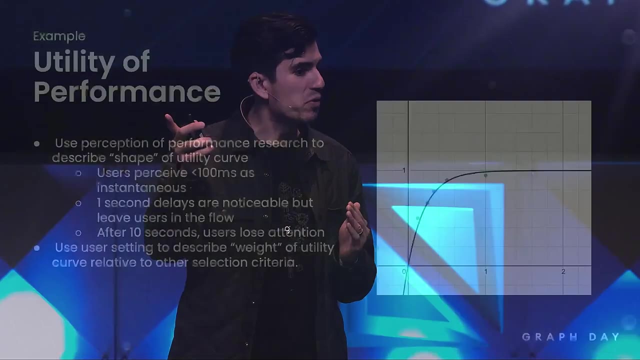 on their behalf. One way we did this with respect to performance was we looked at cognitive research to figure out where the points of diminishing returns were for responsiveness. So you can imagine that, let's say, 50% of the agents that we're using they're not using the same. 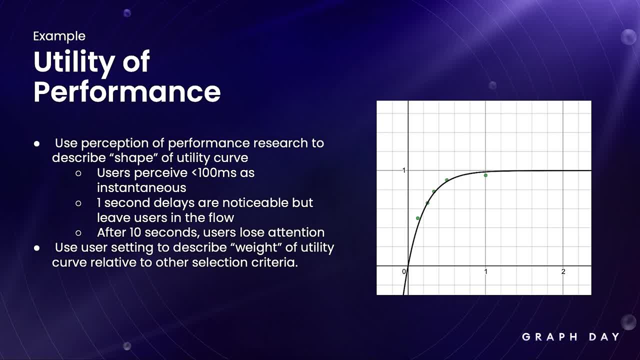 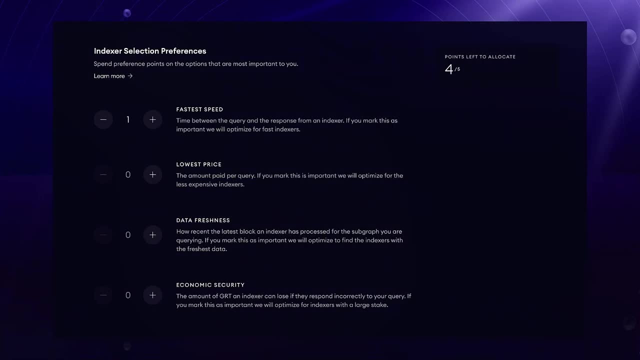 results. We're doing the same observations, but we're trying to figure out where they're at: the output, the API, the responsibility, the performance, and we're doing this all these different things over and over, And then we put all this together to make the. 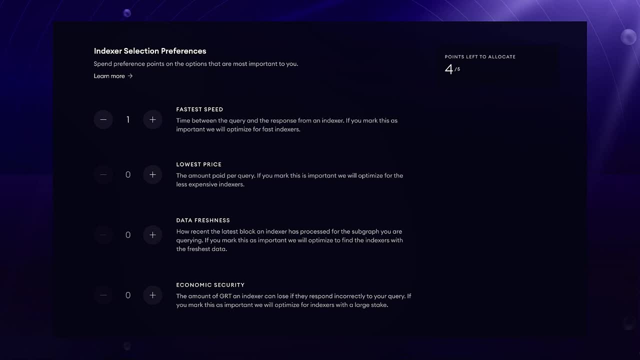 very, very basic 태p story. So you can see the cost of service performance, cost of service data freshness, how much these things mean to them. So this is a screen capture. So this is where we're going to look at how our stakeholders, users and people that are 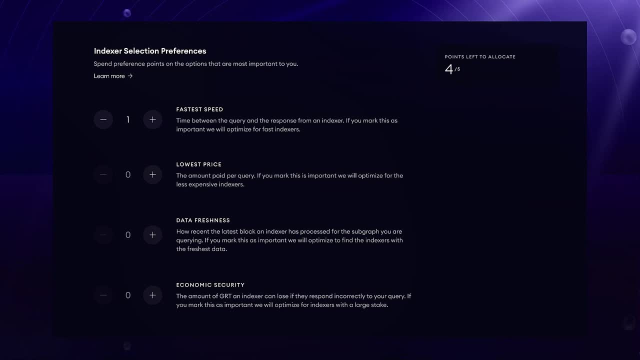 using the right tools, how they're using the data, freshness, how they're using it, And shot from the subgraph studio, where the subgraph developer can modify an API key to decide which of these things they want to value. And then, into that experience, we're building reporting. 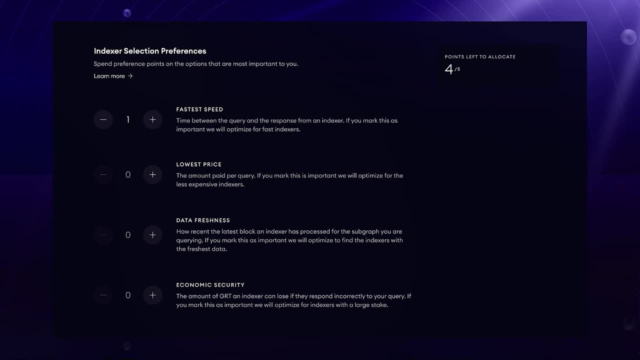 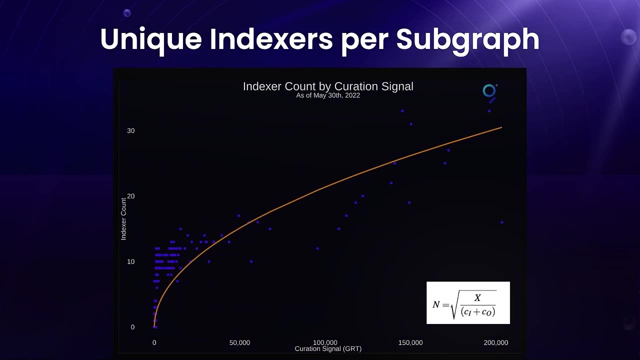 tools and predictive analytics to help them understand what is the experience that they're going to get when using the decentralized network that's going to give them the quality of service that they expect. Another big driver of performance is just the number of indexers on a subgraph. As you might imagine, more indexers on a subgraph means there's more likely to be a 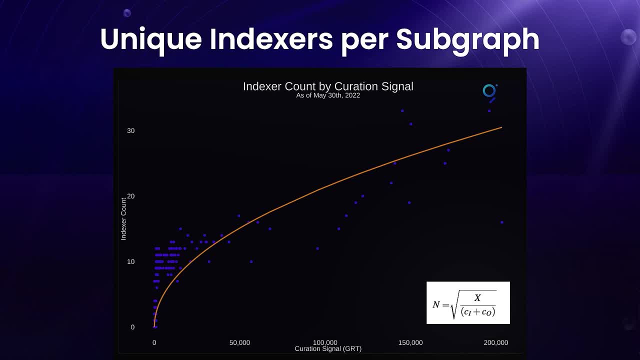 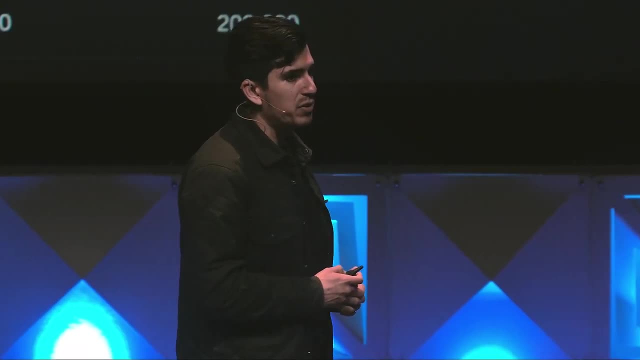 high-quality indexer with good uptime, the data freshness you need and the geography that you want, And so another big portion of our focus has been on how do we drive the number of indexers on a subgraph up. Interestingly, a grant from the Graph Foundation to the economic auditing firm. 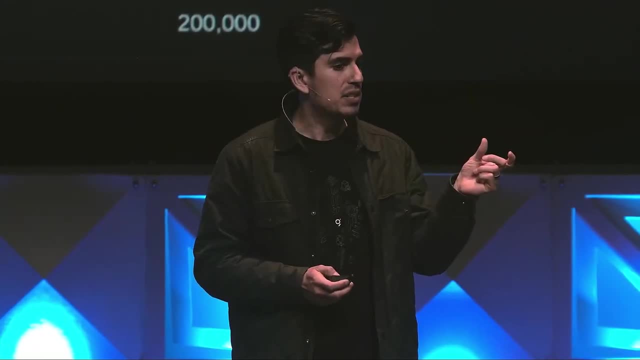 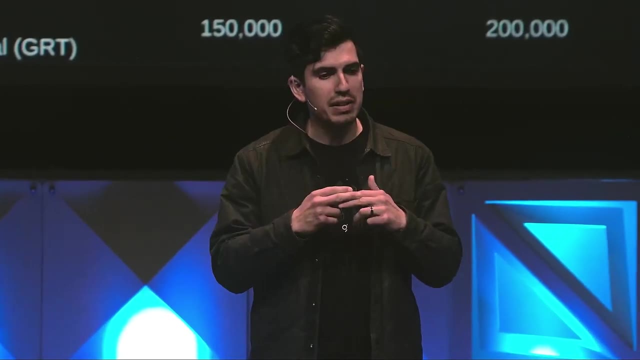 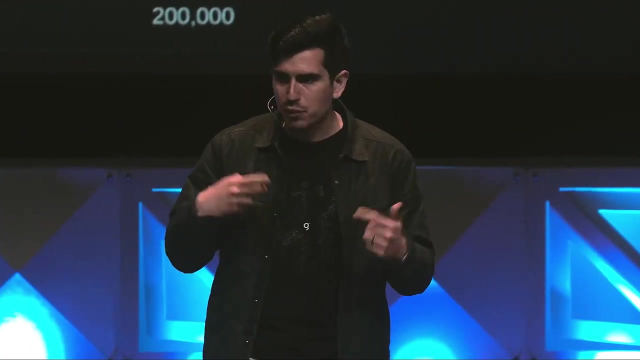 Prism Group included equilibrium analysis That related the number of indexers on a subgraph to indexing rewards, basically the square root of indexing rewards over the fixed costs of servicing that subgraph. And so there's this inverse relationship between the fixed costs that indexers have to pay to service a subgraph. 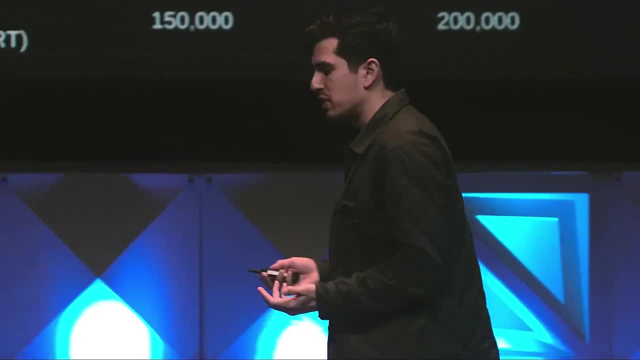 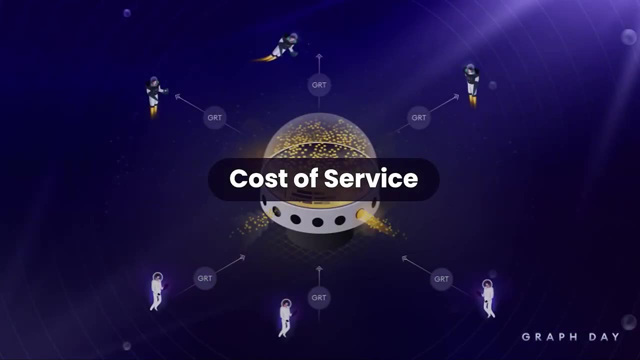 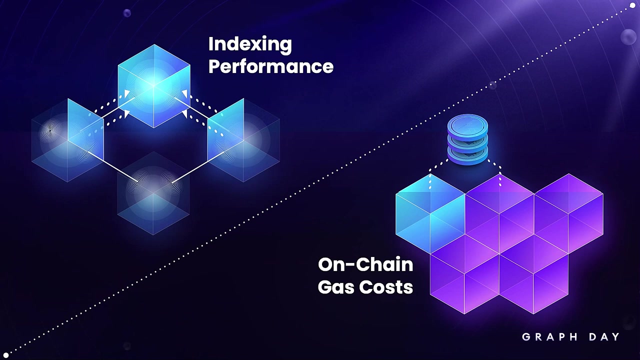 and the number of indexers we'd expect to service a given subgraph. And that brings me to the next section, the next pillar of success, which is cost of service. Cost of service in the graph today has two main components. One is indexing performance, which I'm 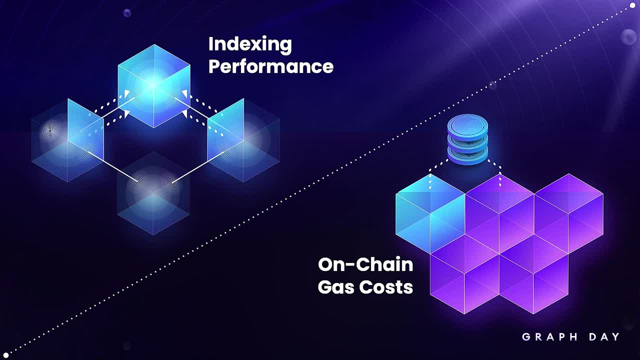 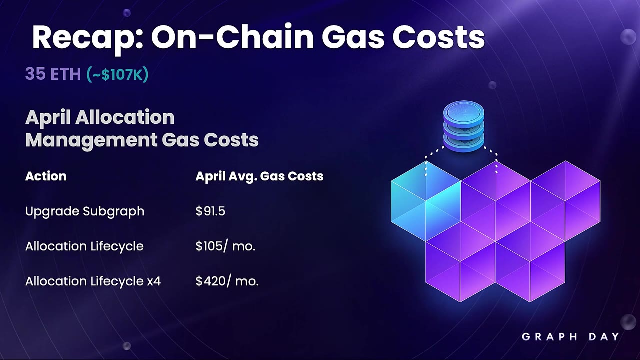 not going to spend a ton of time on in this talk because there's going to be a great talk by Sebastian later today. as we mentioned that, I highly encourage you to stick around. for The other big driver of cost is on-chain gas costs. To give you a recap of where we're at today in the network, to upgrade a subgraph, these are April averages. 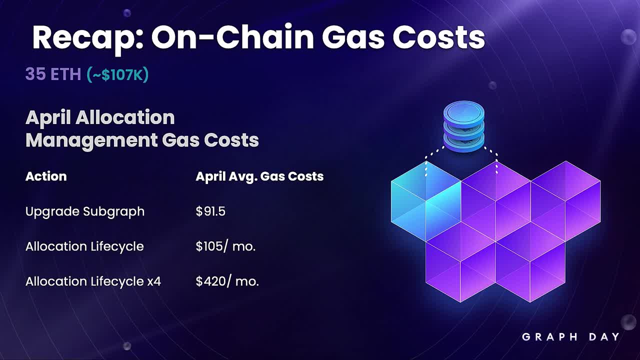 Costs about $100.. So if you're a subgraph developer- let's say upgrading your subgraph a couple times a month, that's close to $200.. And then the cost- the gas cost- that an indexer has to pay to service that subgraph for about a month- is upwards of $100.. And as we just talked about more subgraphs, excuse me, more indexers on a subgraph is better than less indexers. So if we say four is the magic number, well, now we're up to $420 a month, And so, if you're keeping count, we're at $600 total for a subgraph upgrading twice a month. and that's all just gas, right. 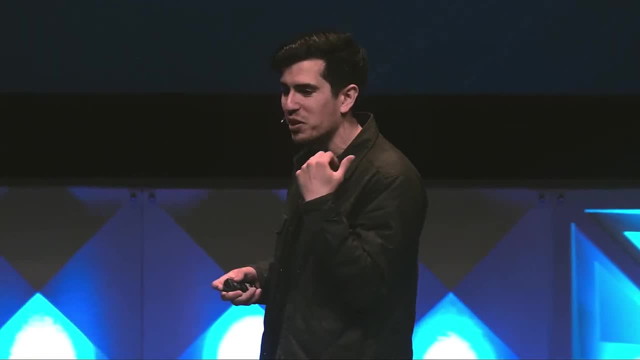 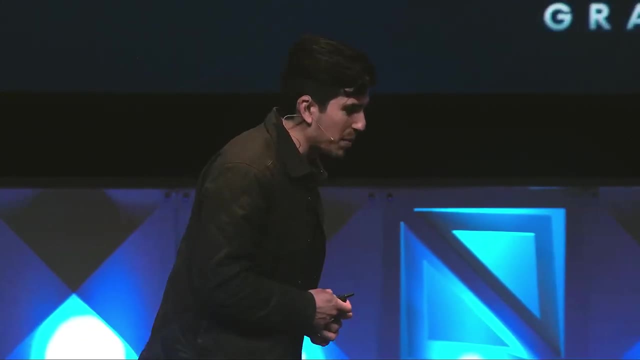 That's not value. that's going to the bottom line of indexers. That's not value that's going into quality of service or DevOps infrastructure. That's just gas, And so it should come as no surprise that the answer here is Layer 2 scaling. 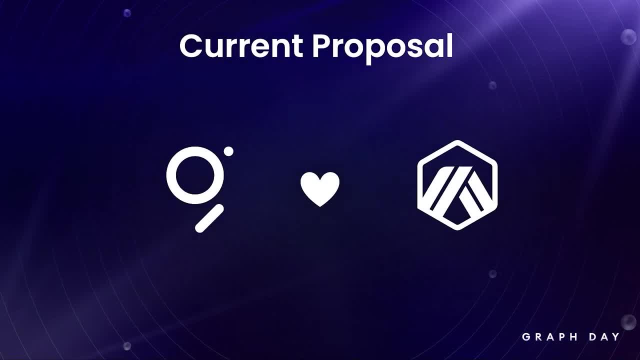 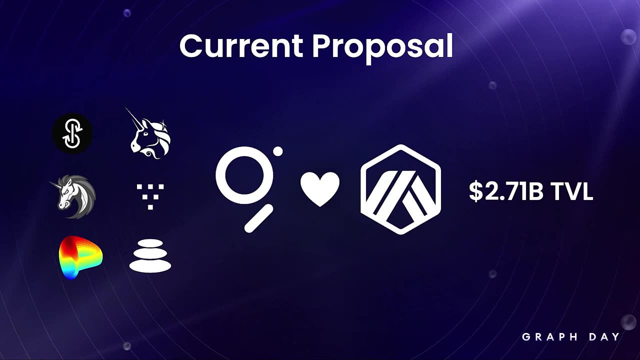 And today I'm excited to announce that the graph is planning on migrating its smart contracts to Arbitrum 1.. We feel that at this stage in the game, Arbitrum 1 has proven itself. It's been battle tested. It has several billion dollars in total value locked. 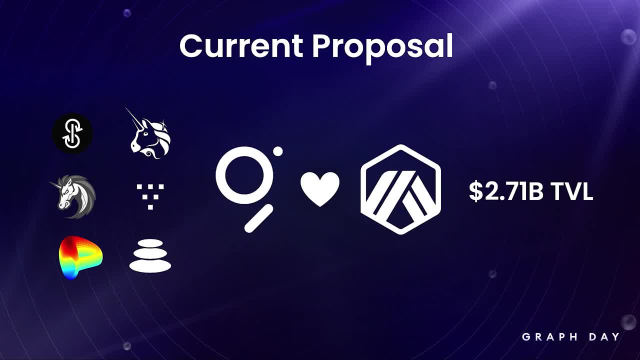 It has prominent projects that have migrated to it, including projects like Livepeer that have very similar requirements and economic considerations. as the graph To give you a sense of the impact that this has had on the market, Arbitrum 1 is a very similar project to Arbitrum 1.. 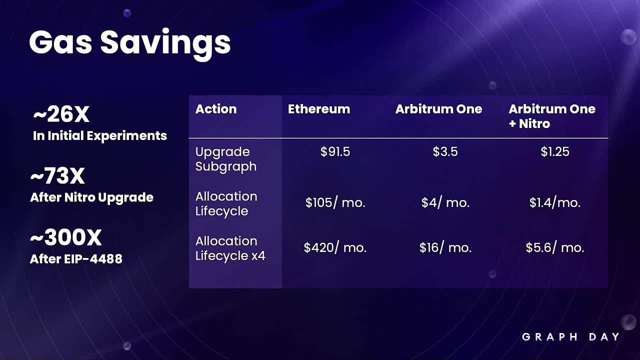 This is going to have on the network. In our initial experiments with Arbitrum we saw about a 26X improvement in gas costs. With the planned Nitro upgrade that Arbitrum has, that's going to both start adding support for WASM but also introduces a smarter compression techniques. 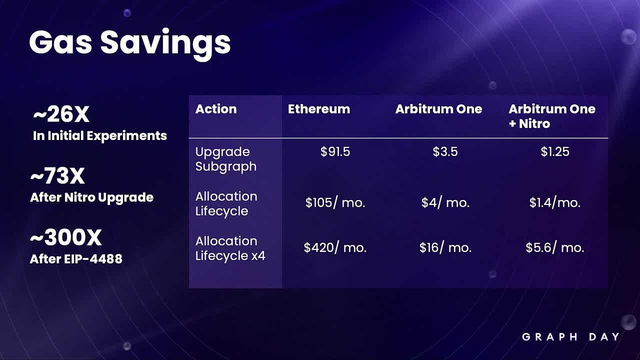 We predict that those gas savings will bump up to 73X and if EIP 4488 passes, Kristobal Ernia parte. distributor de entublik decyatación en el mercado 스�í certificación de gastos de gastos. of call data on Ethereum, we could see those improvements go upwards of 300x. Now what this means for end users is that upgrading the subgraph could go from $90 on chain today to $1.25, and the cost of four indexers servicing a subgraph for a month. would go from $420 to about $5.. And what that means is using the graph as decentralized network is going to suddenly become a viable strategy for a huge long tail of independent subgraphs that were maybe too small or priced out of the network as it exists today. 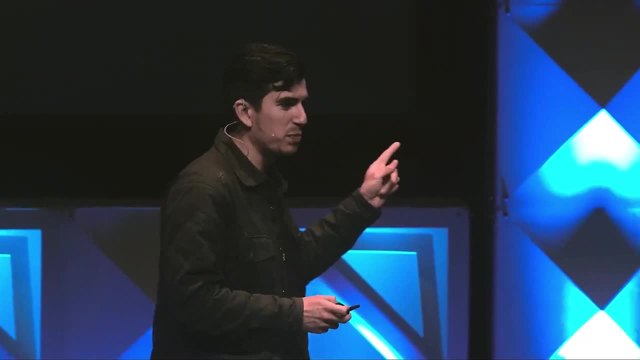 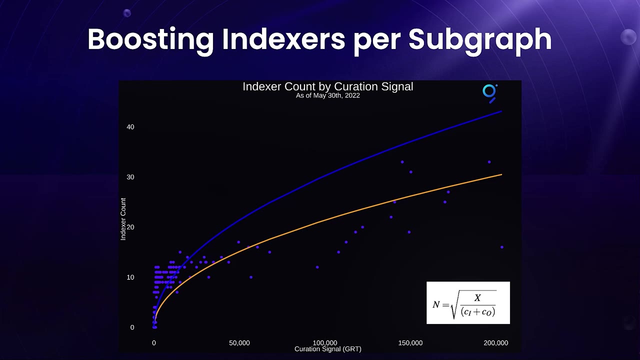 The other effect that this is going to have, tying back to the quality of service pillar earlier, is that, if you recall, We had the cost of servicing the subgraph in the denominator. Now we expect an upward shift in the number of indexers per subgraph and we expect this. 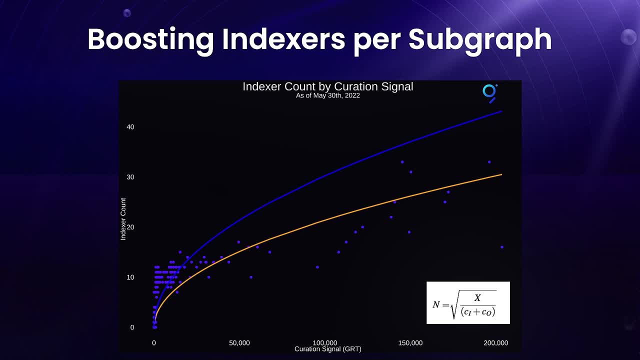 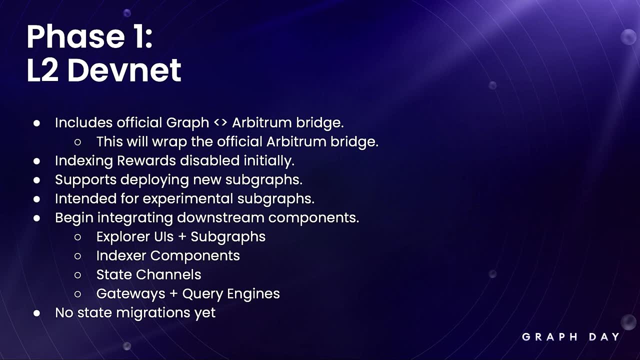 to continue driving quality of service even beyond where we're at today. This is going to be split into several phases. The first phase of this is what we're calling an L2 DevNet. This is going to include an official graph to Arbitrum Bridge wrapping the native Arbitrum. 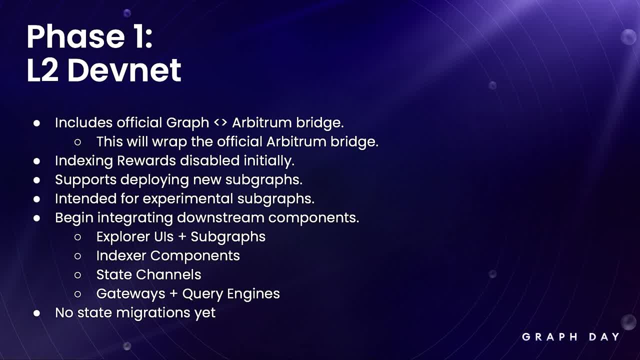 Bridge. Initially it's going to have indexing rewards disabled and the intent is for this to be a place to put experimental subgraphs and altruistic indexer allocations, And the main purpose here is for us to get comfortable with the Arbitrum model and also. 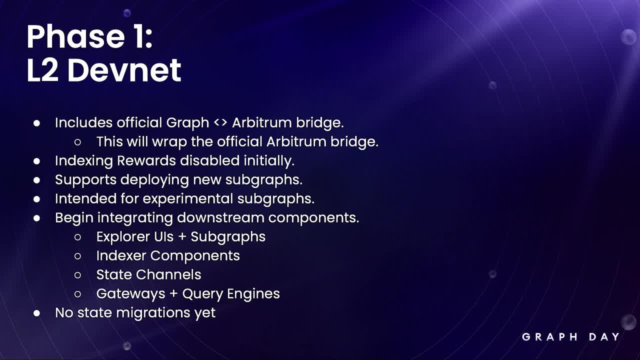 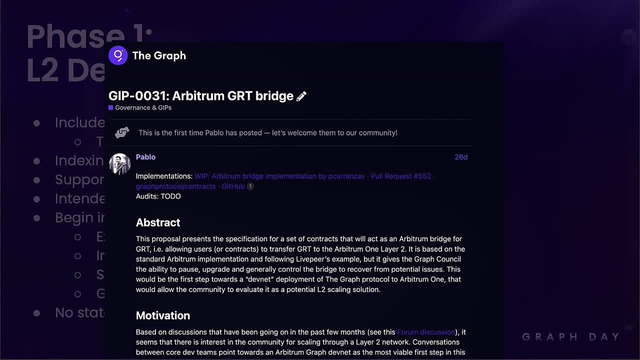 give the various downstream components a place to start integrating, And I highly encourage you to check out the forumcom as well as the GIPs that are hosted on Radical. This is the first of seven. There are several GIPs that are going to be published to explain what that Layer 2 rollout. 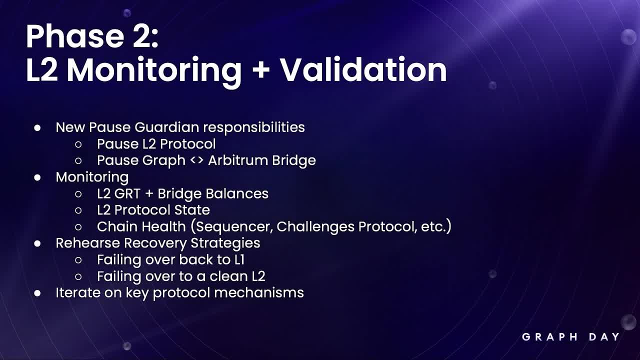 looks like The next phase is monitoring and validation. It feels like every week we wake up to another multi-hundred-of-millions-of-dollars bridge hack and we take the security of the protocol extremely seriously, as well as the fact that 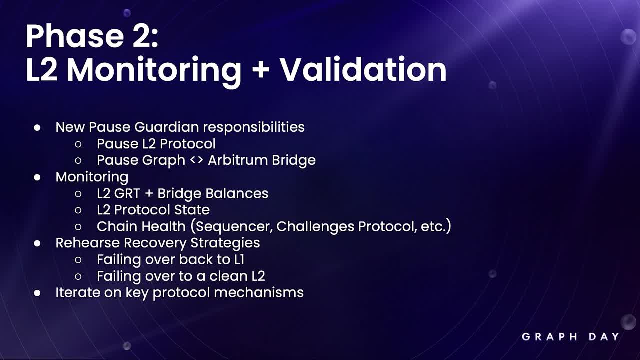 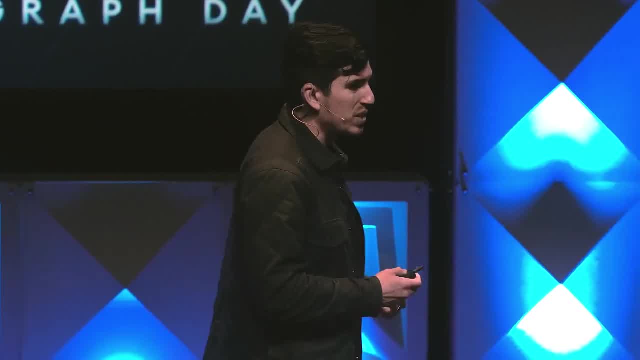 the graph is mission-critical infrastructure for dApps that are running in production. So in this next phase we'll be rolling out new capabilities for the PaaS guardians and the protocol. We'll be setting up new monitoring infrastructure to make sure that the state of the bridge. 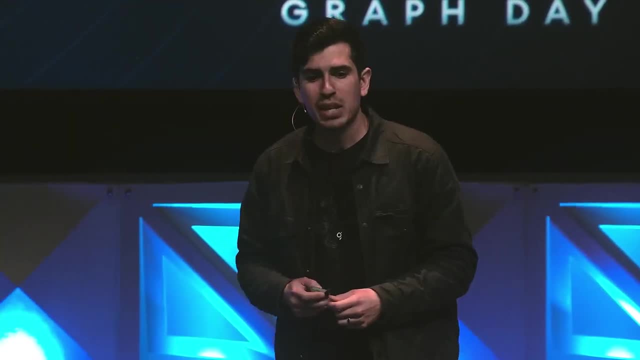 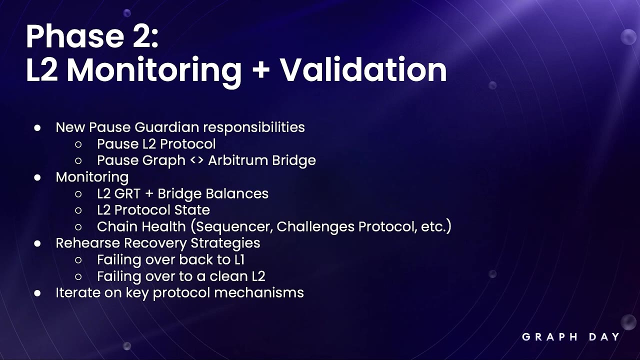 as well as the state of token. balances on L2 are consistent And we're going to be rehearsing recovery strategies as an ecosystem, building a better understanding of what it feels like to failover back to Layer 1 or to a fresh Layer 2 in. 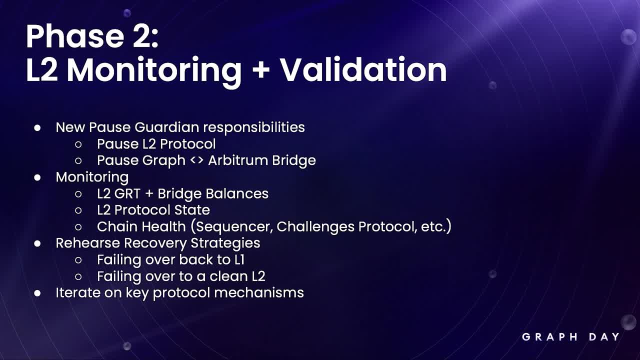 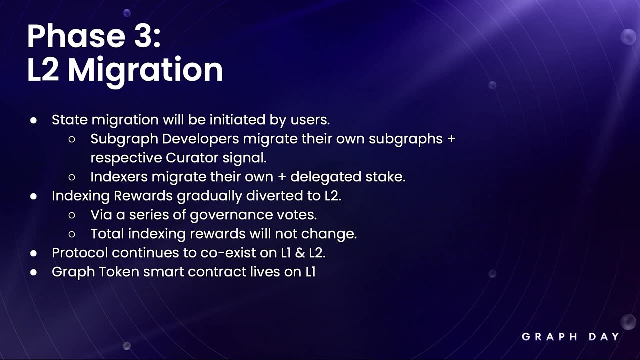 the case of a catastrophic L2 failure, And this is also an opportunity for us to iterate on key protocol mechanisms that will benefit user experience, which we'll get to in a little bit. The next phase is migrating subgraphs from Layer 1 to Layer 2, or, as may be the case, 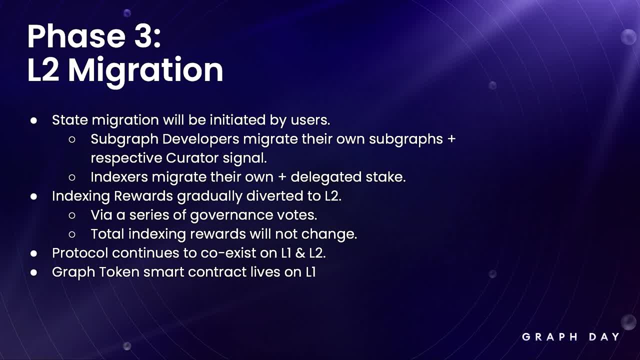 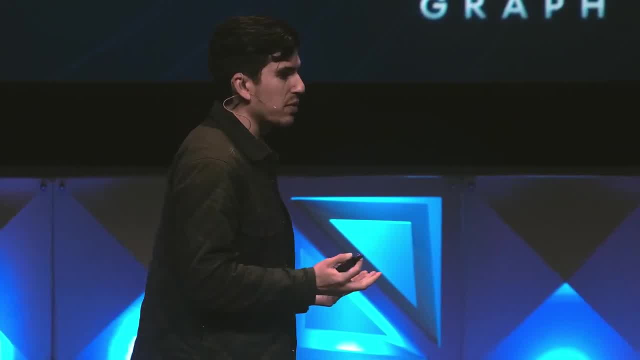 migrating subgraphs directly from edge-to-nose hosted service to Layer 2.. Importantly, state migration will be incremental and it will be initiated by key users, So subgraph developers will be able to migrate over their own subgraphs as well as the curation. 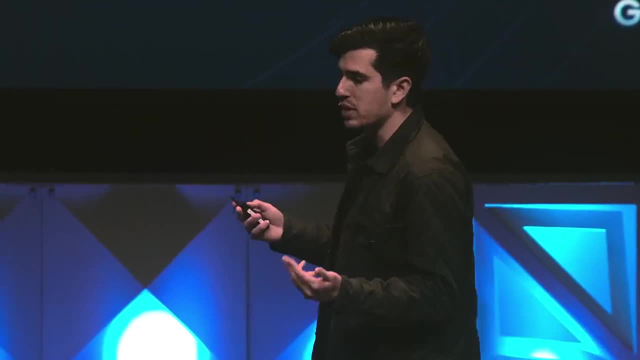 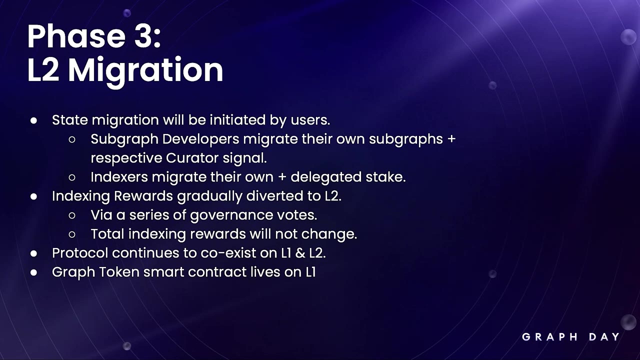 that's been received on those subgraphs and indexers will be able to migrate their own stake And that's almost the stake that's been delegated to them And at this point in time in the core developer ecosystem there's no intention whatsoever. 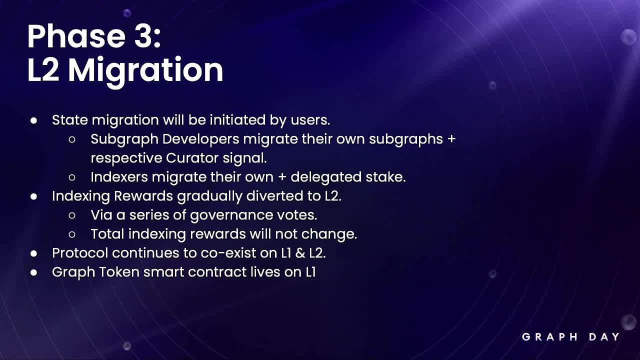 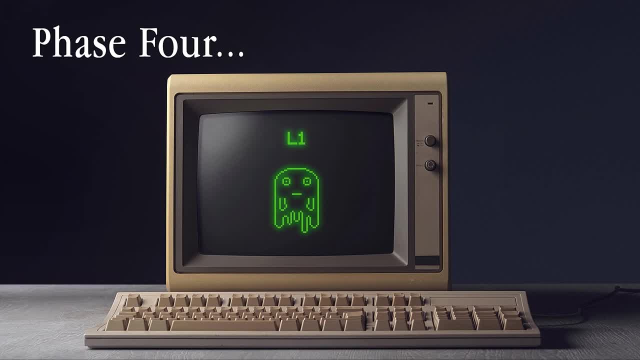 of moving the graph token anywhere other than where it exists today on Layer 1.. And phase 4, we hope is that over time, L1 just becomes a ghost town. It'll continue to be there if we need it, but we fully expect that as the assumptions. 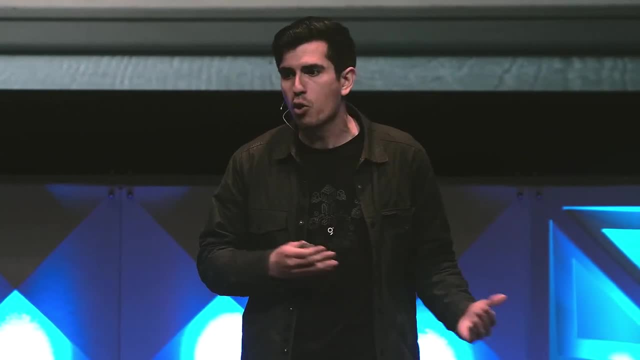 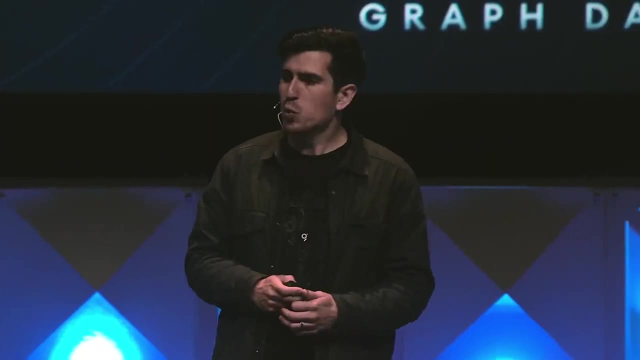 around Layer 2 and people get comfortable with it from a user perspective, that all graph usage will change. We'll just move to arbitrage from Layer 2.. To give you a quick idea of the estimated timeline, noting that it's always hard to make estimates in a decentralized, open source environment. we expect L2 DevNet to launch by the end of Q3.. In Q4, we expect to complete monitoring and validation and we expect to begin migration of subgraphs from Layer 1 to Layer 2 by the end of the year. 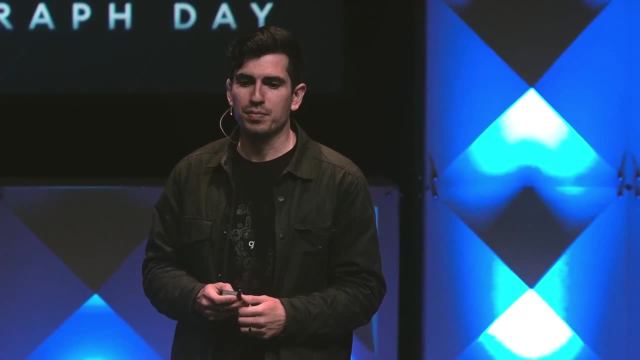 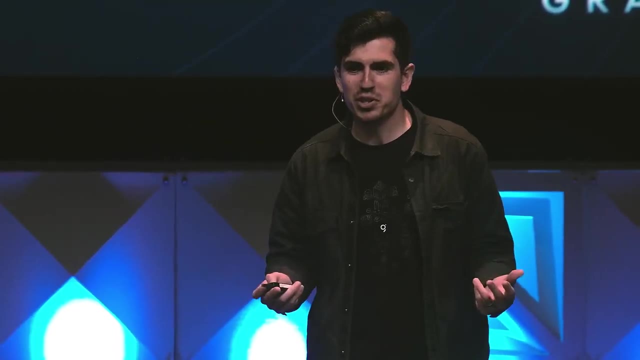 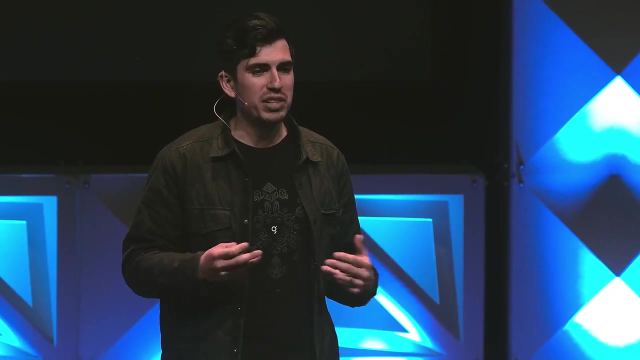 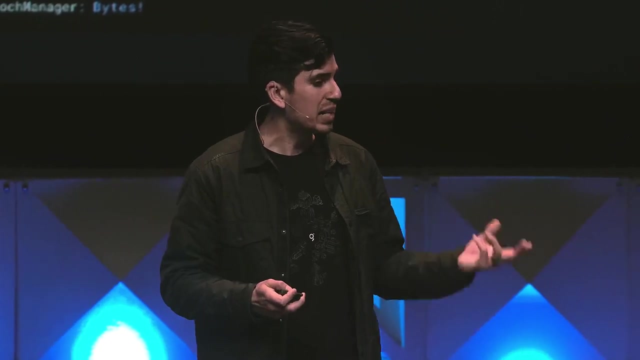 So let's talk about user experience, And when I say user experience, what I really mean is developer experience, And for us, developer experience really starts with the subgraph studio, where we do things like give you subgraph developers tools for API key management, the preferences that 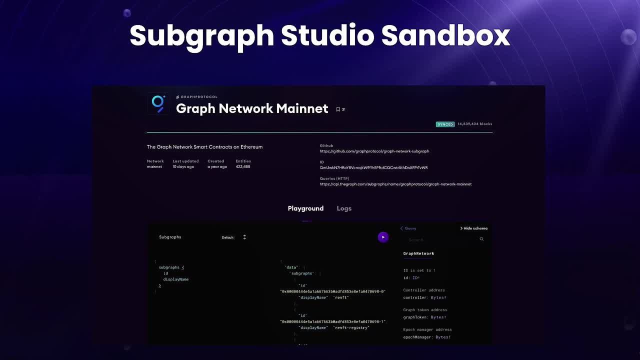 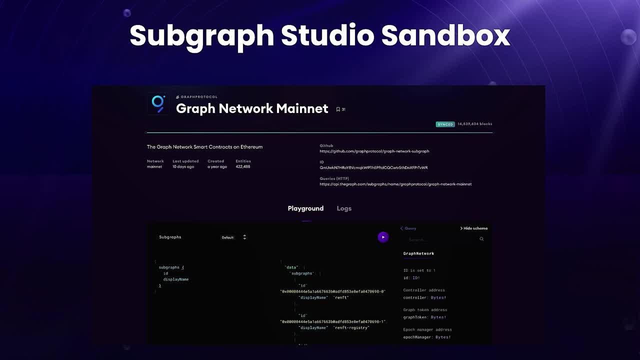 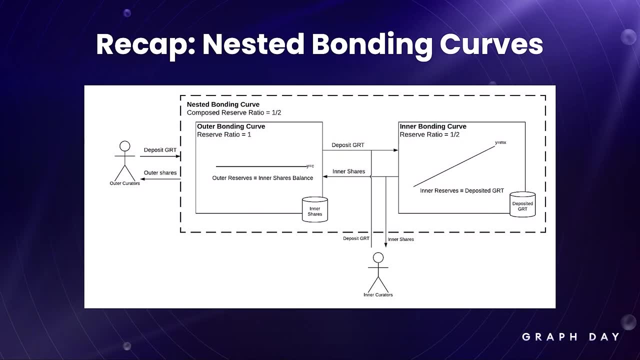 But there's limits to what we can do just on the front end with developer experience. At a certain point we're constrained by the economics, And let me give you a few examples of that. One is the way that bonding curves are used to deploy subgraphs in the protocol today. 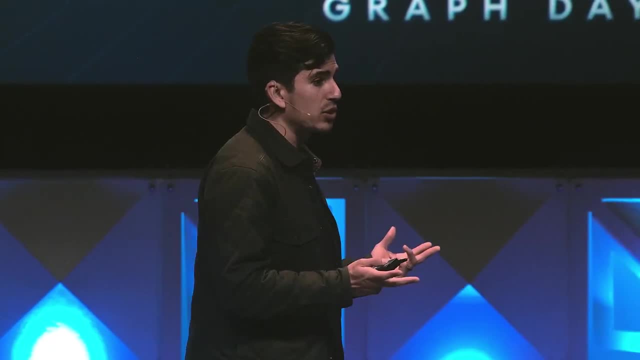 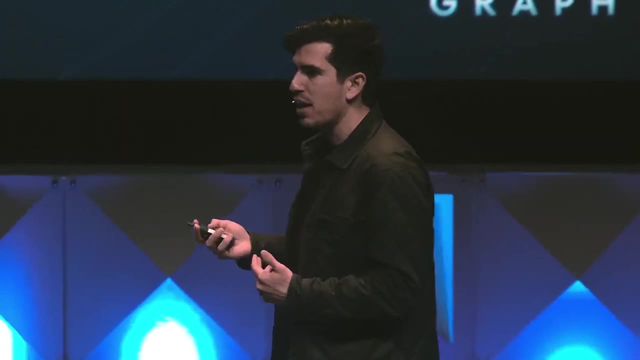 You heard a little bit about the curation market. It's not as widely known that our curation market uses a two-layer. It's not as widely known that our curation market uses a two-layer nested bonding- curve construction. When users want to deploy or upgrade subgraphs, they're interacting with one or more bonding. 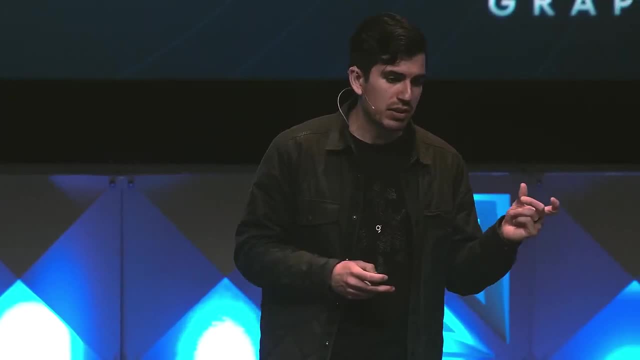 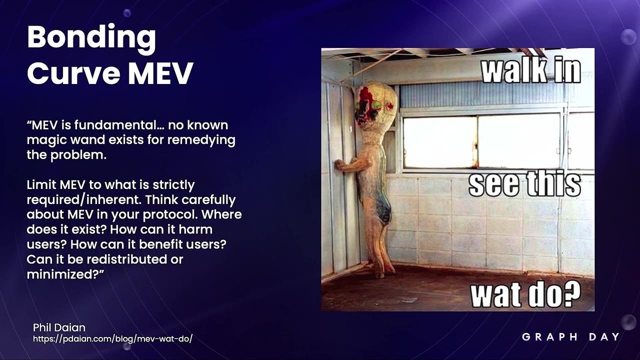 curves And we've seen a lot of the issues you might expect with things like price slippage and also MEV. Prominent MEV researchers today basically say that some level of MEV- which is either minor or maximal extracted value, depending on who you ask- is inevitable. 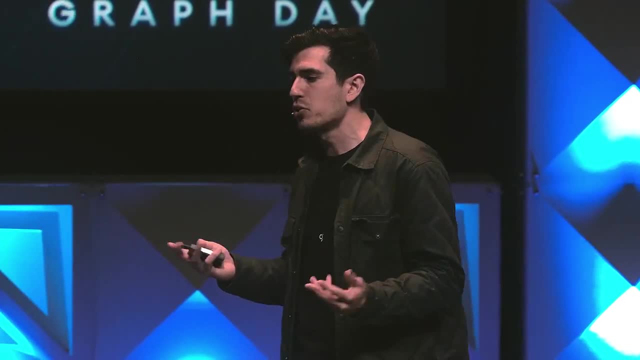 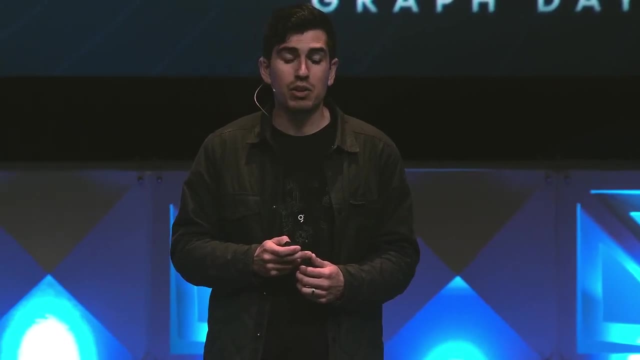 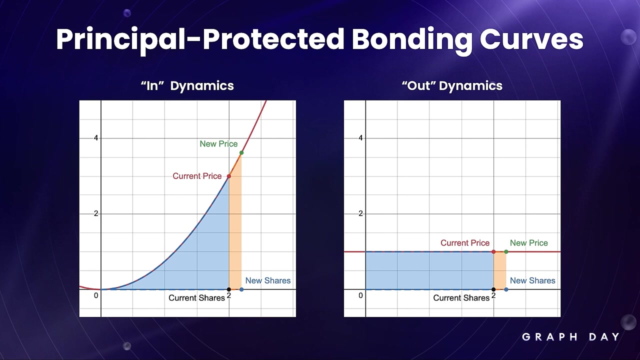 And it's really up to us as protocol and application designers to figure out ways to mitigate MEV at the protocol layer. So on this front we actually have an exciting announcement- Well, exciting if you're a wonkish protocol economics type that we call principle-protected. 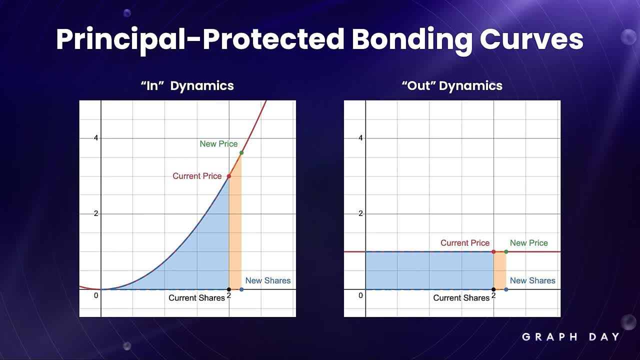 bonding curves And without getting too much into the weeds. these are MEV-proof bonding curves that preserve some of the earlier is better- dynamics of traditional bonding. And these are MEV-proof bonding curves that preserve some of the earlier is better dynamics of traditional bonding. 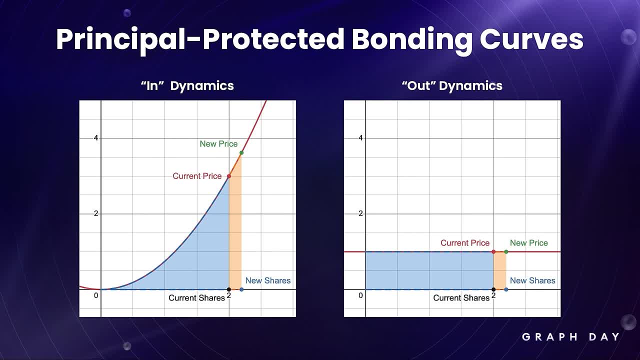 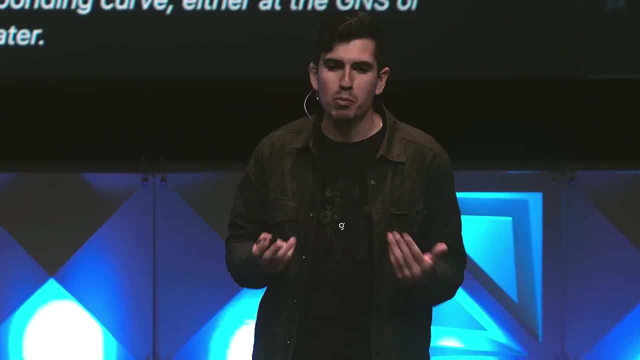 But where the user doesn't incur any principal risk by interacting with the bonding curves. I highly recommend you check out the GIP in the forums if you're interested in learning more. This was a proposal put forward by Juan de Fago from actually one of our new core development. 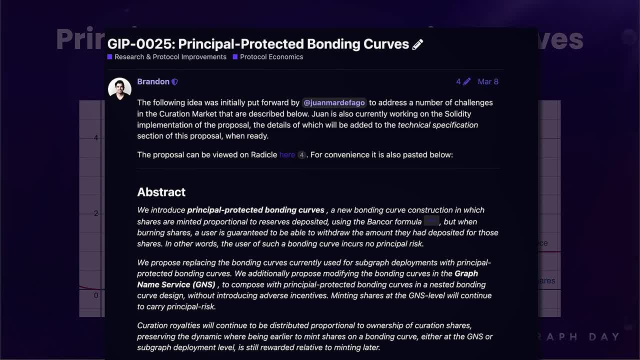 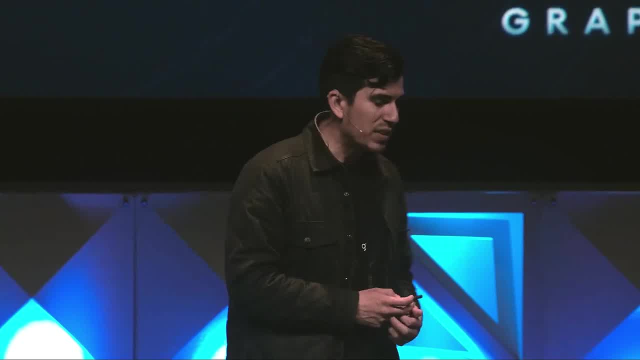 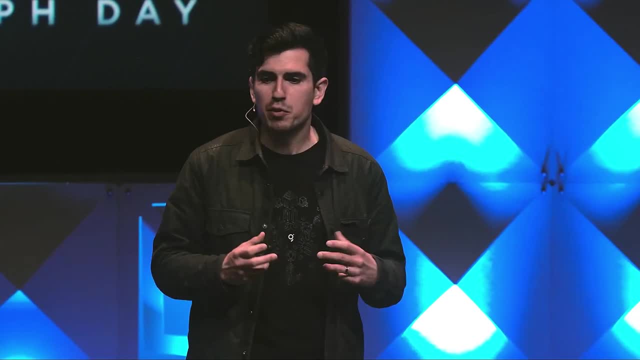 teams announced today at graph ops. One of the other pieces of feedback we hear from subgraph developers is that it's you know. sometimes they have a preference for modularity for performance and upgradability purposes, And when you do that in the decentralized 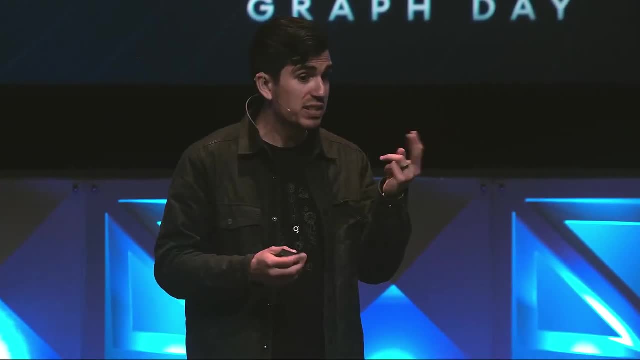 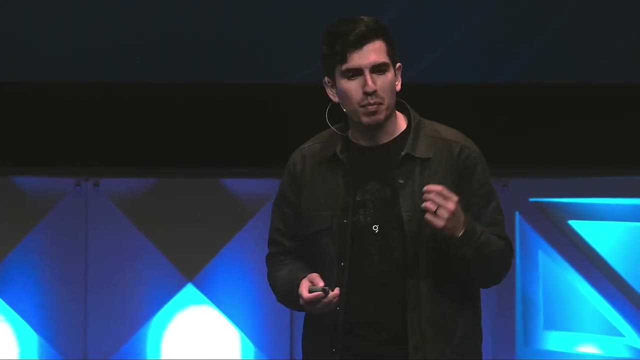 network. that means now you've gone from interacting with two bonding curves to 10 bonding curves, all as a part of your normal development cycle. So part of what will be enabled by things like principal protection as well as L2 gas savings, is more complex mechanisms. 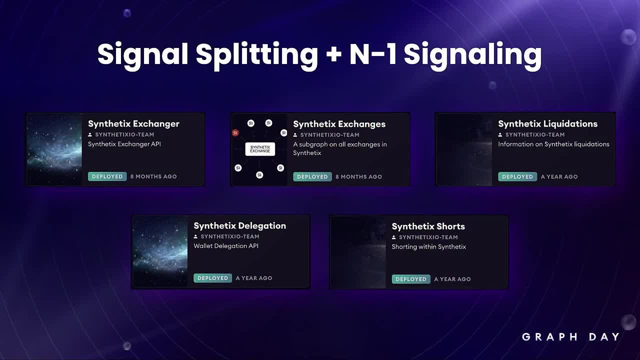 such as signal splitting, which would allow a subgraph developer to interact with one top level bonding curve to manage multiple lower level subgraphs, as well as N minus one signaling, where a subgraph developer could leave some signal on the previous version and the next. 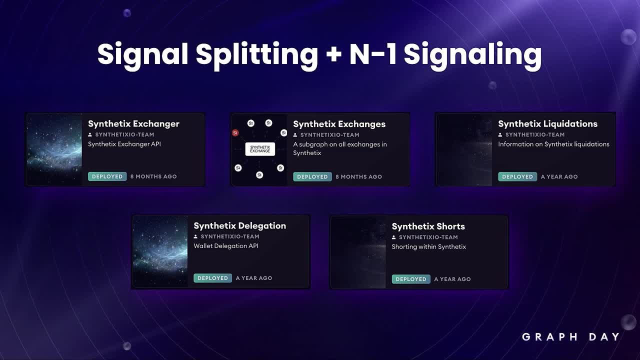 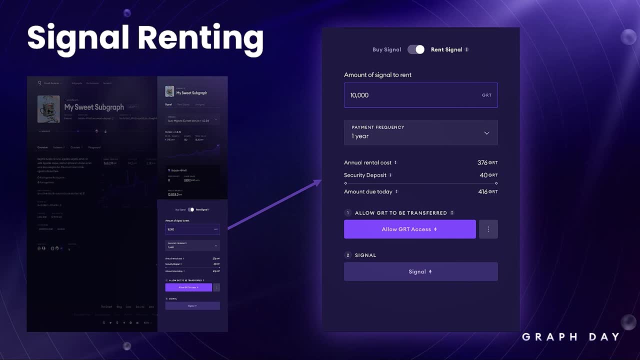 version to avoid any discontinuities in availability for that subgraph. Another really cool mechanism that gets unlocked by both principal protection and L2 gas savings is the ability to use a subgraph to manage multiple lower level subgraphs. L2 gas savings is something that we call signal renting. So one piece of feedback that we've 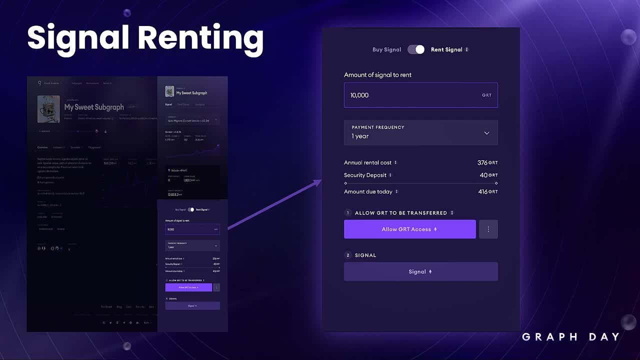 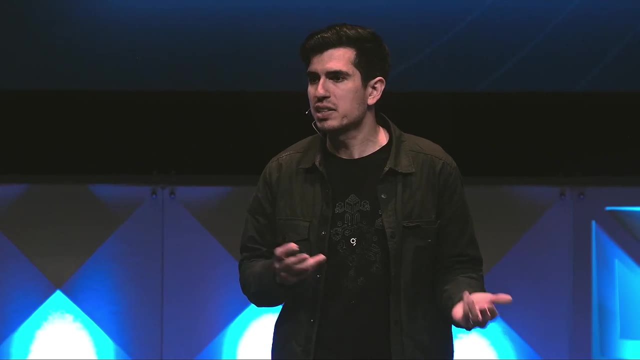 gotten from users today is that having to outlay a bunch of capital by signaling GRT, sometimes in the, you know, in the order of thousands of tokens of GRT, is kind of a unfamiliar and, you know, friction user experience compared to what they might be used to using like a SaaS. 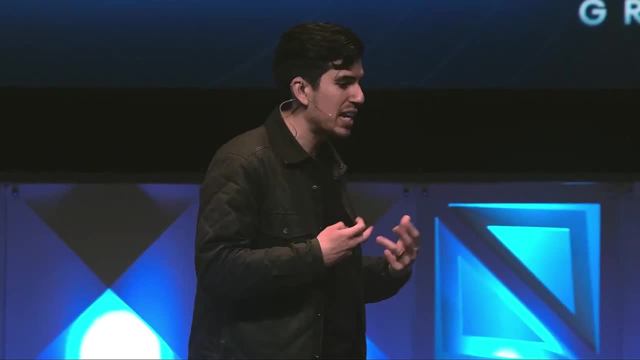 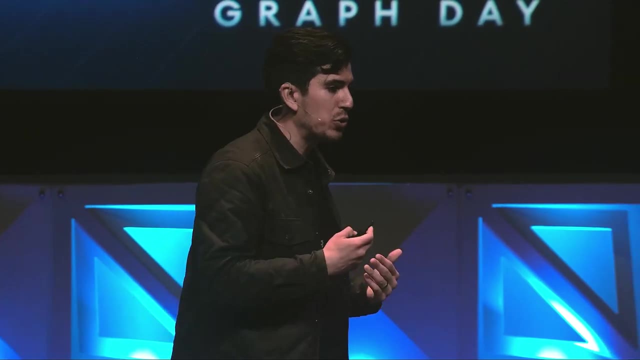 product With principal protection, it's now safe to let subgraph developers rent signal from the other end of the network. So that's a really cool mechanism that we've gotten from some amount of time And with the lower L2 gas costs, it's now cost efficient for them to top. 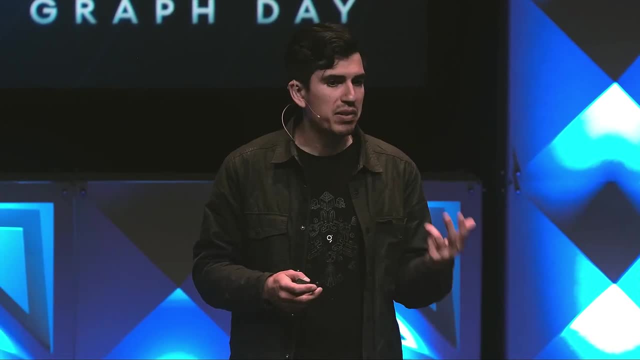 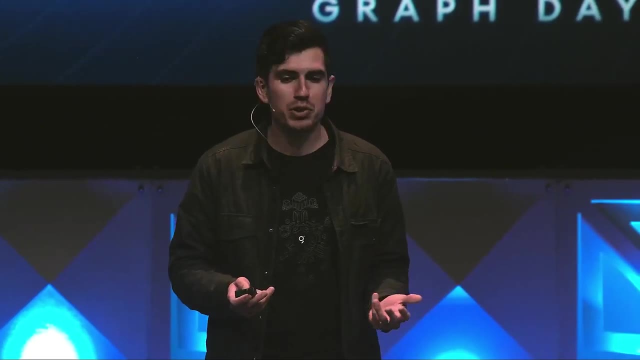 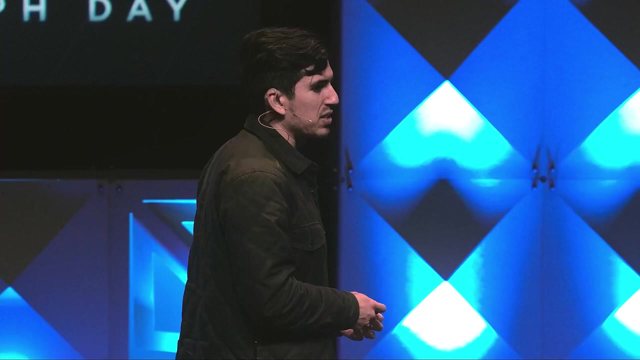 off their subscriptions on a regular basis, whether it's monthly, quarterly, annually, the same way you would expect when using a traditional SaaS or Web2 cloud infrastructure provider. And just to give you an example of you know just the impact that we expect this to have. 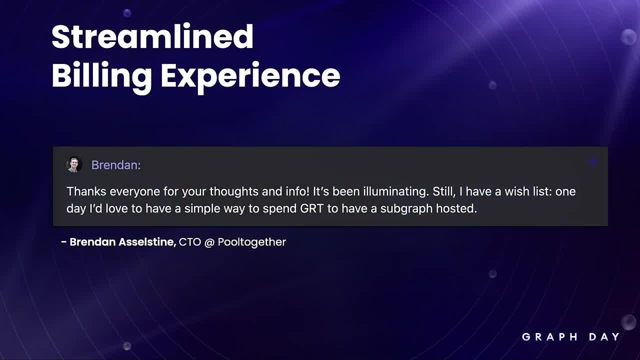 there's a quote from Brandon from PullTogether, the CTO, there, where he's, you know, talking about, you know, his interaction with the curation market and just saying how what he really wants is just the ability to pay GRT to have a subgraph indexed. And with all these changes that I've 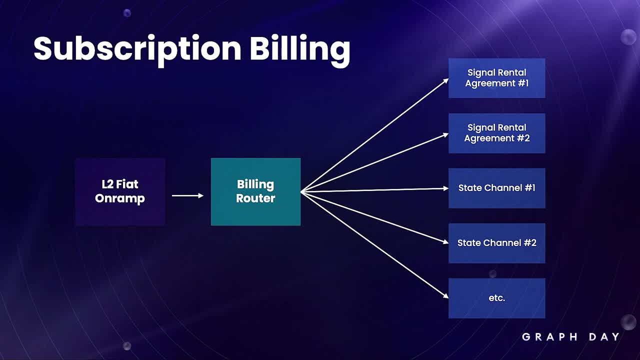 described both signal renting as well as L2 scaling. we'll now have the capacity to have a single on-chain billing router on layer two, where a subgraph developer, for all the subgraphs that they're using, can just pay a single subscription rate, And that's a really cool mechanism. And 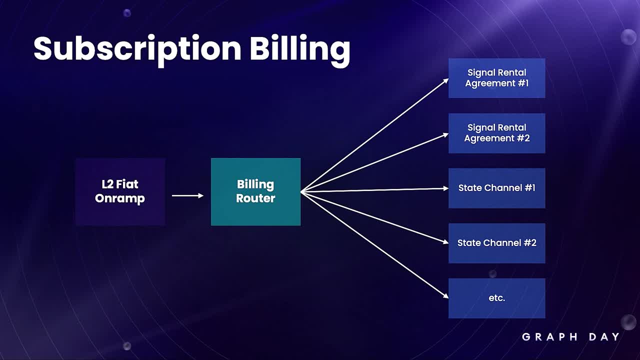 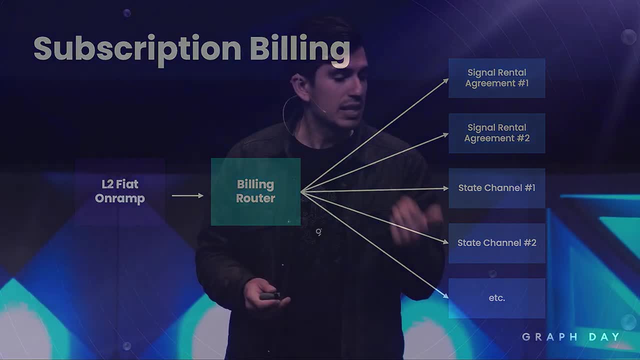 that's a really cool subscription. that's then intelligently routed to all the downstream places in the protocol where a subgraph developer would typically have to interact today, whether that's curating directly, signal renting or managing state channel balances, which, for us today live. 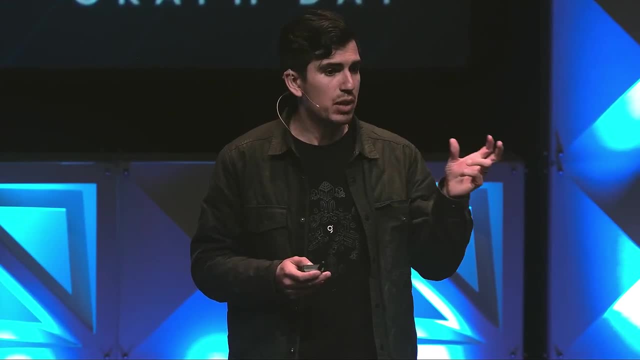 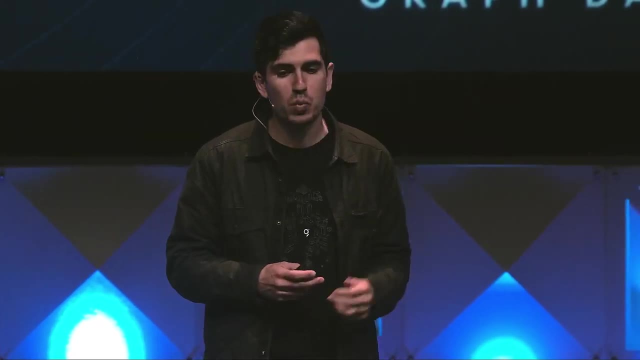 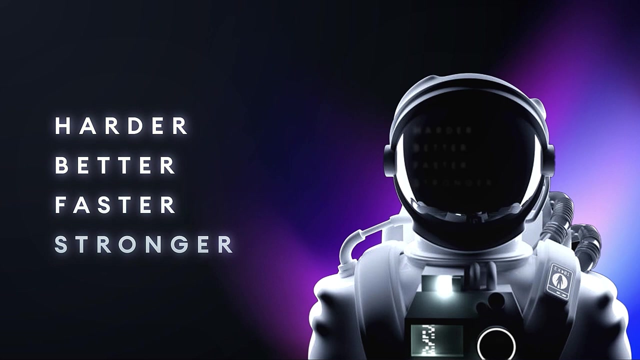 on Polygon. So we think this is going to be a really incredible experience that brings subgraphs to parity with what's. you know the state of the art in Web2 today. So let's put this in the chat. So let's put this all together In the future, based on the research and R&D we've talked about today. 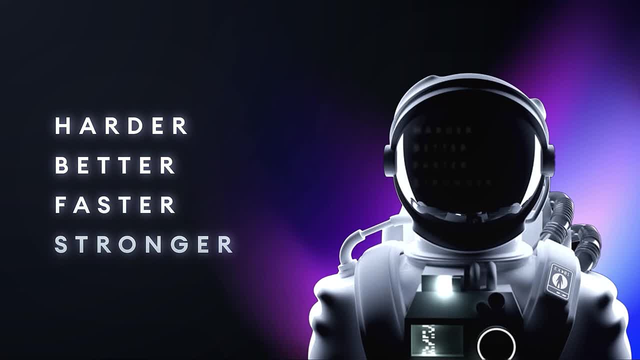 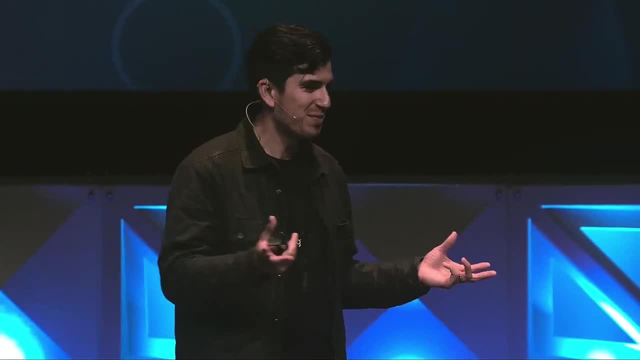 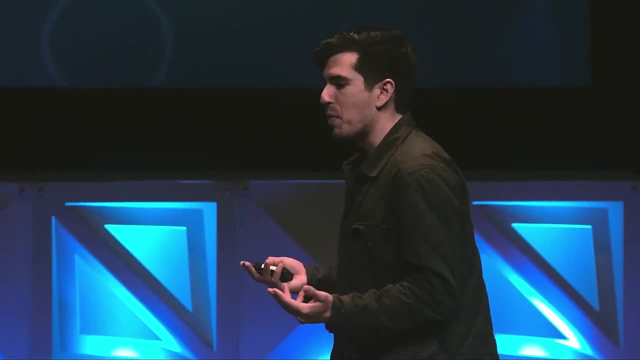 the graph is going to be harder, better, faster, stronger, And by that, of course, I mean we're going to have harder trust guarantees as the graph becomes more and more like a blockchain protocol. We're going to have better developer experience, powered by new economics enabled by layer twos, which is then going to drive. 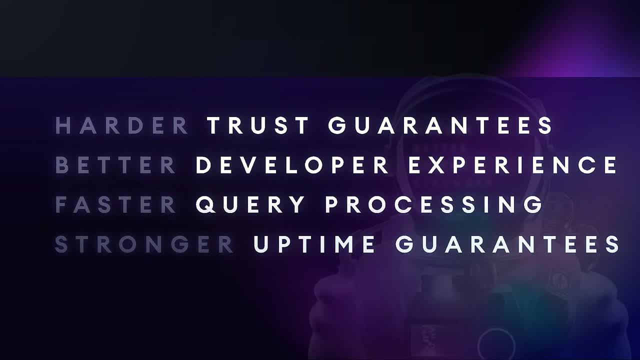 better query processing performance and better uptime guarantees and all around quality of service And I predict that by end of this year, maybe early next year, the graph will have the best quality of service and cost of service of any Web2 or Web3 infrastructure layer without. 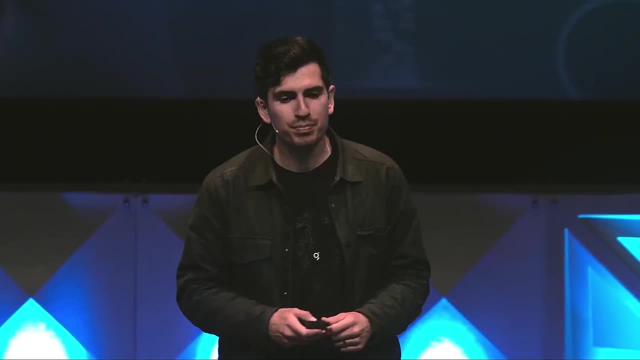 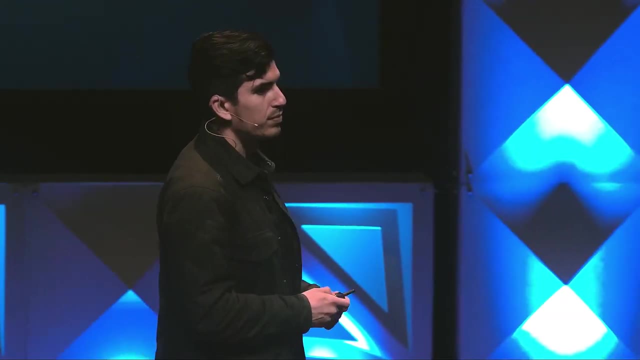 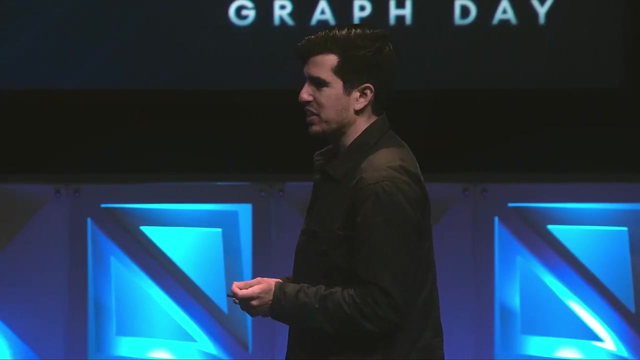 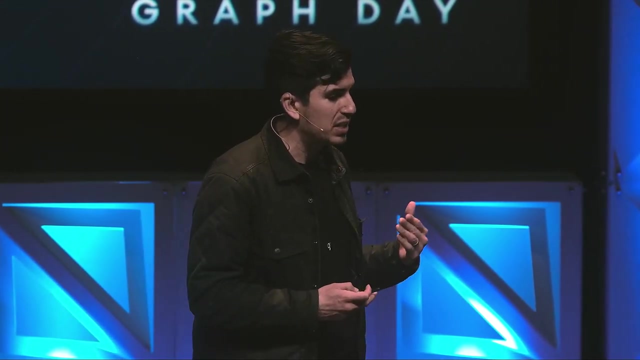 sacrificing any of the benefits of decentralization. And finally, I just want to acknowledge that it's impossible to do justice to all the great work that's happening in this ecosystem in a 50-minute talk. So if you're interested in diving deeper on, 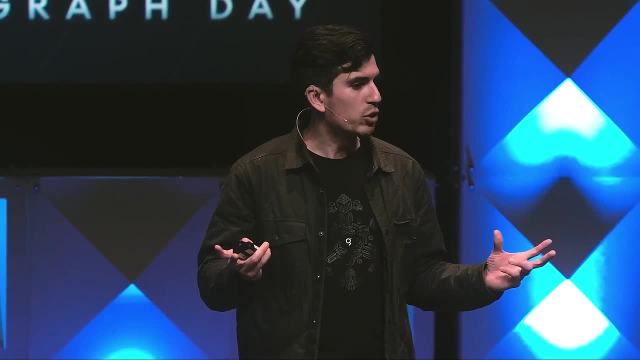 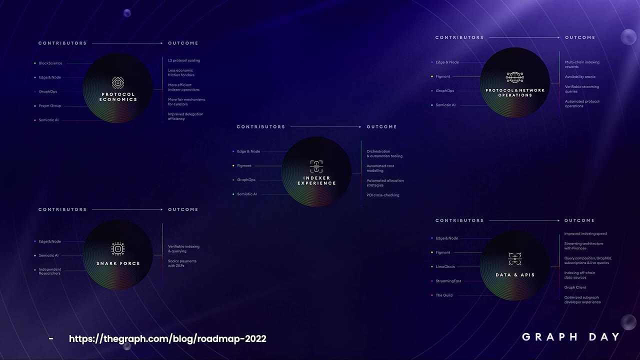 any of these topics. you know we've already heard about the five different working groups today. I highly recommend you checking out the roadmap that was published a few months ago. Hop on the forums, dive into these different GIPs. There's really so much incredible work happening here and we've 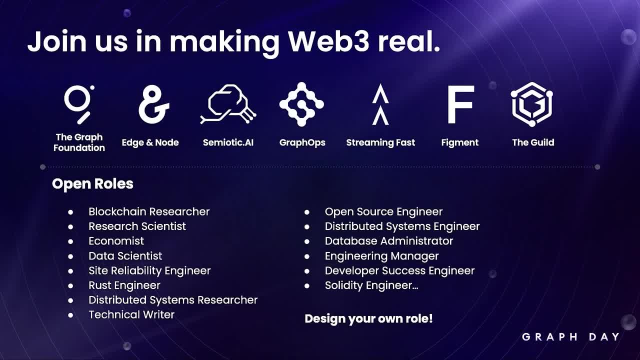 really just scratched the surface. So if you're interested in diving deeper on any of these topics, you know we've already scratched the surface, And I want to give a shout out to all the new core developers that have joined our ecosystem since the last Graph Day. We really wouldn't be here. 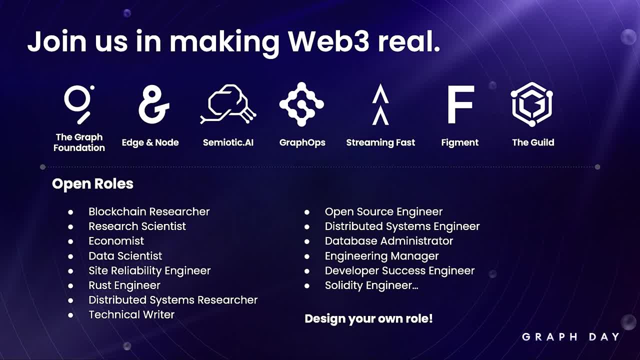 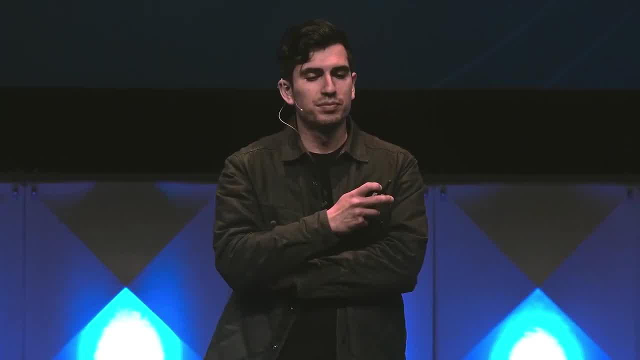 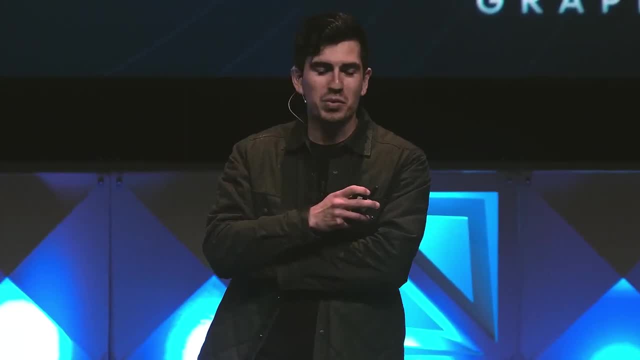 without them, and I know that the future of the graph is bright because we have all of them on board And if you're interested in rolling up your sleeves and getting to work and becoming a part of this journey, we've got a ton of open roles to fill, so please get in touch, Come find one of us. 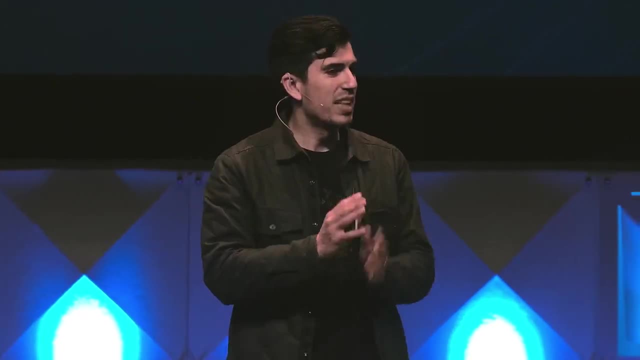 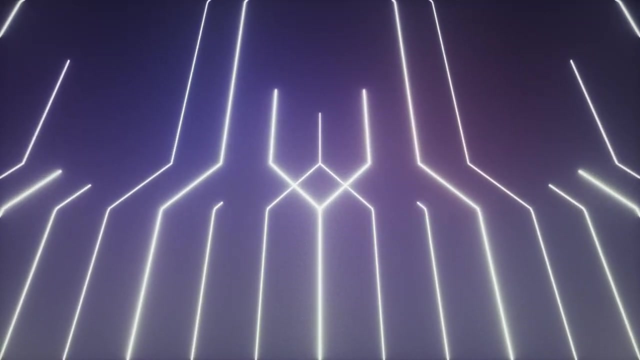 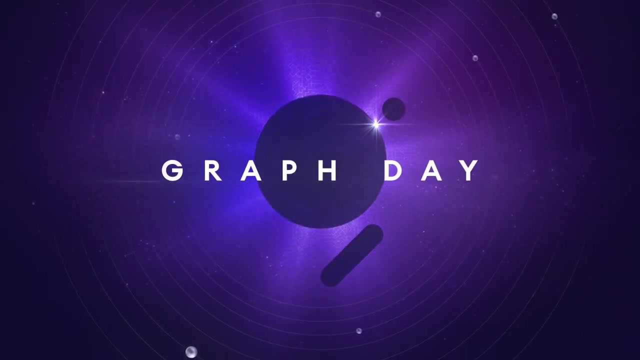 during GraphHack or at the party. Thank you guys very much.